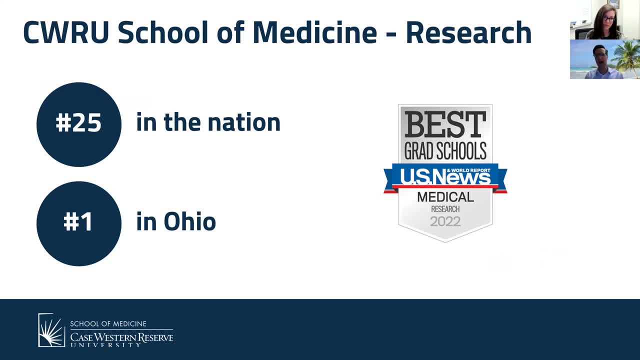 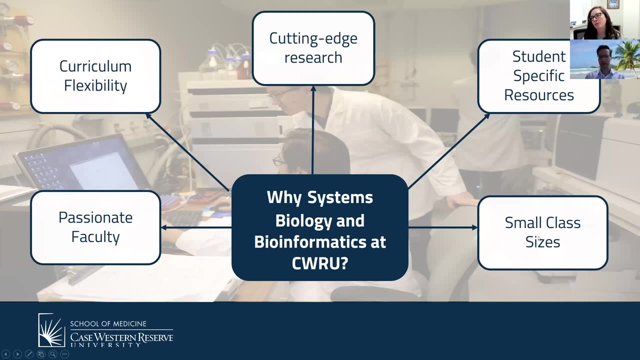 funding at at the medical, the medical school side, In terms of research we are. you can go ahead and go to the next slide. Okay, so so our, our program really is has been designed around sort of a flexible, a flexible framework that really enables students to, to, to really assimilate a lot, a sort of a very difficult 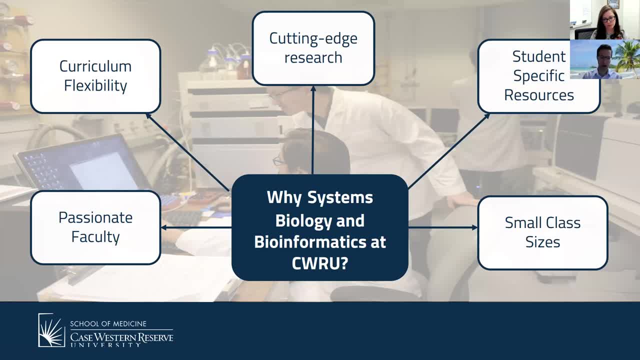 subject matter in a short period of time. so we have a lot of flexibility in what courses you take in terms of we don't. we don't have a set curriculum for every student, so some students come in with a significant experience in, say, computer science or statistics, and then they 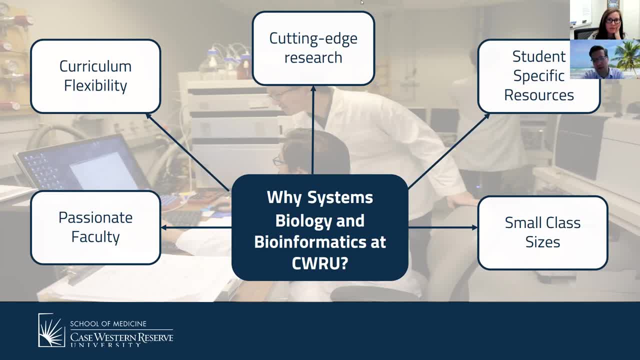 would not take as many statistics or computer science courses and like same with the sort of the biology side. so some students have a, have a, already, have an undergraduate degree in, in, in biological sciences, and so again, we're not going to make them take a bunch of classes. 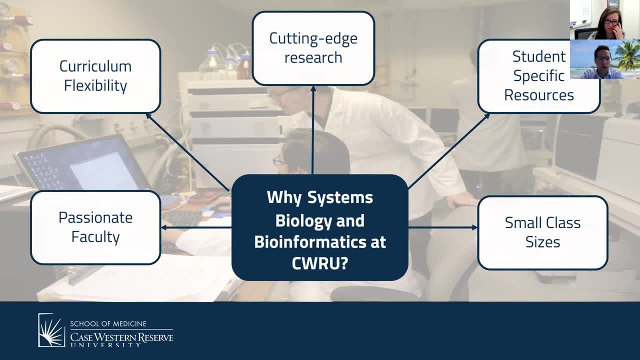 about stuff they've already done. So we have in our, in our program. we have it's right around 45 faculty who are trainers for our MS and PhD students, so they provide sort of the support of for your research um portfolio that you'll develop as as a student um, and you know we really are. 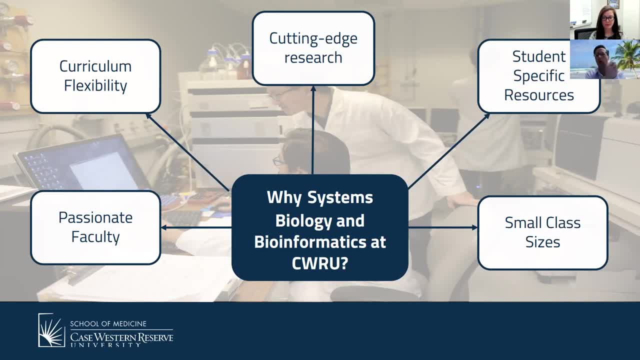 producing some really beautiful research. we've we go everywhere from um. we have people that are working on developing um Alexa apps for for dealing with home medical questions, all the way down to structural biology, to cancer, um informatics. so all of these sort of just you know. 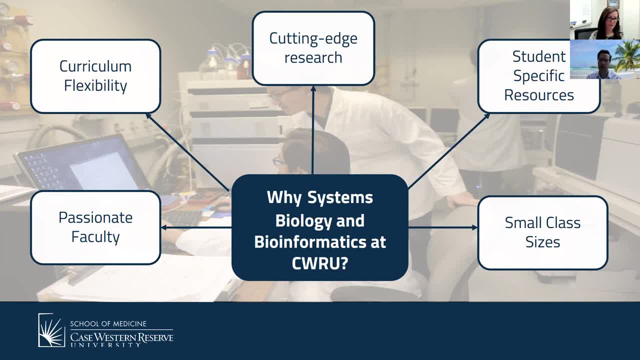 completely spanning the whole sort of constellation of, um, of sort of biological sciences, um, there are big data, questions that can be answered by analyzing them in sort of a systematic method. One more thing I'll mention before we go to the next slide is that, you know, we, we don't have an 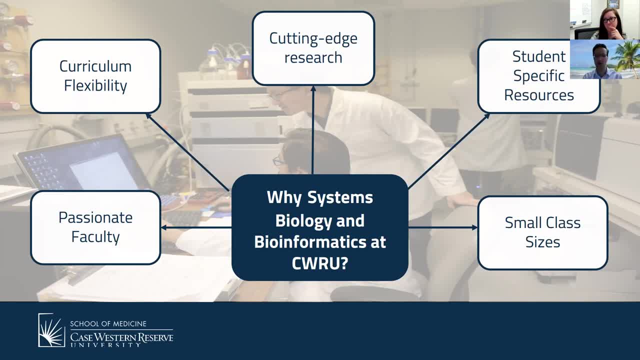 enormous program. we don't take a hundred students per year. we take in between five and ten. this allows me to actually know who you are and and the rest of the training faculty to know who you are and to really get to know who you are and to really get to know who you are and to really get to know. 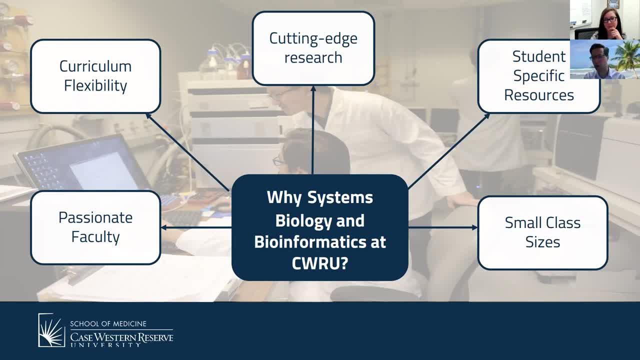 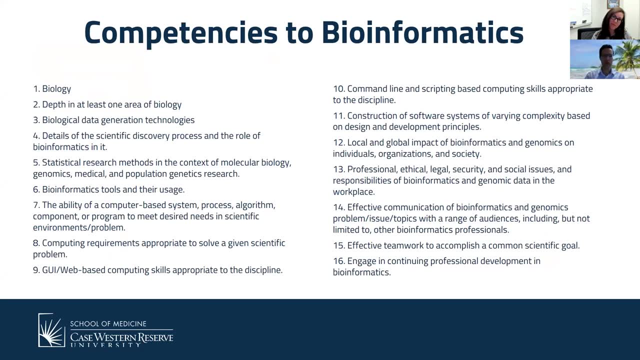 you and really fit you into a lab where you belong and where you can success, succeed, um, so, in terms of what do you need, or what do we teach you? um, and that you know so, so these are our competencies, so what? what? that's another way of saying: what are the skills that I'm going to? 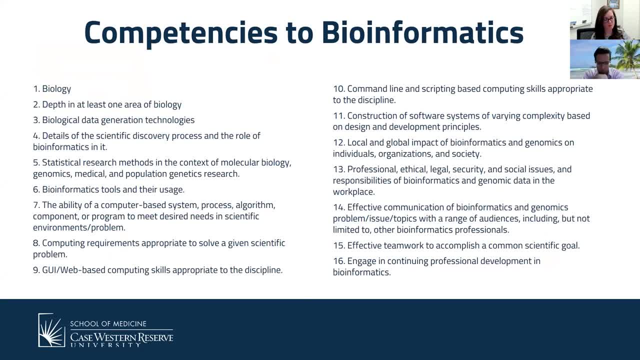 learn as a um, as a, as a um as a student, um as a student, um as a um as a student. And so, first and foremost, biology, right. so we need to know, we need to know about how things work in the sort of in the organism or in the organism, and then we push you down into one area of 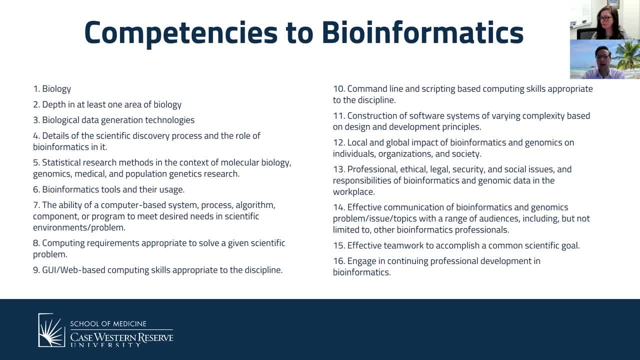 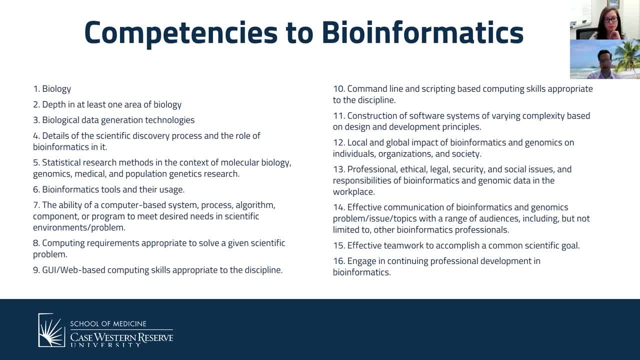 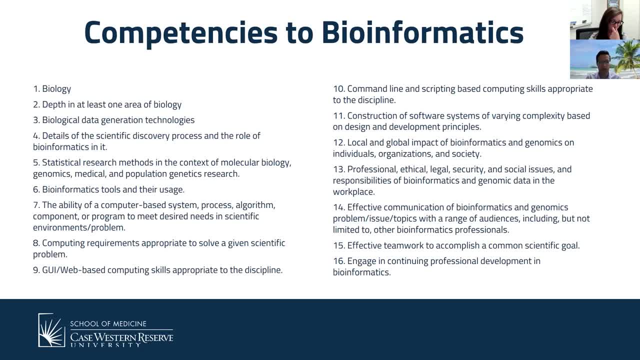 and then, of course, then there's the tools, and then, of course, then there's the tools that we need in order to do that, so that we need, in order to do that, so that we need, in order to do that, so, statistical research methods. statistical research methods. 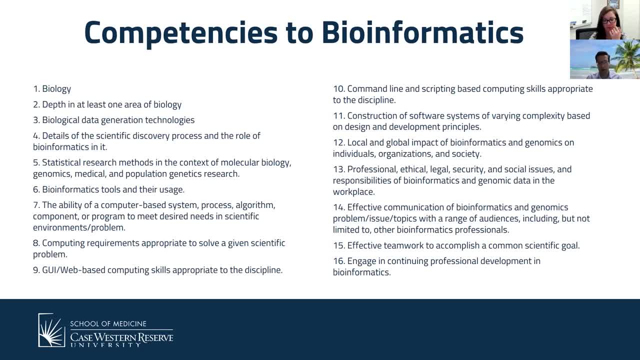 statistical research methods um bioinformatics tools. the utilization um bioinformatics tools. the utilization um bioinformatics tools, the utilization of a computer to really do this, of a computer to really do this, of a computer to really do this, and then sort of, and then you know, and then sort of, and then you know, run that and you know, get the stuff. 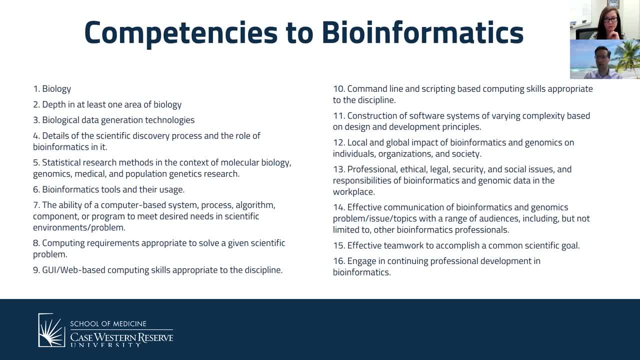 run that and you know, get the stuff. run that and you know, get the stuff out of that. it's necessary to to really out of that. it's necessary to to really out of that, it's necessary to to really gain the high level understanding of the gain, the high level understanding of the. 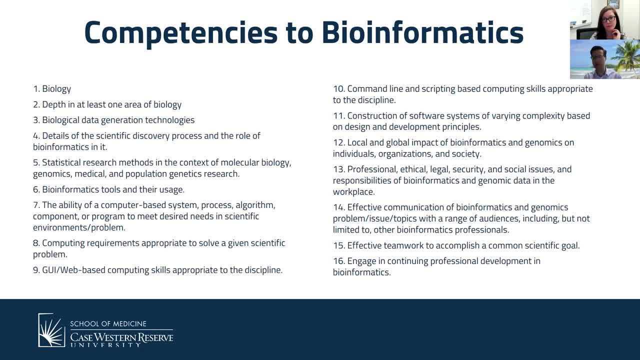 gain the high level understanding of the data that you would have developed in data that you would have developed in, data that you would have developed in competency competency number three, or competency competency number three, or competency competency number three, or four, four, four, um. and then you know, there's, there's a 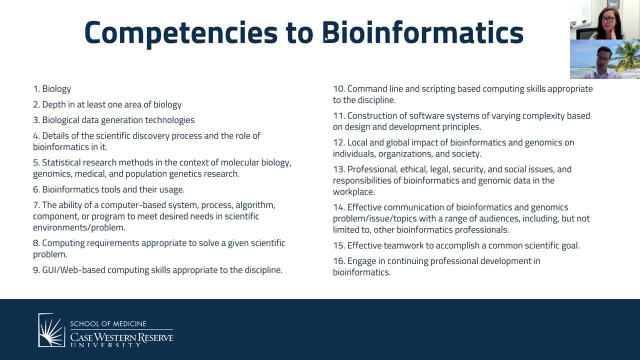 um, and then you know there's. there's a um, and then you know there's there's a whole, whole, whole. there's a whole sort of progression here. there's a whole sort of progression here. there's a whole sort of progression here and so and so. 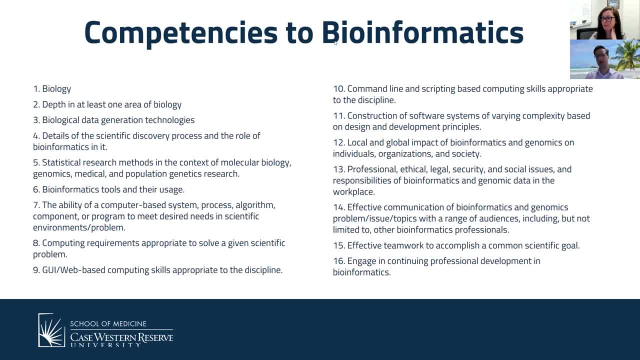 and so you'll, you'll learn about, you know you'll, you'll learn about, you know you'll, you'll learn about, you know making pipelines to go from big data to making pipelines to go from big data, to making pipelines to go from big data to an actionable conclusion from big data. 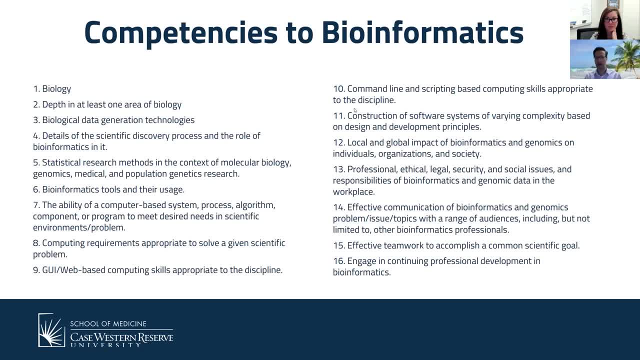 an actionable conclusion from big data, an actionable conclusion from big data. and then, of course, we're going to we're, and then, of course, we're going to we're, and then, of course, we're going to, we're going to make sure that you understand, going to make sure that you understand. 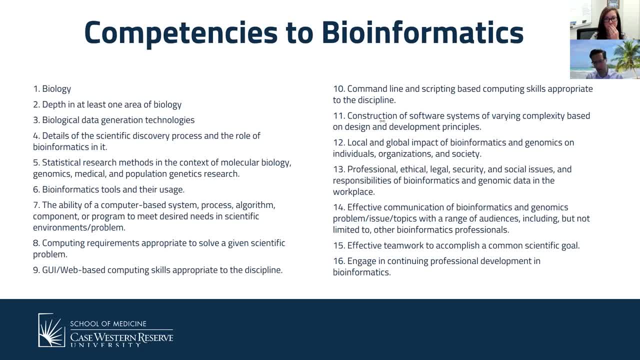 going to make sure that you understand the professional ethical legal, social. the professional ethical legal social. the professional ethical legal, social issues. that issues. that issues that revolve around big data and big data revolve around big data and big data revolve around big data and big data analysis. 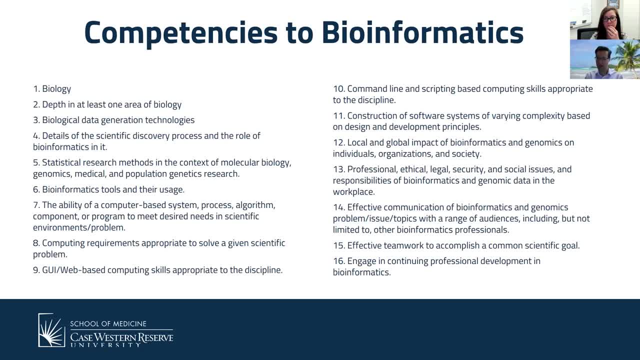 analysis, analysis, because there are some very interesting, because there are some very interesting, because there are some very interesting sort of privacy issues that exist, sort of privacy issues that exist, sort of privacy issues that exist around in that space, around in that space, around in that space. um, and then we'll teach you how to write. 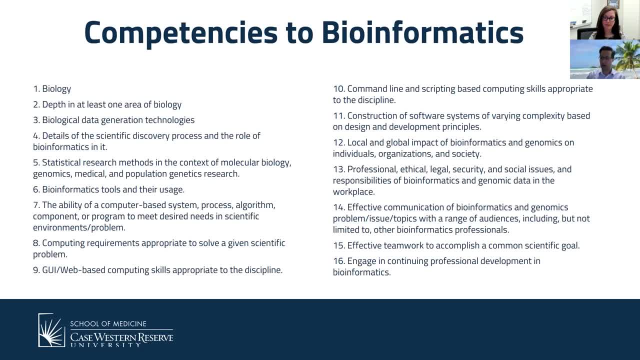 um, and then we'll teach you how to write um, and then we'll teach you how to write this stuff up, this stuff up, this stuff up in in a paper, and then how to really in in a paper, and then how to really in in a paper and then how to really utilize a team. because one thing i 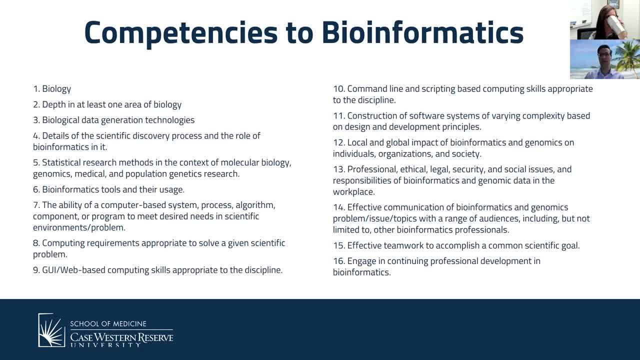 utilize a team, because one thing i utilize a team, because one thing i really stress is that you know these. really stress is that you know these. really stress is that you know these, these kinds of uh data analysis, these kinds of uh data analysis, these kinds of uh data analysis, um degrees and and sort of ways of 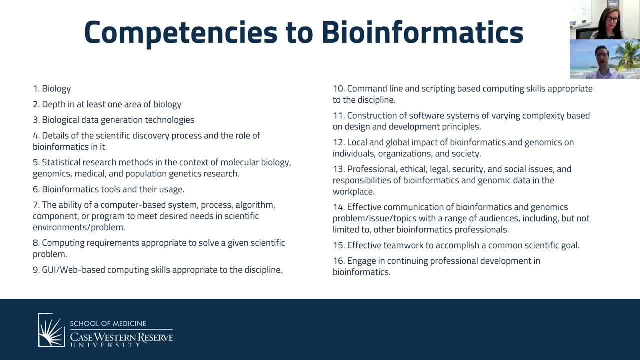 um degrees and and sort of ways of um degrees and and sort of ways of doing things are really not ever done. doing things are really not ever done. doing things are really not ever done in a vacuum. and it's not. you're not going in a vacuum, and it's not. you're not going. 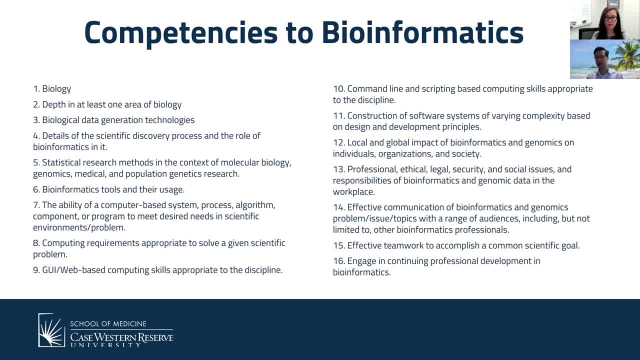 in a vacuum and it's not. you're not going to to to be the single person. who is going to be the single person. who is going to be the single person who is going to generate the data, generate the data. generate the data, analyze the data. take that analysis from. 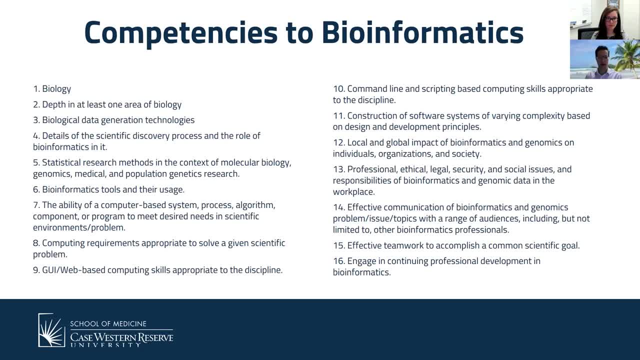 analyze the data. take that analysis from. analyze the data. take that analysis from the data. the data, the data. develop a hypothesis test. the test, the develop a hypothesis test. the test, the develop a hypothesis test. the test, the hypothesis and come out with something at hypothesis. and come out with something at. 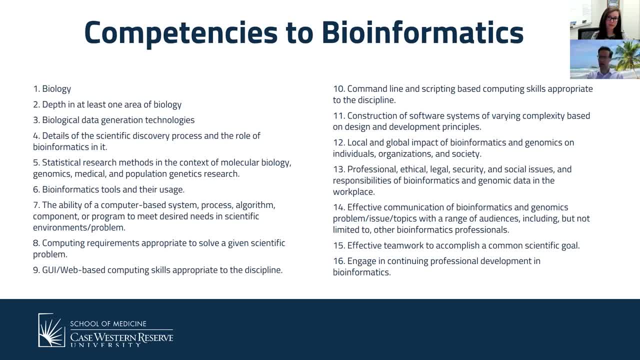 hypothesis and come out with something at the end. that's just way too much work. the end, that's just way too much work. the end, that's just way too much work for one person to do, or even a lot of for one person to do, or even a lot of. 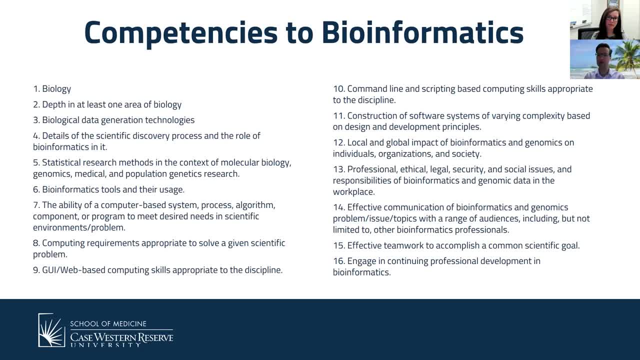 for one person to do, or even a lot of times for even one laptop times for even one laptop times for even one laptop. so you're going to be able to understand, so you're going to be able to understand, so you're going to be able to understand the. 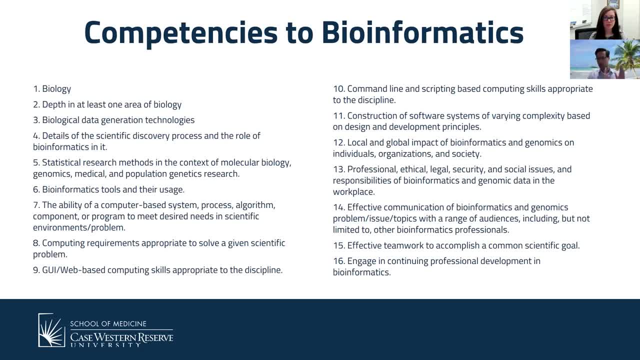 the the sort of where you fit in that, in that sort of where you fit in that, in that sort of where you fit in that, in that role, and some people are going to fit role and some people are going to fit role and some people are going to fit more on the front end and some people more on the front end and some people more on the front end, and some people are going to fit more on the back end, are going to fit more on the back end, are going to fit more on the back end, but we're going to give you the tools to 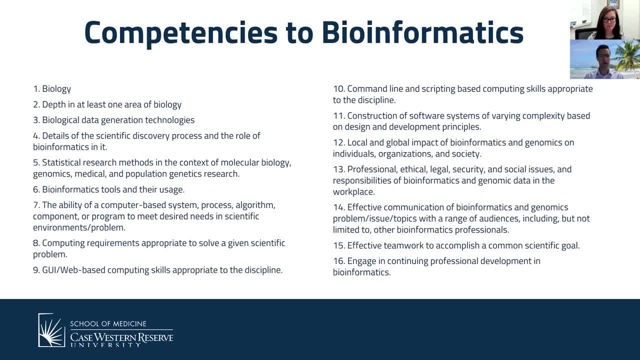 but we're going to give you the tools to. but we're going to give you the tools to fit in where you need to fit. okay. so fit in where you need to fit. okay, so fit in where you need to fit. okay. so let's go ahead and go to the next slide. 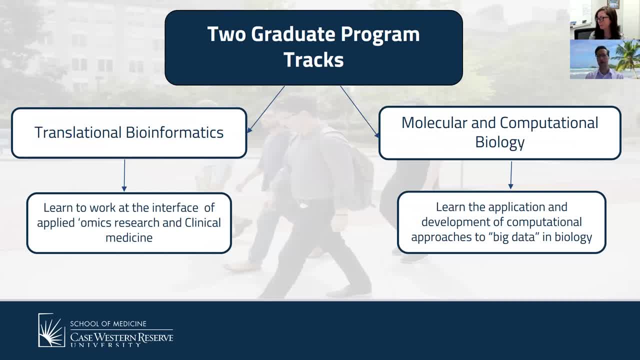 let's go ahead and go to the next slide. let's go ahead and go to the next slide. okay, so we offer two tracks in in the. okay, so we offer two tracks in in the. okay, so we offer two tracks in in the sybb program um. 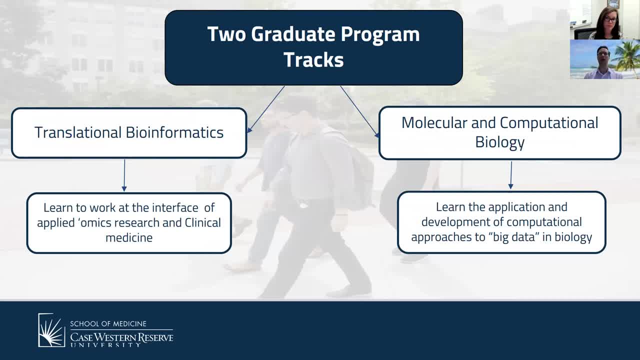 sybb program, um, sybb program, um, they, they really are quite similar, they, they, they really are quite similar, they, they, they really are quite similar. they really just kind of define, really just kind of define, really just kind of define the research topics over which you are. 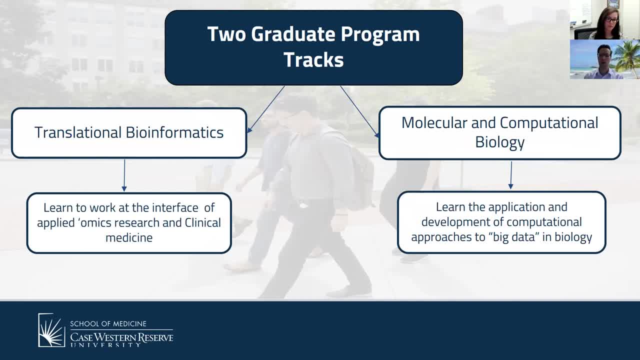 the research topics over which you are, the research topics over which you are going to um, going to um, going to um, what you're really interested in, um, what you're really interested in, um, what you're really interested in, um. there's no real binding decision. so if 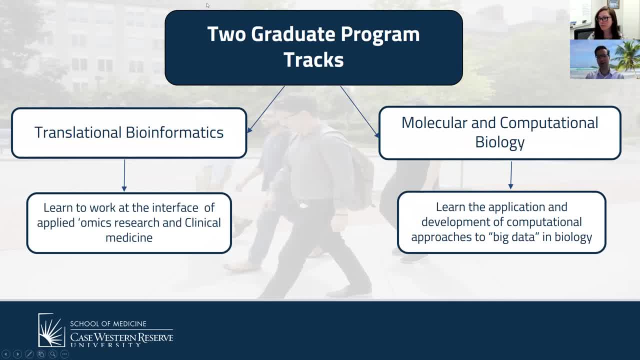 there's no real binding decision. so if there's no real binding decision, so if you are doing the translational for a, you are doing the translational for a, you are doing the translational for a while and you decide that molecular and while and you decide that molecular and. 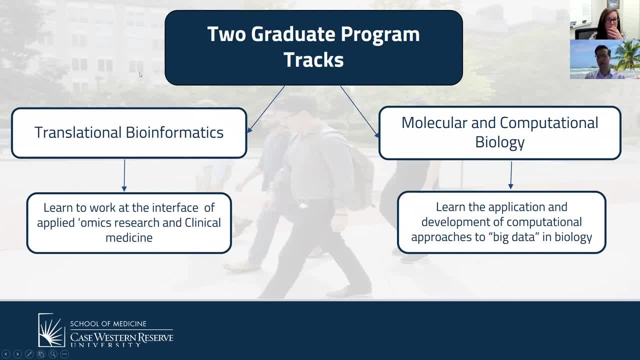 while, and you decide that molecular and computational biology tract is computational biology tract is computational biology tract is more, more to your liking the class, more, more to your liking the class, more, more to your liking the class, the classes that you take aren't much. the classes that you take aren't much. 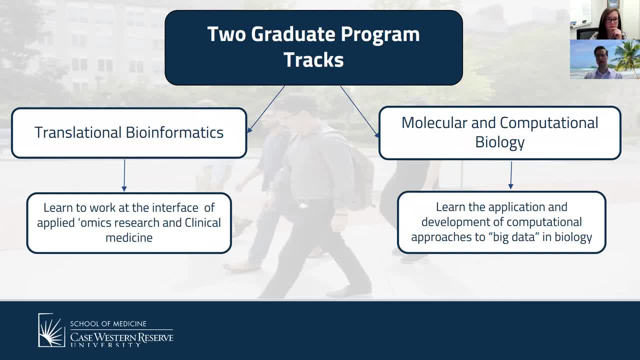 the classes that you take aren't much different. so really there is a really different. so really there is a really different. so really there is a really just a direct switch back and forth. so just a direct switch back and forth. so just a direct switch back and forth. so it really just reflects what 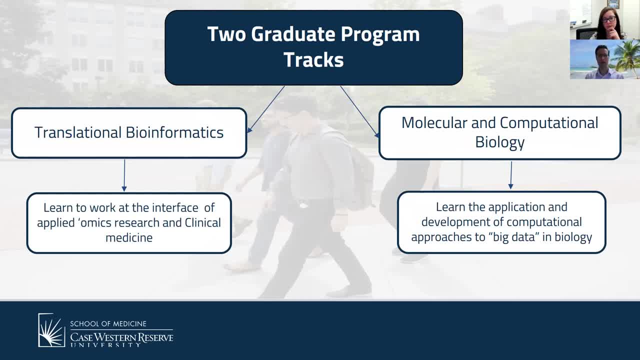 it really just reflects what. it really just reflects what, um what your personal interests are and um what your personal interests are and um what your personal interests are. and so the translational bioinformatics, so the translational bioinformatics, so the translational bioinformatics we're really looking at sort of how can 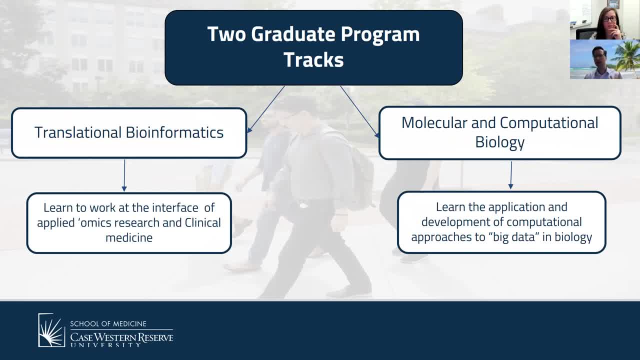 we're really looking at sort of how can we're really looking at sort of how can we use this in the clinical in the? we use this in the clinical in the. we use this in the clinical in the clinical space and then the molecular clinical space and then the molecular. 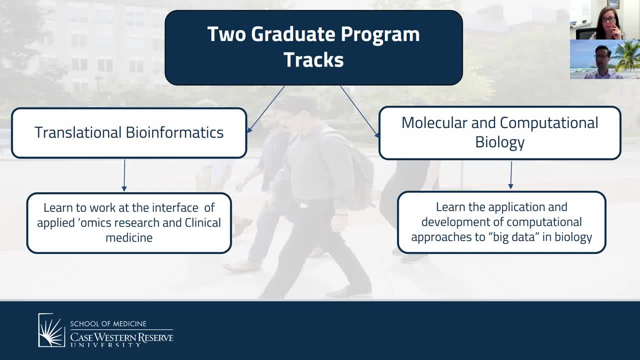 clinical space. and then the molecular computational biology. it's, it's very computational biology. it's, it's very computational biology. it's, it's very similar, it's just it's taking big data. similar, it's just it's taking big data. similar, it's just it's taking big data in that's developed in more biological. 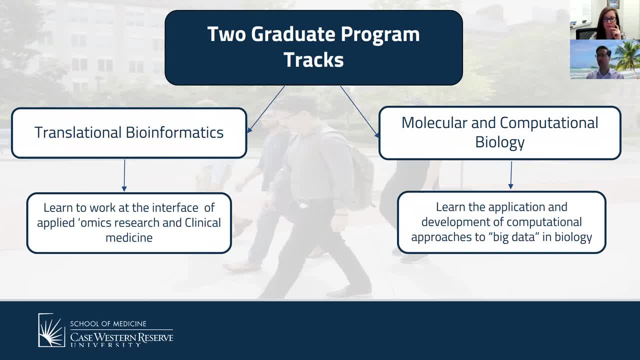 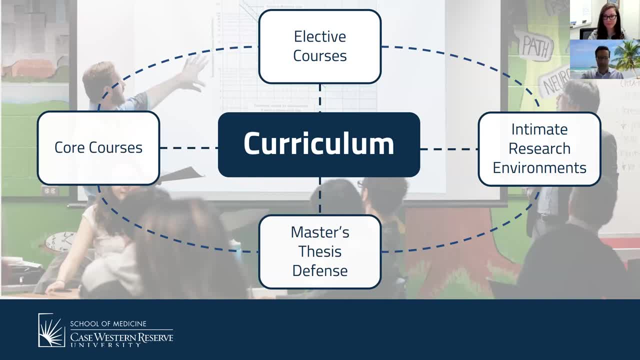 in that's developed in more biological, in that's developed in more biological science as opposed to medical science, science as opposed to medical science, science as opposed to medical science. and developing actionable things from and developing actionable things from and developing actionable things from that. okay, next slide. 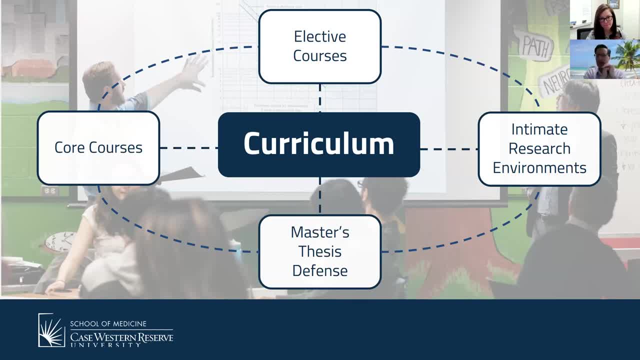 okay so in terms of a curriculum. okay so in terms of a curriculum. okay so in terms of a curriculum, so we do this, so we do this a little, so we do this, so we do this a little, so we do this, so we do this a little bit differently. i i mentioned this. 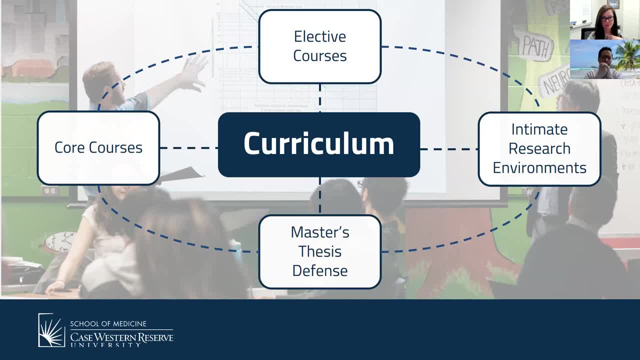 bit differently. i i mentioned this bit differently. i i mentioned this before. we have a very before. we have a very before. we have a very flexible, flexible, flexible curriculum. so we have two core classes curriculum. so we have two core classes curriculum. so we have two core classes that are absolutely required of all. 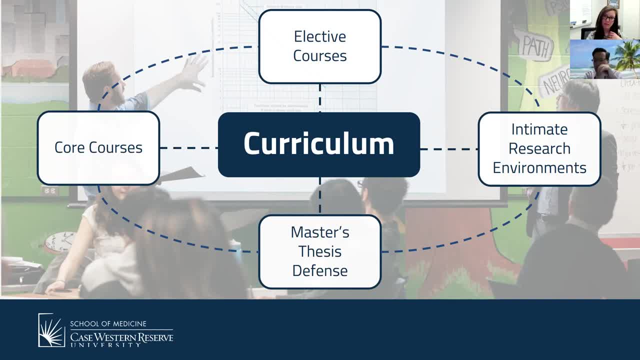 that are absolutely required, of all, that are absolutely required of all students, students, students, um. and then we will push you into um, and then we will push you into um, and then we will push you into classes and we'll we'll do this in classes and we'll we'll do this in. 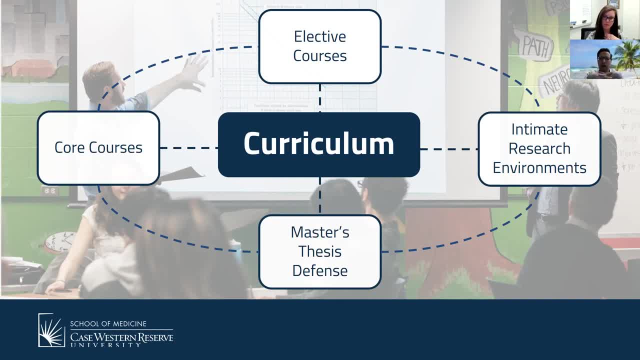 classes and we'll- we'll do this in consultation with you, consultation with you, consultation with you um to figure out where um to figure out where um, to figure out where you know what classes are best for you. you know what classes are best for you, you know what classes are best for you in order to 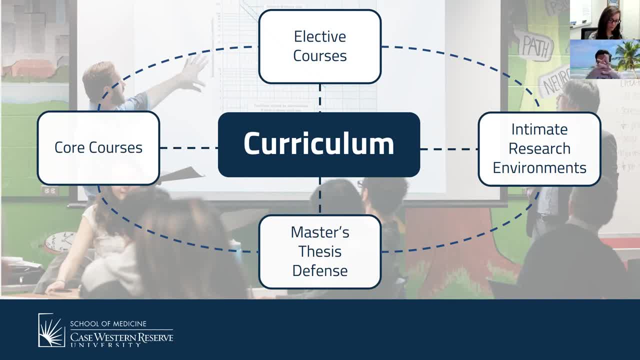 in order to, in order to um learn. you know everything that you um learn. you know everything that you um learn. you know everything that you need to do to to successfully. uh, you need to do to successfully. uh, you need to do to successfully. uh, you know. do your thesis research. now i will. 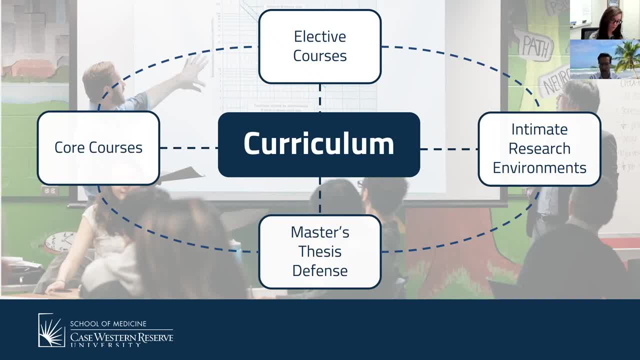 know, do your thesis research now. i will know, do your thesis research now. i will say that there are two tracks that are. say that there are two tracks that are. say that there are two tracks that are that exist within the program. there's a that exist within the program. there's a. 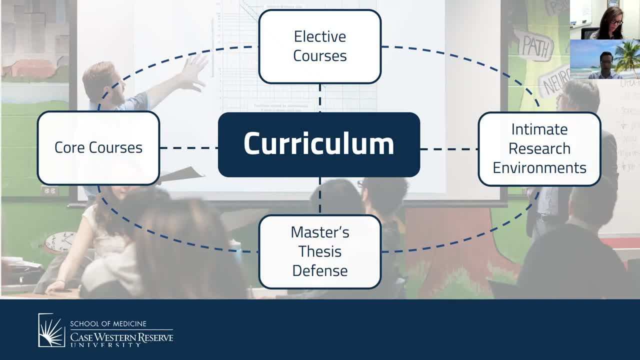 that exist within the program. there's a, so we do. we have well sorry, two tracks, so we do. we have well, sorry, two tracks, so we do. we have well sorry, two tracks, but we, but we, but we, sorry, that was. that's a bad, bad way of. sorry that was. that's a bad, bad way of sorry that was. that's a bad, bad way of saying that. so we have the two tracks saying that. so we have the two tracks saying that. so we have the two tracks that i talked about the last, that i talked about the last. 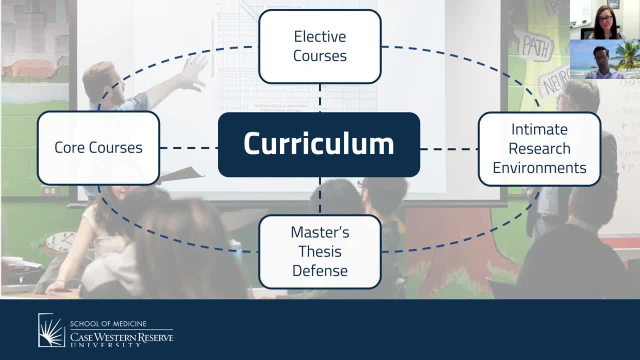 that i talked about the last unless, but there's also a way to do a unless, but there's also a way to do a unless, but there's also a way to do a completely course-based thesis, completely course-based thesis, completely course-based thesis, as well as a master's thesis, where 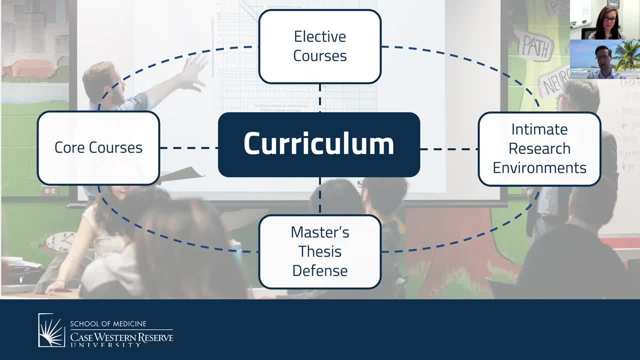 as well as a master's thesis, where, as well as a master's thesis, where you've done, you've done, you've done um a significant effort towards um, a significant effort towards um, a significant effort towards research, um, and we really, we really research um and we really, we really. 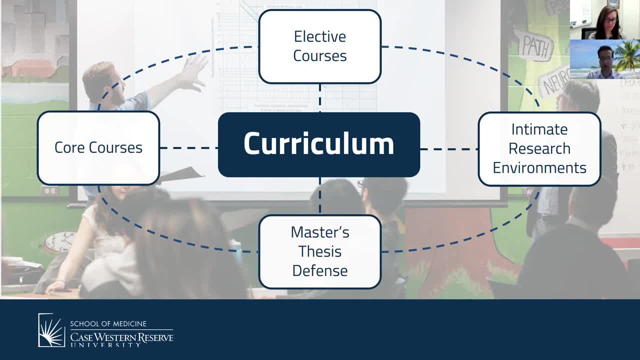 research, um, and we really, we really really um try to encourage you guys to really um try to encourage you guys to really um try to encourage you guys to only do the master's thesis, only do the master's thesis, only do the master's thesis work, because we think that that's the 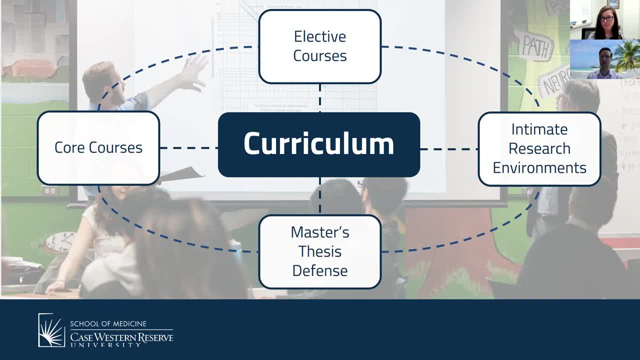 work, because we think that that's the work, because we think that that's the best way for you to really learn these. best way for you to really learn these, best way for you to really learn these skills is to put them into practice. skills is to put them into practice. 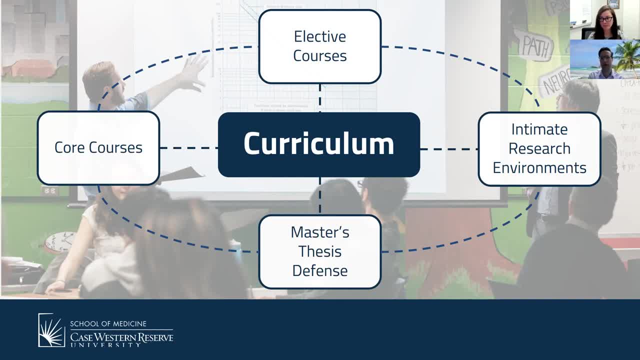 skills is to put them into practice. um, and then the nice thing at the end: um, and then the nice thing at the end: um, and then the nice thing at the end is: you have a big, is you have a big, is you have a big? you have a big book or a document that 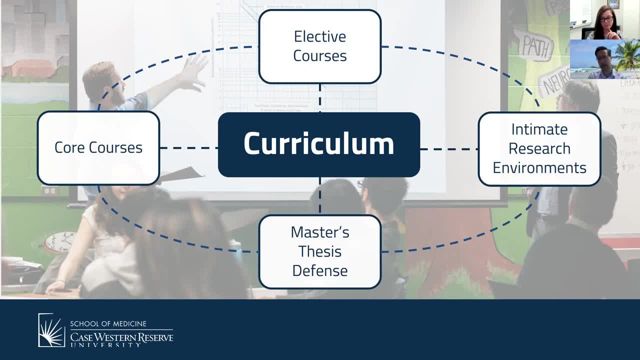 you have a big book or a document, that you have a big book or a document that really, really, really documents how you utilized informatics to documents, how you utilized informatics to documents, how you utilized informatics to do something with a big data set. do something with a big data set. 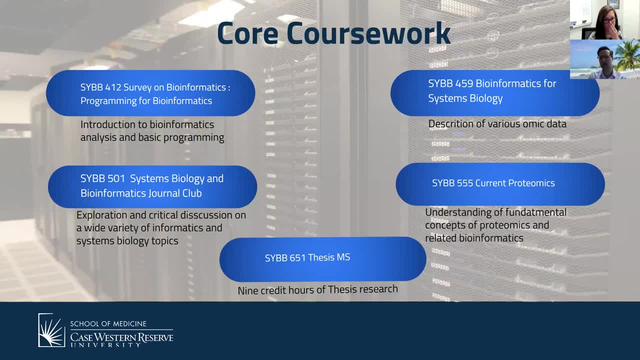 do something with a big data set. if you do the coursework based thing, if you do the coursework based thing, if you do the coursework based thing, it's a little bit less. it's a little bit less. it's a little bit less. um, there's a little bit less for you. 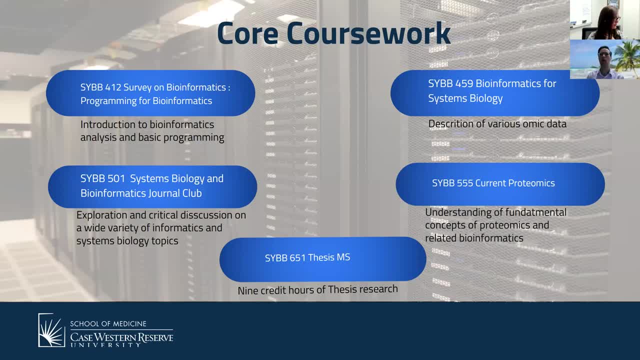 um, there's a little bit less for you. um, there's a little bit less for you to show when you're going to a to show, when you're going to a to show when you're going to a prospective employer, prospective employer, prospective employer or or to a phd program for. 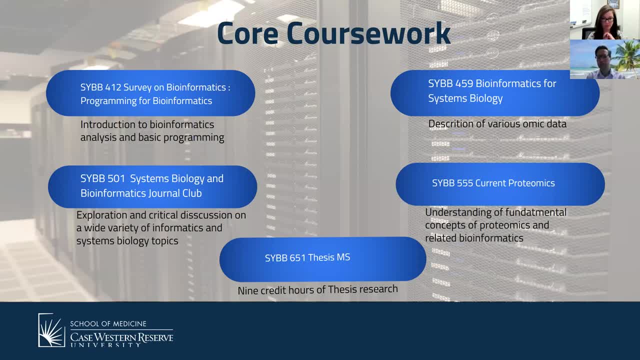 or or to a phd program for, or or to a phd program for um application um application um application, um. so, as i said, there's only a um. so, as i said, there's only a um. so, as i said, there's only a. there's only a small amount of. 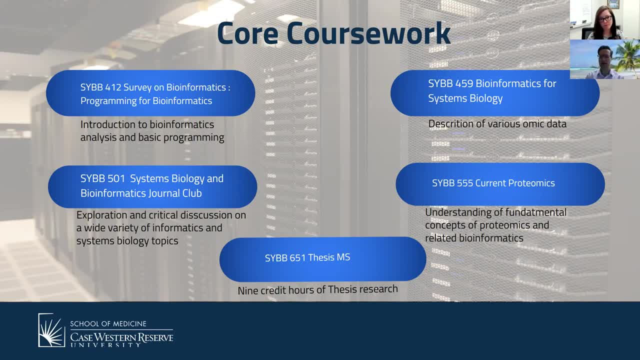 there's only a small amount of, there's only a small amount of required courses, so we have a. i said required courses, so we have a. i said required courses, so we have a. i said two, i actually meant three. two, i actually meant three. two, i actually meant three. um, so we have this. sybb 412 survey. 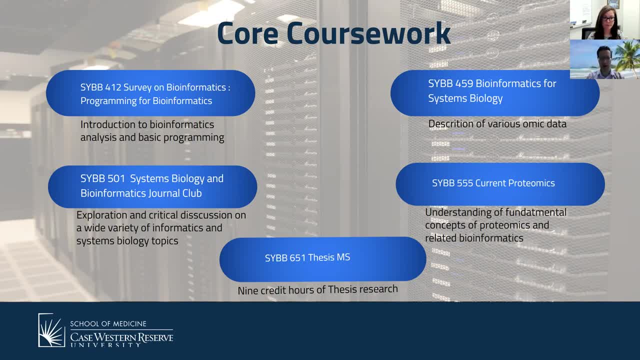 um, so we have this sybb 412 survey. um, so we have this sybb 412 survey course, which is really just a very course, which is really just a very course, which is really just a very, a very perfunctory introduction to a very perfunctory introduction to. 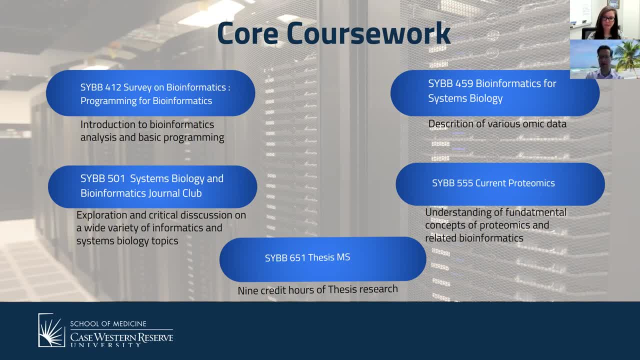 a very perfunctory introduction to a little bit of the programming behind a little bit of the programming behind a little bit of the programming behind bioinformatics, bioinformatics, bioinformatics. um then we have this sybb 459 course. um then we have this sybb 459 course. 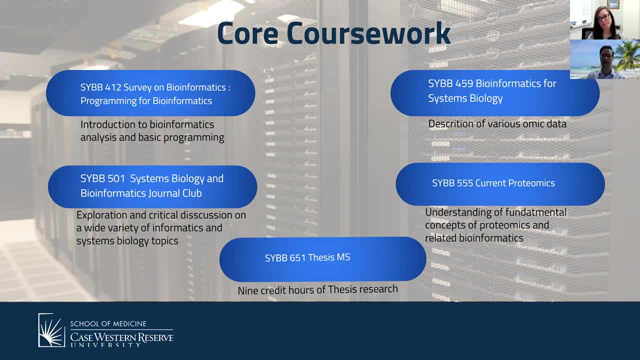 um, then we have this sybb 459 course which really helps you, which really helps you, which really helps you kind of understand, not the initial kind of understand, not the initial kind of understand, not the initial analysis of the data, but how do you take analysis of the data, but how do you take? 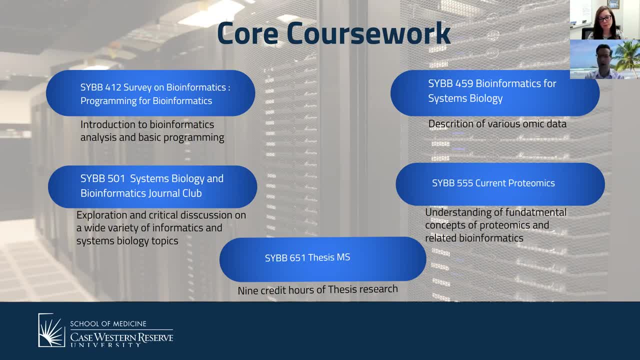 analysis of the data. but how do you take that analyzed data and develop a model that analyzed data? and develop a model that analyzed data and develop a model from it, from it, from it? and then we want to have you learn a, and then we want to have you learn a. 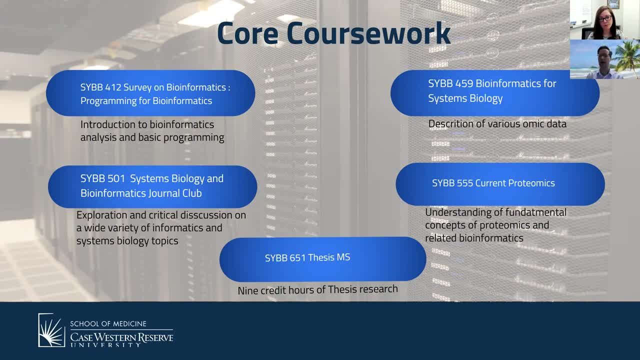 and then we want to have you learn a sort of from beginning to end, idea of sort of from beginning to end, idea of sort of from beginning to end, idea of how do i take, how do i take, how do i take, how do i go from a tissue. 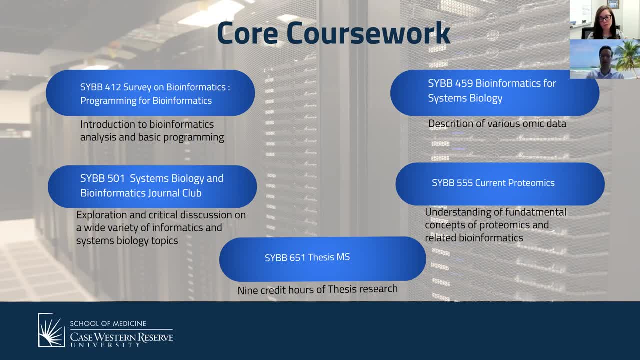 how do i go from a tissue, how do i go from a tissue to a, to a, to a testable hypothesis? and so this sybb555 testable hypothesis. and so this sybb555 testable hypothesis. and so this sybb555 class is the, class is the. 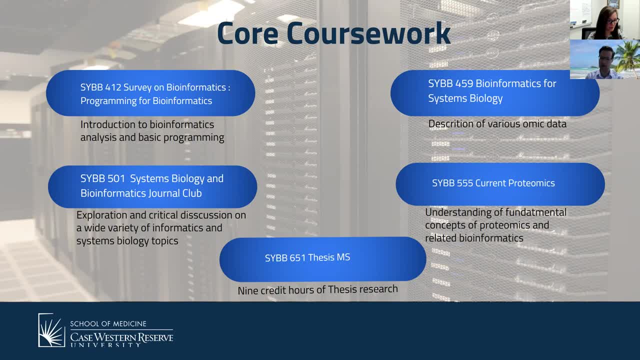 class is. the is one of a couple that we offer. that is one of a couple that we offer. that is one of a couple that we offer that allows you to really see, allows you to really see, allows you to really see from the beginning to the end. so you see, 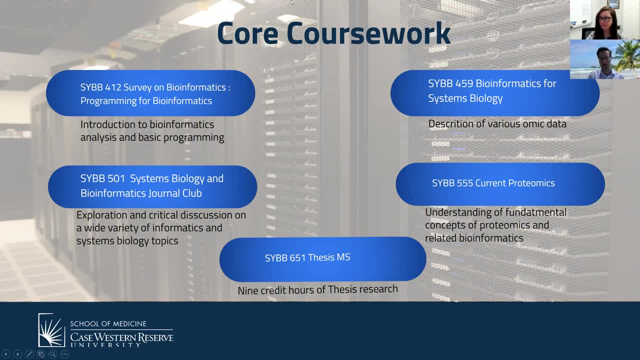 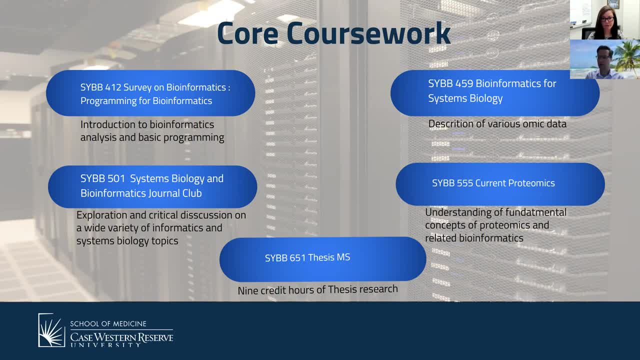 take that data, take that data and analysis. utilize that all all the and analysis. utilize that all all the and analysis. utilize that all all the way up through to get sort of a way up through to get sort of a way up through to get sort of a actionable biological hypothesis. so 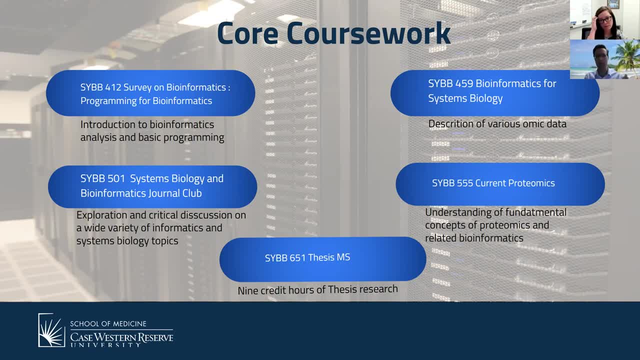 actionable biological hypothesis. so actionable biological hypothesis, so really all the way from from literally really all the way from from literally, really all the way from from literally, from from from cells to a hypothesis, from what? from the cells to a hypothesis, from what? from the cells to a hypothesis, from what? from the beginning to the end. 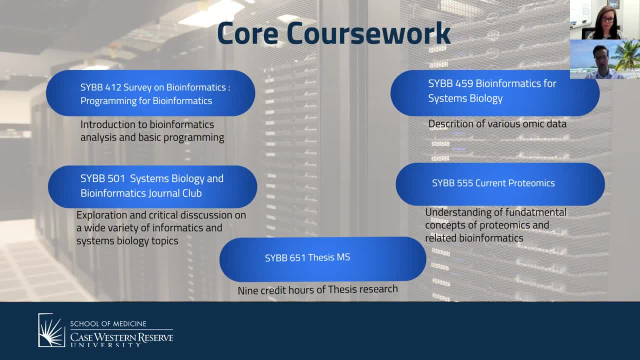 beginning to the end. beginning to the end: um, and then the thesis master, the the um, and then the thesis master, the, the um, and then the thesis master, the, the thesis research. if you do that, you're thesis research. if you do that, you're thesis research. if you do that, you're going to do that in year two of the of. 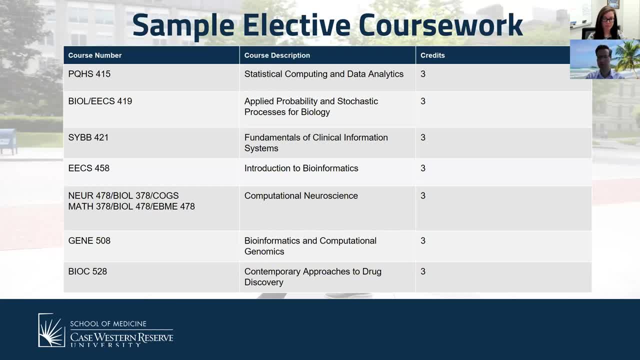 going to do that in year two of the of going to do that in year two of the of the master's degree, okay, so this is just a sample. this is okay. so this is just a sample. this is okay. so this is just a sample. this is not. this is not what everybody takes at. 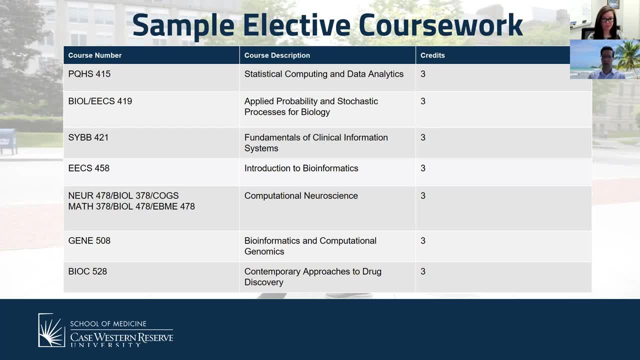 not, this is not what everybody takes at. not, this is not what everybody takes at all, but this is something. these are some all, but this is something. these are some all, but this is something. these are some of the electives that that are offered, of the electives that that are offered. 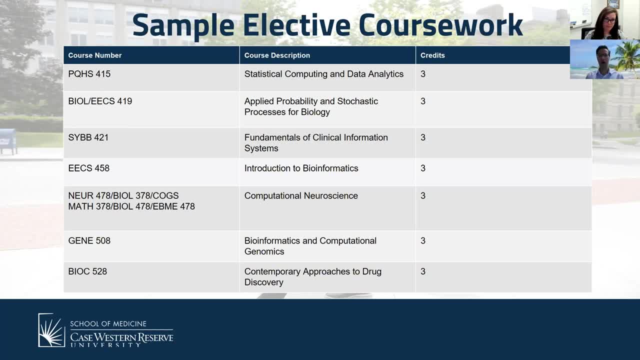 of the electives that that are offered. so um, so um, so um. there's there's statistical um. there's there's statistical um. there's there's statistical um. there's some statistical uh analysis. there's some statistical uh analysis. there's some statistical uh analysis uh classes that are taught pqhs. 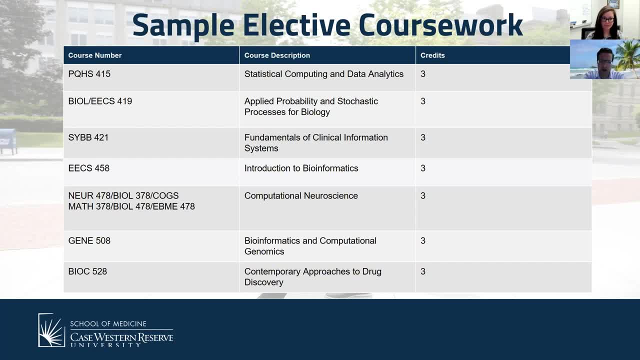 uh, classes that are taught pqhs. uh, classes that are taught pqhs. 415 is one. i also have another one that i 415 is one. i also have another one that i 415 is one. i also have another one that i send most of the master students to. 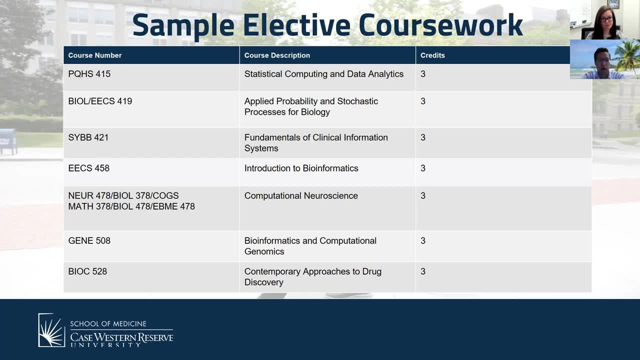 send most of the master students to send most of the master students to which is pqs- pqhs 451. which is pqs pqhs 451. which is pqs pqhs 451 and 45, oh sorry, 431 and 432 and that. and 45, oh sorry, 431 and 432 and that. 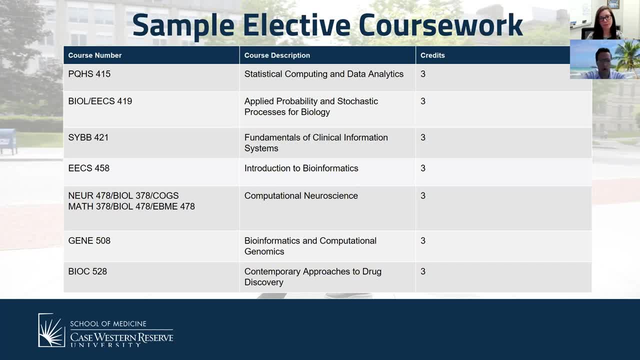 and 45, oh sorry, 431 and 432, and that really is sort of a big, really is sort of a big, really is sort of a big a beginning and advanced our a beginning and advanced our a beginning and advanced our programming course, programming course, programming course. then we have a bunch of things that 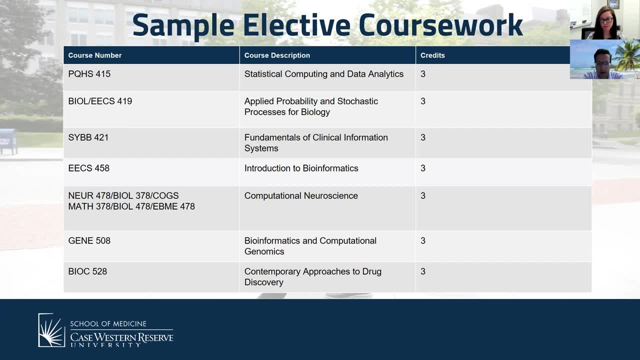 then we have a bunch of things that then we have a bunch of things that really are a little bit more, really are a little bit more, really are a little bit more niche and fit directly into people's niche and fit directly into people's niche and fit directly into people's interests. so like this: 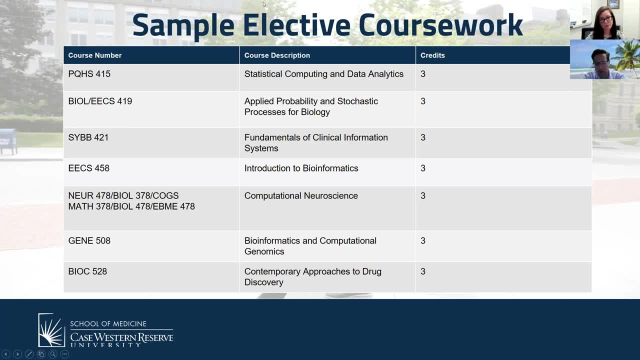 interests, so like this interests, so like this applied probability, or fundamentals of applied probability, or fundamentals of applied probability, or fundamentals of clinical information systems, which is a clinical information systems, which is a clinical information systems, which is a very popular course, really teaches you. very popular course really teaches you. 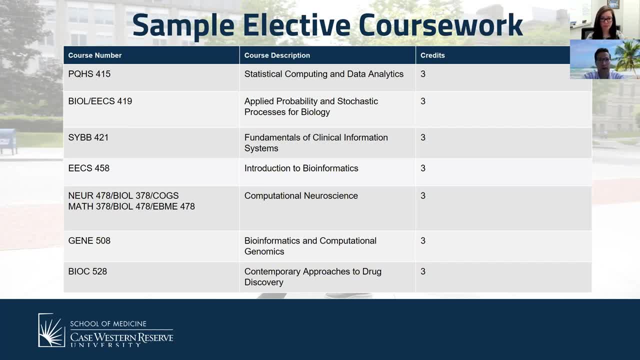 very popular course really teaches you how to develop a, how to develop a, how to develop a informatic based, informatic based, informatic based product for for um product, for for um product for for um. well, kind of for sale or for sort of in. well, kind of for sale or for sort of in. 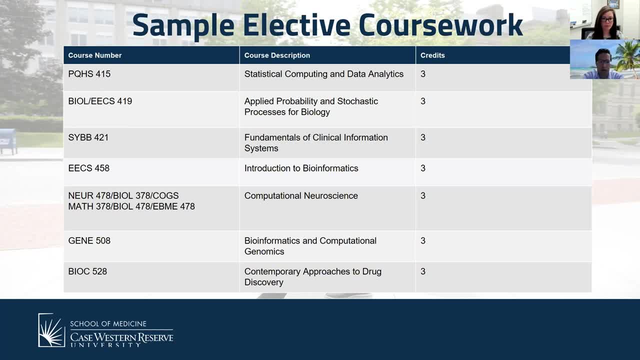 well, kind of for sale or for sort of in the industrial or non-academic space, the industrial or non-academic space, the industrial or non-academic space, um, um, um, and then you know there's some things, and then you know there's some things, and then you know there's some things that have to do more with the biology. 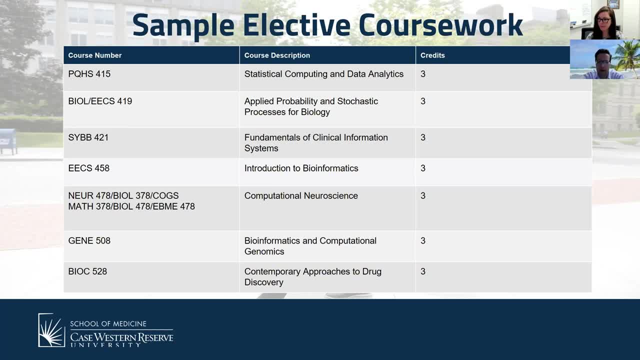 that have to do more with the biology, that have to do more with the biology. realm or realm or realm or um or even drug discovery can be you. you, um or even drug discovery can be you. you, um or even drug discovery can be you. you can utilize a systems approach to kind. 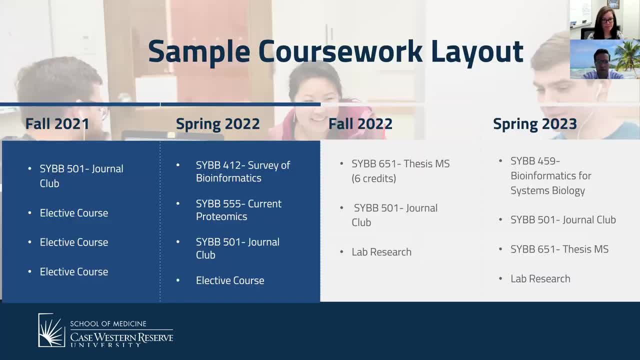 can utilize a systems approach to kind can utilize a systems approach to kind of figure that out. okay, next slide, so so. so, how do i get this done in two years? well, how do i get this done in two years? well, how do i get this done in two years? well, this is kind of how you're going to do. 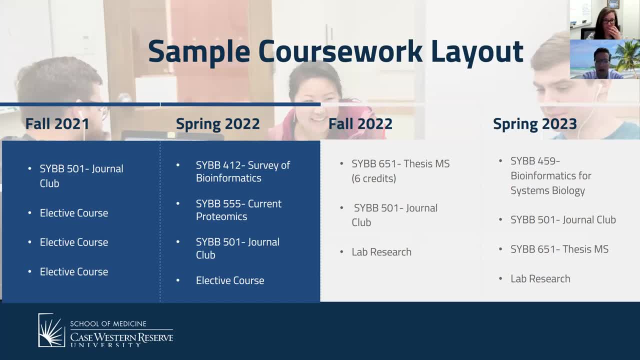 this is kind of how you're going to do. this is kind of how you're going to do this. so you'll take your journal club this. so you'll take your journal club this. so you'll take your journal club, you'll take it a lot you'll take actually. 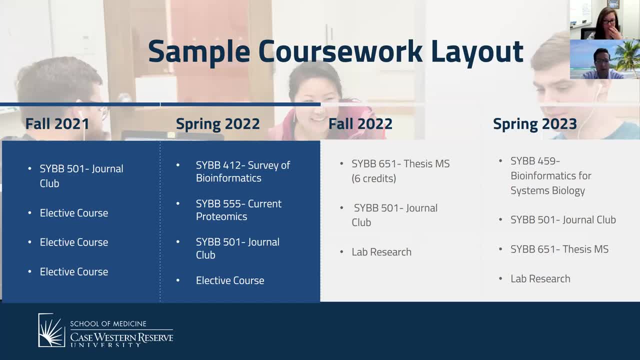 you'll take it a lot. you'll take, actually you'll take it a lot. you'll take actually three electives that first semester, and so three electives that first semester, and so three electives that first semester, and so um, and then that second semester, we're. 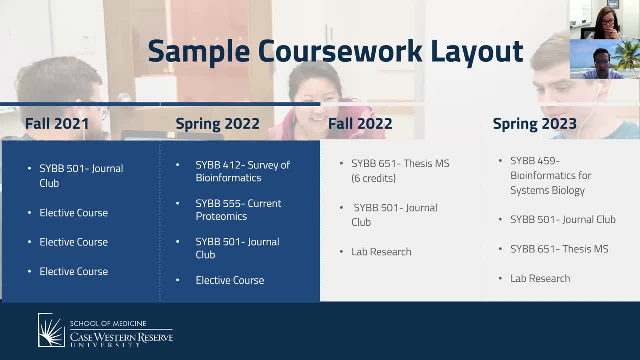 um, and then that second semester we're um, and then that second semester we're going to, going to, going to, to roll you into several different, to roll you into several different, to roll you into several different courses: that um courses, that um courses, that um, that, that will really give you the skills. 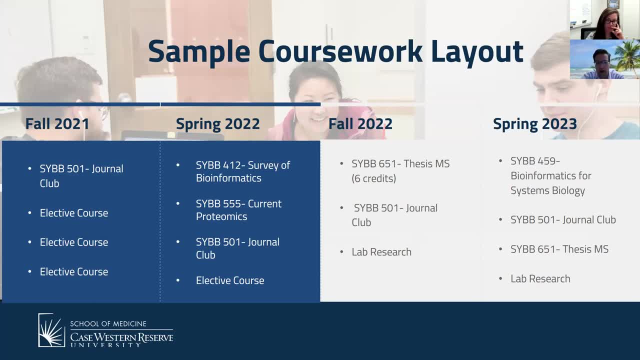 that that will really give you the skills. that that will really give you the skills. and and are two of the required courses. and and are two of the required courses. and and are two of the required courses for graduation. so you'll take one more for graduation. so you'll take one more. 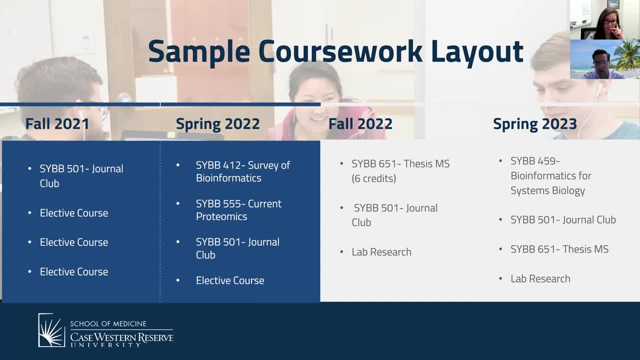 for graduation. so you'll take one more elective there and then elective there, and then elective there and then starting in the fall of 20, or if this starting in the fall of 20, or if this starting in the fall of 20, or if this says 2021, 22. this is just an example. 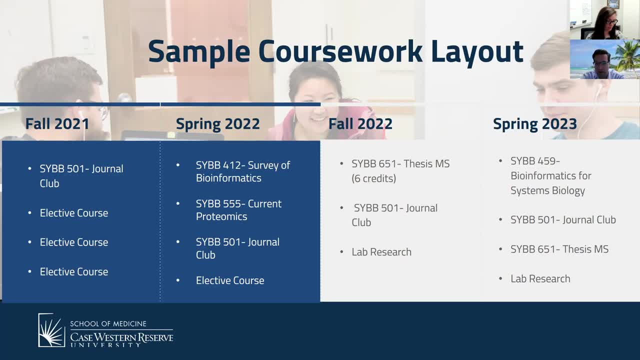 says 2021 22- this is just an example- says 2021 22- this is just an example. um you would start doing your thesis, um you would start doing your thesis, um you would start doing your thesis- research and research, and research, and so you'll take credits of the thesis. 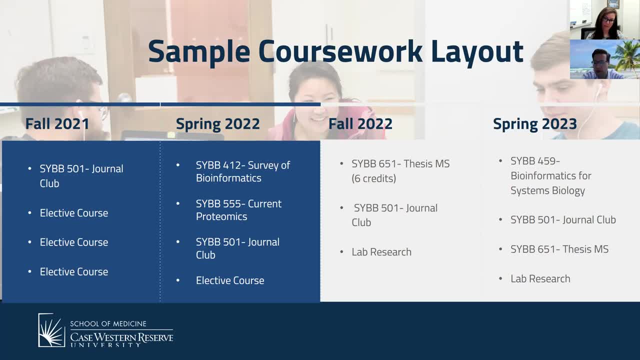 so you'll take credits of the thesis. so you'll take credits of the thesis: research, research, research. and one thing i didn't mention before: we, and one thing i didn't mention before we, and one thing i didn't mention before: we have a journal club, that is, that meets. 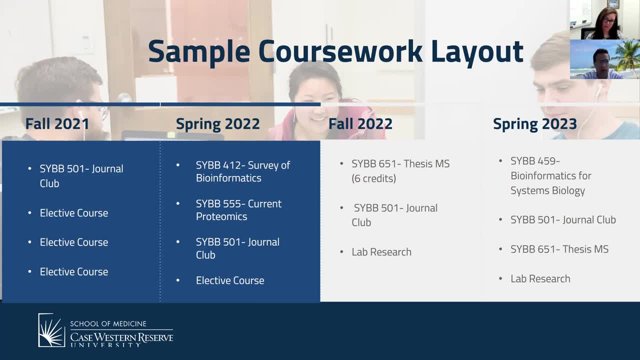 have a journal club that is that meets. have a journal club that is that meets once a once a week every week during once a once a week every week during once a once a week during during the school year, and it's not a during the school year and it's not a. 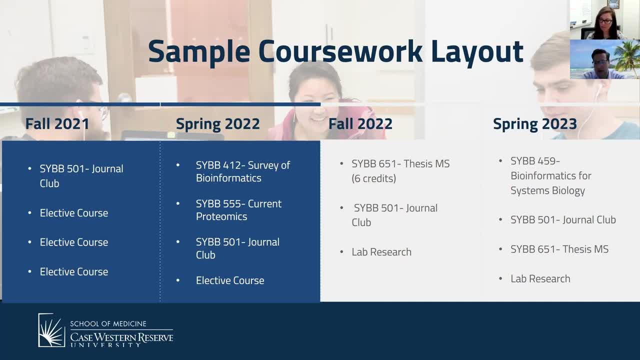 during the school year and it's not a traditional journal club. it really is traditional journal club. it really is traditional journal club. it really is about dissemination of your own work, about dissemination of your own work, about dissemination of your own work. so, as a master's student, you're not. 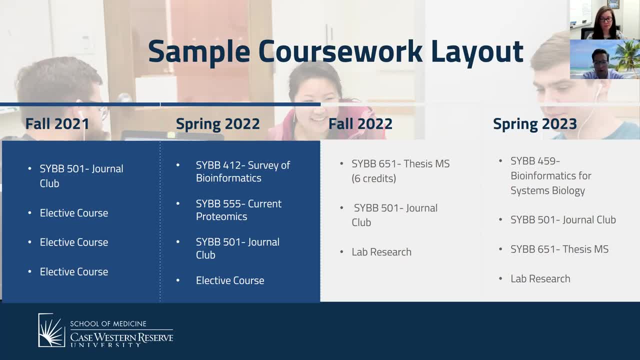 so as a master's student, you're not. so as a master's student, you're not expected to present until year two. expected to present until year two. expected to present until year two. but you'll see all of our sybb phd. but you'll see all of our sybb phd. 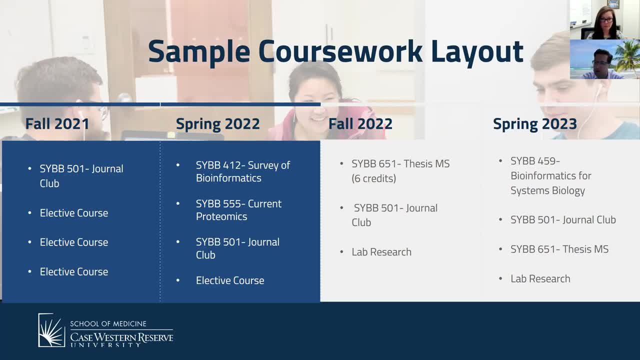 but you'll see all of our sybb phd students present, students present, students present during your first year and they actually during your first year and they actually during your first year and they actually present their own research, present their own research, present their own research and they- it's a relatively we'll call. 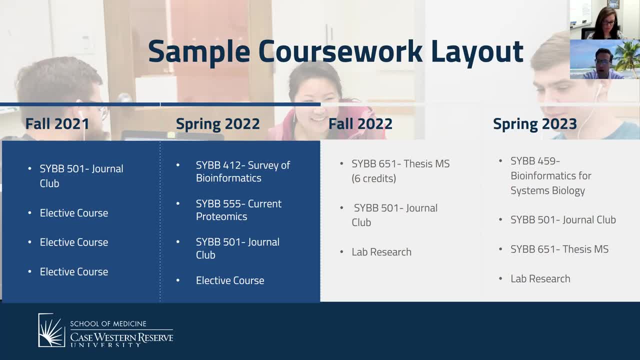 and they, it's a relatively, we'll call, and they, it's a relatively, we'll call it friendly, it friendly, it friendly um environment, to kind of learn how to um environment, to kind of learn how to um environment, to kind of learn how to present, present, present, what you've come up with, and it really 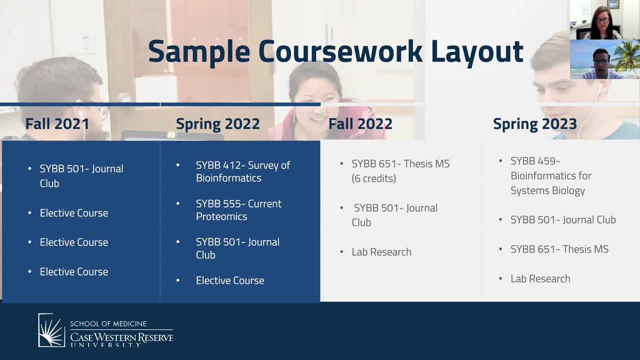 what you've come up with, and it really what you've come up with and it really seems to work quite well, for teaching seems to work quite well. for teaching seems to work quite well for teaching you to really give a good, you to really give a good. 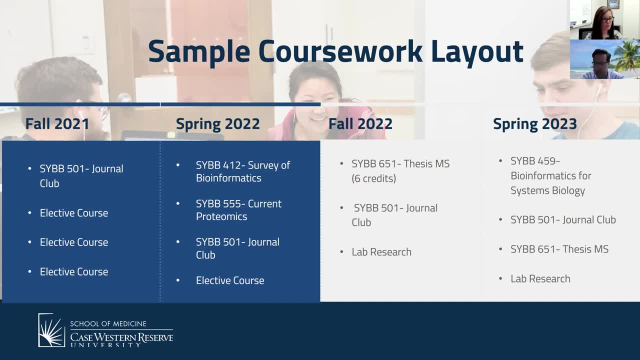 you to really give a good scientific presentation. so you get up scientific presentation. so you get up scientific presentation. so you get up there. you say what you're doing, how it's there. you say what you're doing, how it's there. you say what you're doing, how it's working. 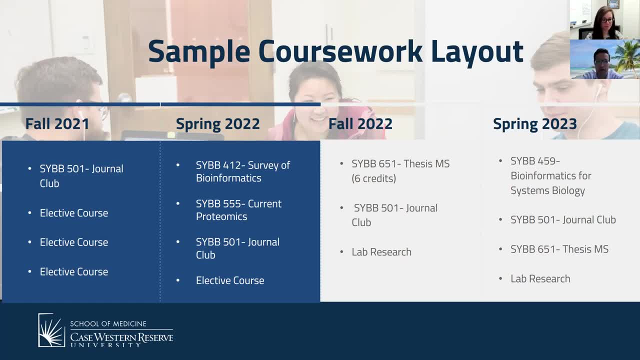 working, working, all of your results and the all of your results, and the all of your results and the it's students in the in the um, it's students in the in the um, it's students in the in the um in the course, actually really kind of run. 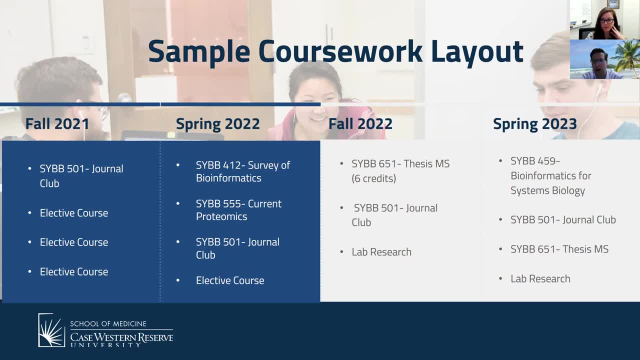 in the course, actually really kind of run in the course, actually really kind of run the whole thing, and they give the whole thing and they give the whole thing and they give really good advice on how do you actually really good advice on, how do you actually really good advice on, how do you actually what would be a better way to do that? 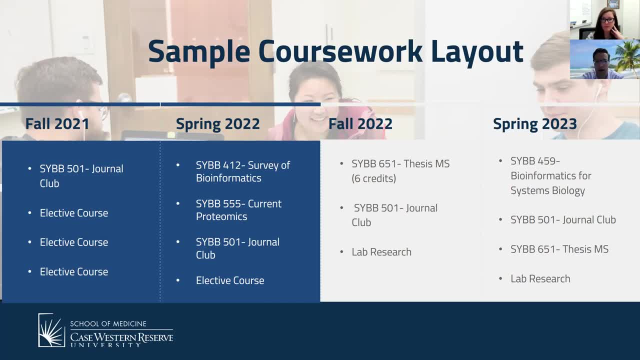 what would be a better way to do that? what would be a better way to do that experiment or experiment, or experiment or um, or how to how to present something a um, or how to how to present something a um, or how to how to present something a little bit more clearly. all that stuff. 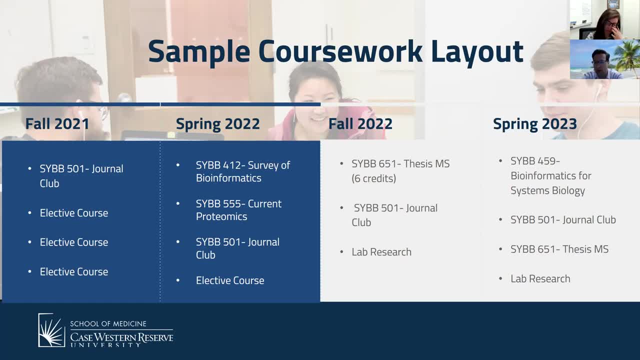 little bit more clearly all that stuff, little bit more clearly, all that stuff. um so, anyway, by the end of spring 2023. um, so, anyway, by the end of spring 2023. um, so, anyway, by the end of spring 2023. hopefully your, your thesis project is. 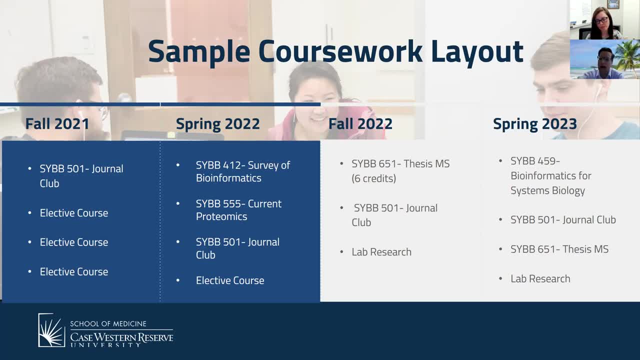 hopefully your your thesis project is, hopefully your your thesis project is done, done, done. if not you can, you can extend by another. if not you can, you can extend by another. if not you can, you can extend by another semester and take another semester of semester and take another semester of. 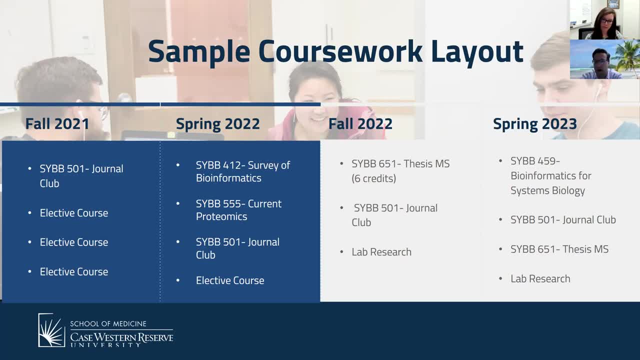 semester and take another semester of the thesis research, the thesis research, the thesis research. but um, we, but we really want you guys to, but um, we, but we really want you guys to, but um, we, but we really want you guys to be done in in four semesters and it's. 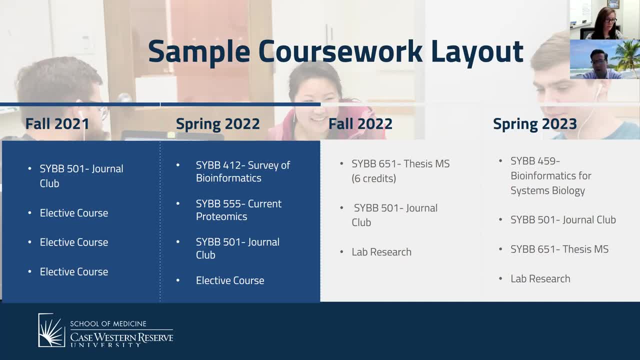 be done in in four semesters. and it's be done in in four semesters and it's totally doable. it's actually doable in totally doable. it's actually doable in totally doable. it's actually doable in three semesters with no real um. 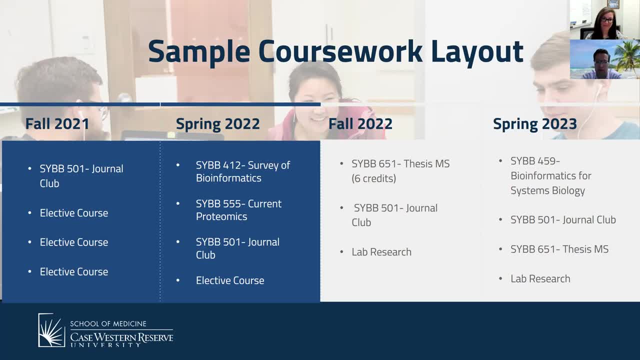 three semesters with no real um. three semesters with no real um. sort of crazy, sort of crazy, sort of crazy class scheduling um. so we've had that class scheduling um. so we've had that class scheduling um. so we've had that. we've had at least one student, that's. 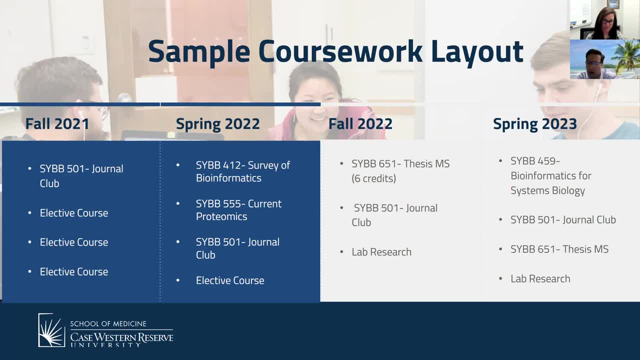 we've had at least one student that's. we've had at least one student that's done it in a, done it in a, done it in a in three semesters, so it is possible. it's in three semesters, so it is possible. it's in three semesters, so it is possible. it's just a little bit more of a tricky. 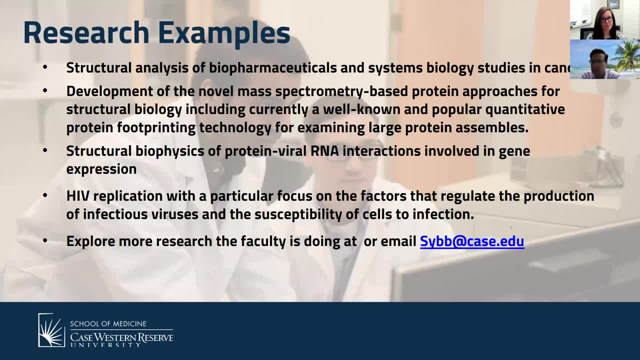 just a little bit more of a tricky, just a little bit more of a tricky, tricky scheduling thing. okay, next slide. okay, next slide. okay, next slide. all right, so a few examples of projects. all right, so a few examples of projects. all right, so a few examples of projects that people who, who have gone through 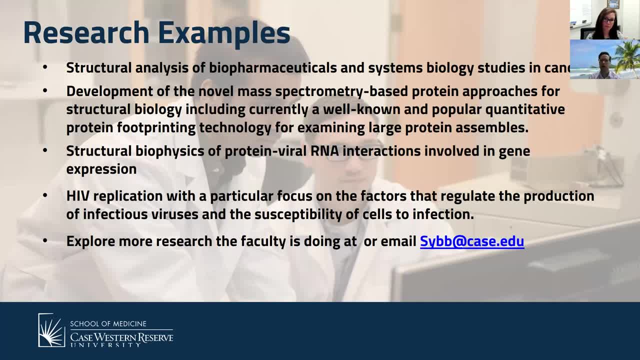 that people who who have gone through that, people who who have gone through the master's degree, the master's degree, the master's degree, have have done so. looking at how have have done so, looking at how have have done so, looking at how, um, how, uh, drugs interact, um. 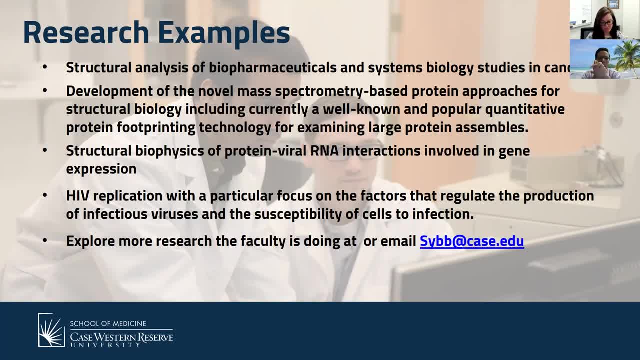 um how uh drugs interact. um um how uh drugs interact um with a target in cancer. um with a target in cancer, um with a target in cancer. um we've had some people work on a mass. we've had some people work on a mass. we've had some people work on a mass spectrometry based. 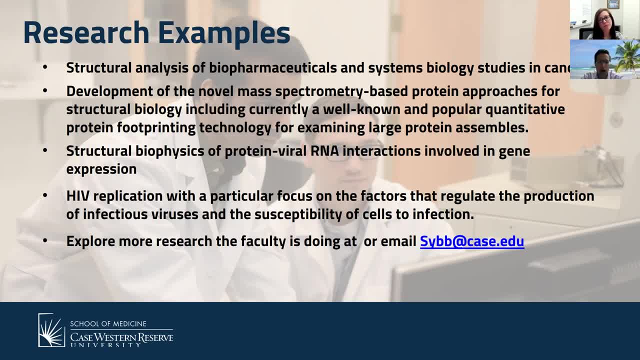 spectrometry based. spectrometry based approach to doing structural biology, approach to doing structural biology, approach to doing structural biology. we've done sort of protein rna, we've done sort of protein rna. we've done sort of protein rna. interactions, interactions, interactions using structural biophysics, um. 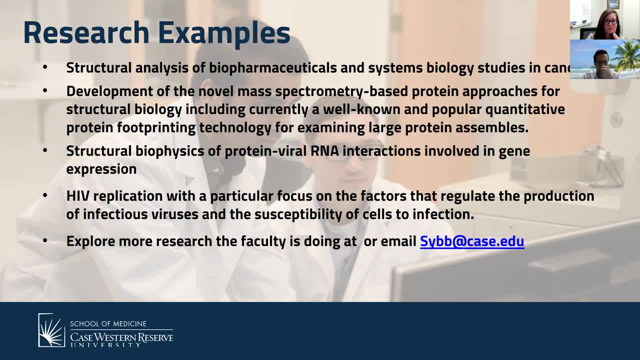 using structural biophysics, um, using structural biophysics, um, aspects of h by hiv, aspects of h by hiv, aspects of h by hiv, replication um, and then replication um, and then replication um, and then you know really the what our, what our, you know really the what our, what our. 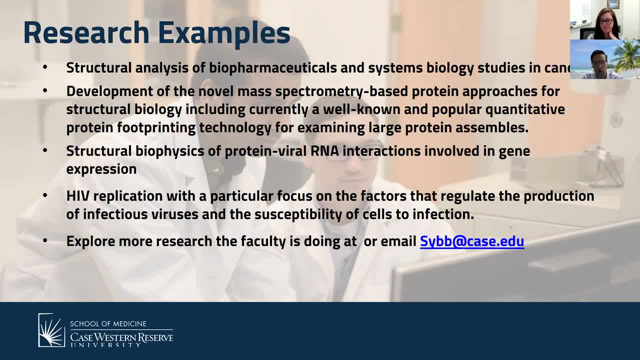 you know, really, the what our, what our research faculty and in the department research faculty and in the department research faculty and in the department are doing is really incredibly varied. we are doing is really incredibly varied. we are doing is really incredibly varied. we have a bunch of people doing coven work. 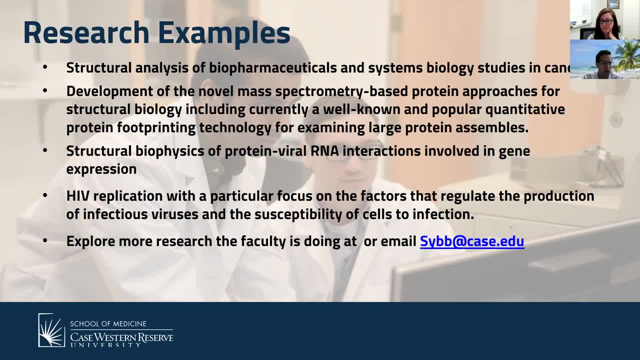 have a bunch of people doing coven work. have a bunch of people doing coven work at this point, at this point, at this point, um, we have people doing structural um, we have people doing structural um, we have people doing structural biology. we have people doing biology. we have people doing 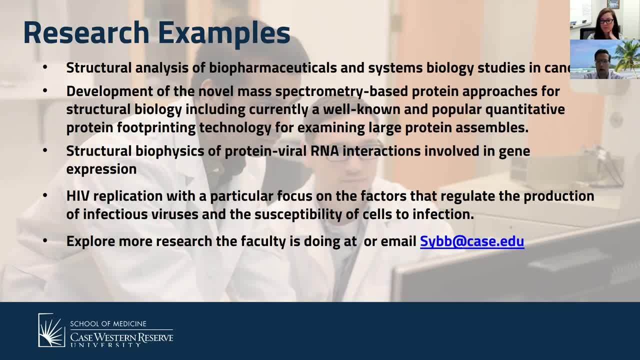 biology. we have people doing structural genetics um uh structural genetics, um uh structural genetics, um uh of of cancer, of of cancer, of of cancer, genetics of alzheimer's disease, um genetics of alzheimer's disease, um genetics of alzheimer's disease. um what else? what else? 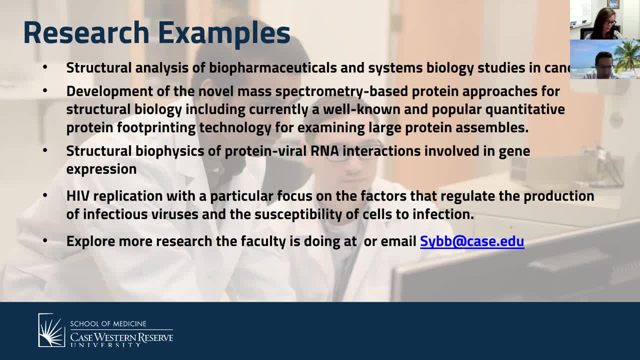 what else? really sort of population level genetics, really sort of population level genetics, really sort of population level genetics and the inheritance of of disease and the inheritance of of disease and the inheritance of of disease. really it just spans a huge slew of. really it just spans a huge slew of of. 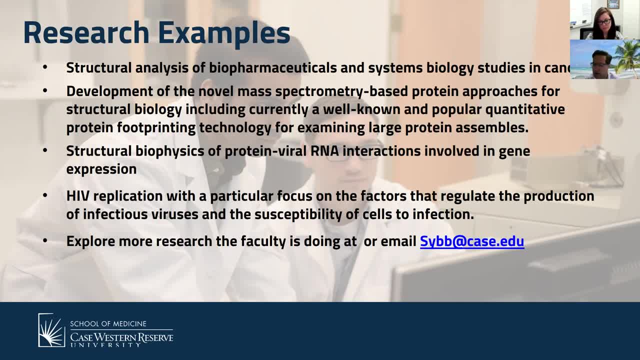 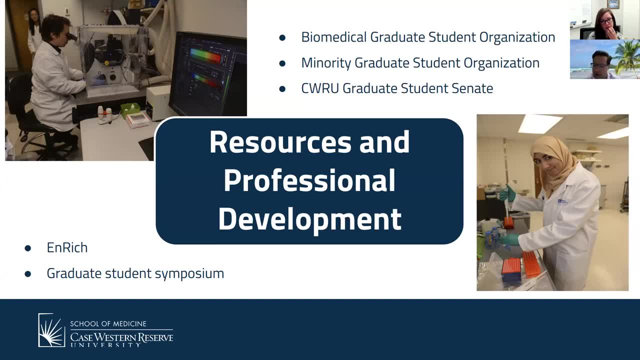 really, it just spans a huge slew of of, of topics, of topics, of topics, um, um, um. so okay, so next slide, so beyond, so beyond, so beyond. or is this where you take over jackie? or is this where you take over jackie? or is this where you take over jackie? right, keep going, it's up to you, you can. right, keep going. it's up to you. you can right, keep going, it's up to you. you can keep going. if you want, oh, i can do it. keep going. if you want, oh, i can do it. keep going. if you want, oh, i can do it. okay, so so. 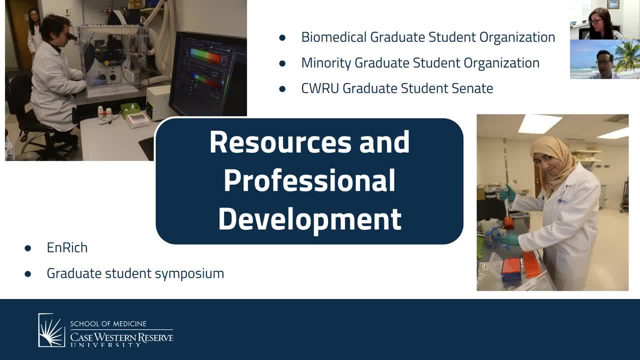 okay, so, so, okay, so so, beyond just the, you know the sort of beyond just the. you know the sort of beyond just the. you know the sort of teaching you the skills that you need to teaching you the skills that you need to teaching you the skills that you need to do a. 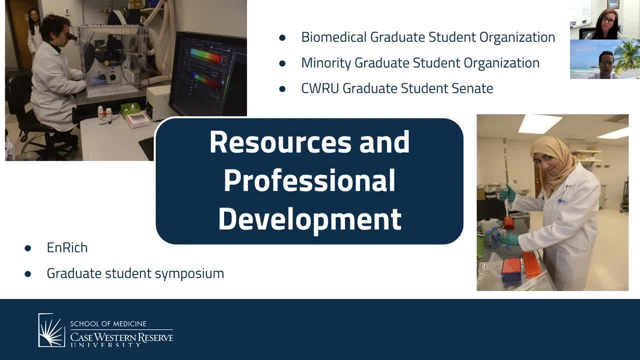 do a, do a do bioinformatics. we want to sort of do bioinformatics. we want to sort of do bioinformatics. we want to sort of develop you do bioinformatics. we want to sort of develop you all the way around, and so we. all the way around, and so we. 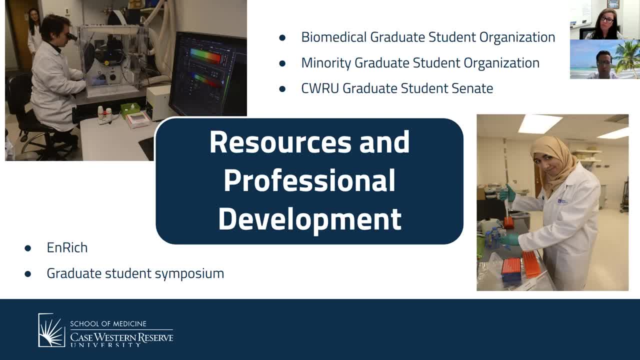 all the way around. and so we have some programs, have some programs, have some programs that exist, that exist, that exist for our masters and phd programs, which, for our masters and phd programs, which, for our masters and phd programs, which are, are geared around professional 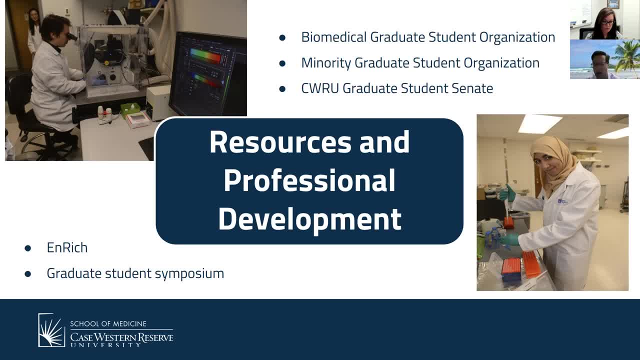 are are geared around professional are are geared around professional development, development, development. so there's this enriched program which i so there's this enriched program which i so there's this enriched program which i don't remember what it stands for. don't remember what it stands for. 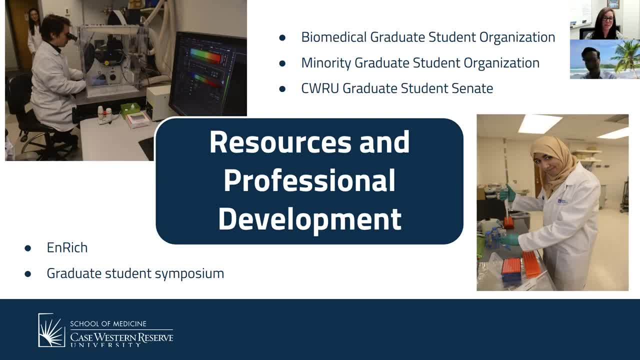 don't remember what it stands for, because this is where jackie's supposed. because this is where jackie's supposed, because this is where jackie's supposed to be talking. to be talking. to be talking. to be fair. i don't remember what it. to be fair, i don't remember what it. 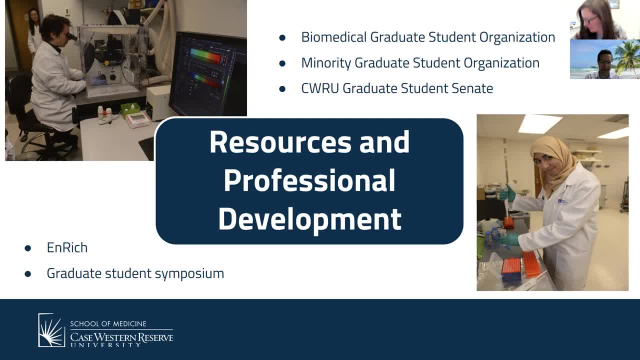 to be fair, i don't remember what it stands for. it always escapes my mind stands for. it always escapes my mind stands for. it always escapes my mind. you see, uh, you know what an acronym. but you see, uh, you know what an acronym. but you see, uh, you know what an acronym. but it really is a program for, for getting 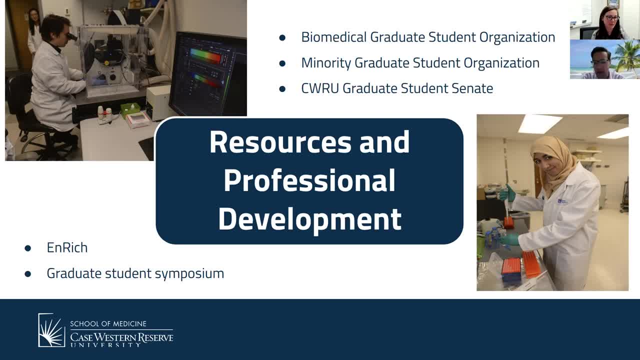 it really is a program for for getting. it really is a program for for getting you to do some, you to do some, you to do some sort of internship, um at outside the sort of internship um at outside, the sort of internship um at outside the university university. 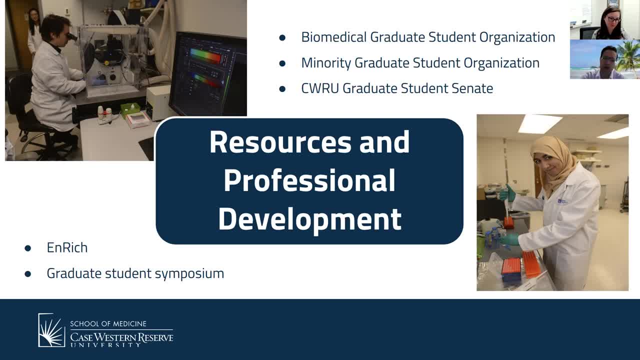 university um we offer a graduate student symposium. um. we offer a graduate student symposium um. we offer a graduate student symposium once a year where you can present your once a year, where you can present your once a year, where you can present your your work um to to other graduate. 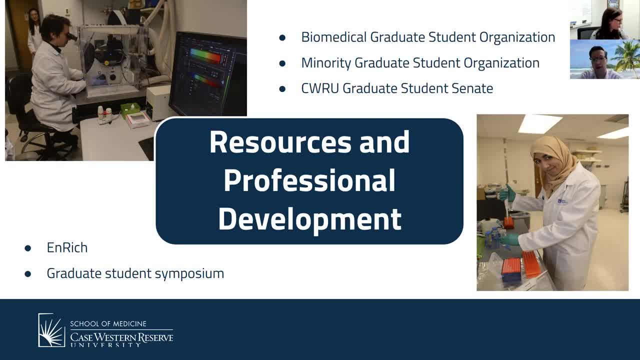 your work um to to other graduate students. there's cash prizes for your students. there's cash prizes for your students. there's cash prizes for your for the best poster, um for the best poster, um for the best poster, um. there's also some- uh, you know, graduate 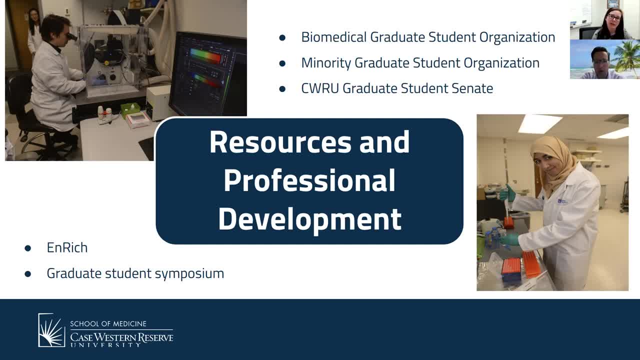 there's also some- uh, you know, graduate. there's also some- uh, you know, graduate- student organizations to support you, student organizations to support you, student organizations to support you. while you're here, the the big one is the. while you're here, the the big one is the. 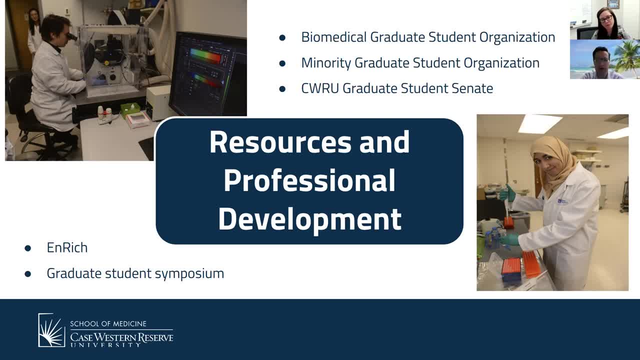 while you're here, the, the big one is the biomedical biomedical graduate student, biomedical biomedical graduate student, biomedical biomedical graduate student organization. so that's for all of the organization. so that's for all of the organization, so that's for all of the masters and phd level students at. 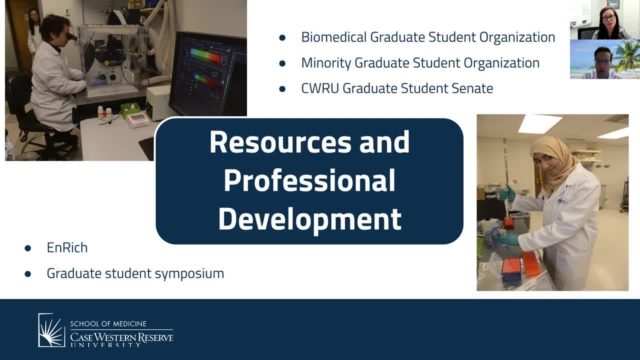 masters and phd level students at masters and phd level students at in the school of medicine. there's also in the school of medicine. there's also in the school of medicine. there's also a minority graduate student, a minority graduate student, a minority graduate student organization to help to, to um. 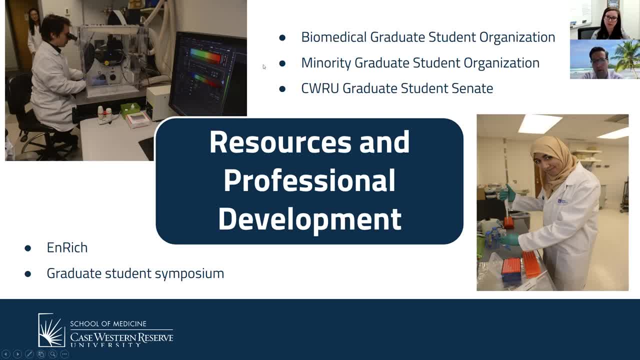 organization to help to to um organization to help to to um. represent uh. concerns for represent uh. concerns for represent uh. concerns for underrepresented minorities and underrepresented minorities and underrepresented minorities and underrepresented uh individuals in underrepresented uh individuals. in underrepresented uh individuals in in sort of in medicine and research, and. 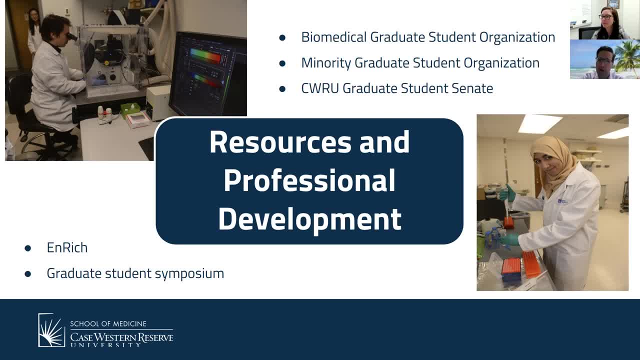 in sort of in medicine and research, and in sort of in medicine and research. and then there's also, then there's also, then there's also, if you really, if you really want to, if you really, if you really want to, if you really, if you really want to embrace this, there's also a graduate. 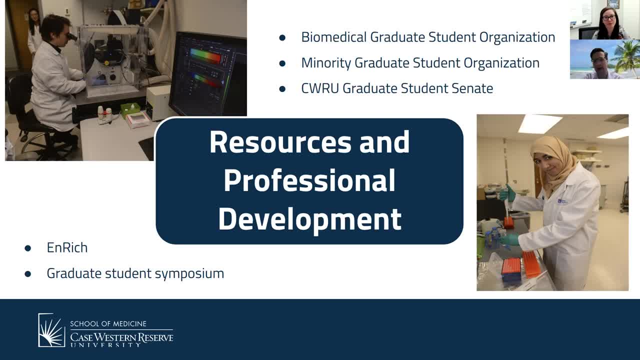 embrace this. there's also a graduate. embrace this. there's also a graduate student senate, which isn't just the student senate, which isn't just the student senate, which isn't just the school of medicine, it's the entire school of medicine. it's the entire school of medicine, it's the entire university, because we have almost as 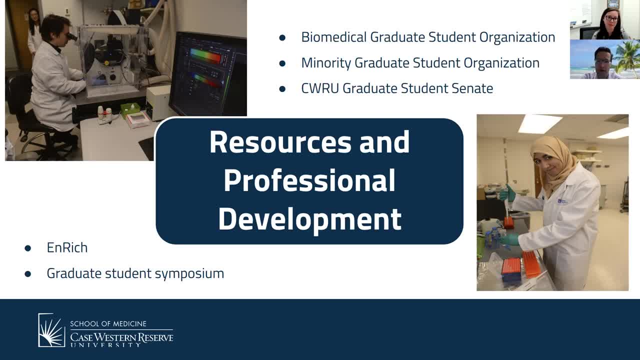 university, because we have almost as university, because we have almost as many, many, many. we probably have only one tenth of the. we probably have only one tenth of the. we probably have only one tenth of the. the number of graduate students in the. the number of graduate students in the. 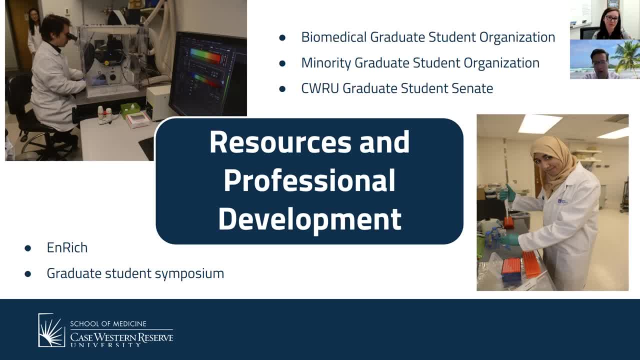 the number of graduate students in the school of medicine, as there are in all school of medicine, as there are in all school of medicine, as there are in all the other students, the other students, the other students in all the other graduate schools, as in all the other graduate schools, as. 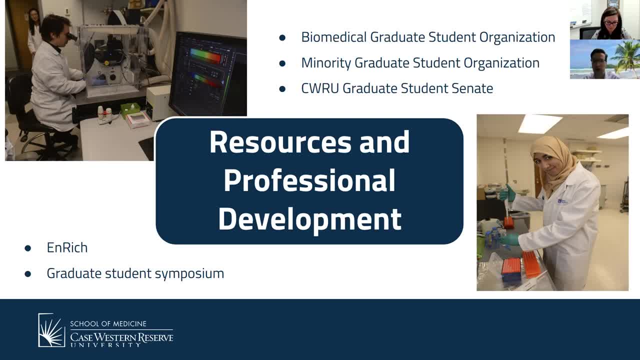 in all the other graduate schools as well. so there's really a huge amount of well. so there's really a huge amount of well, so there's really a huge amount of graduate students here and so graduate students here and so, and these things will help with, and these things will help with. 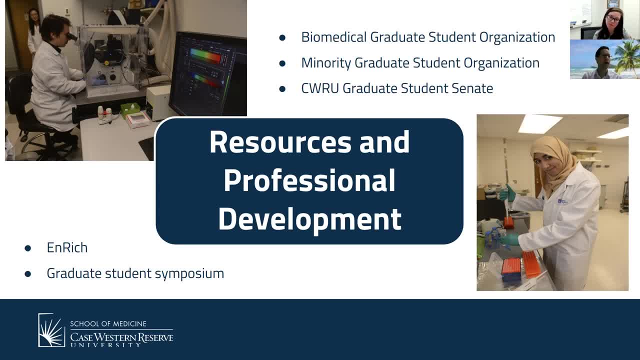 and these things will help with governance of governance of, governance of of the of programs and how you know how of the of programs and how you know how of the of programs and how you know how the the rules and regulations that the, the rules and regulations that. 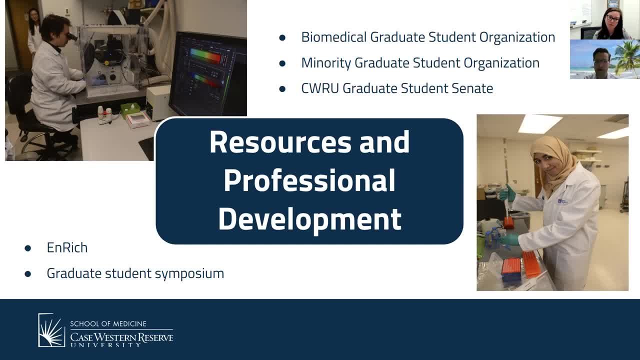 the, the rules and regulations that that students, uh, you know that students, uh, you know that students, uh, you know- get to write for themselves and how get to write for themselves and how get to write for themselves and how things are run and you can give. things are run and you can give. 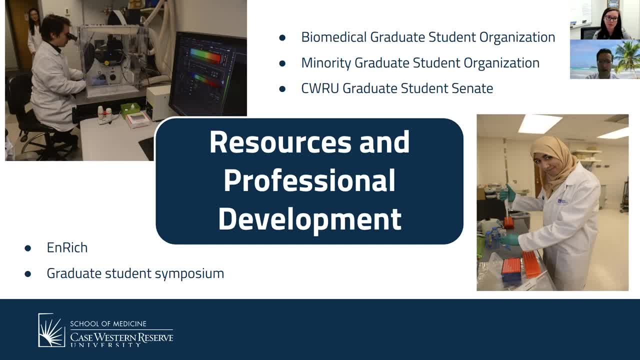 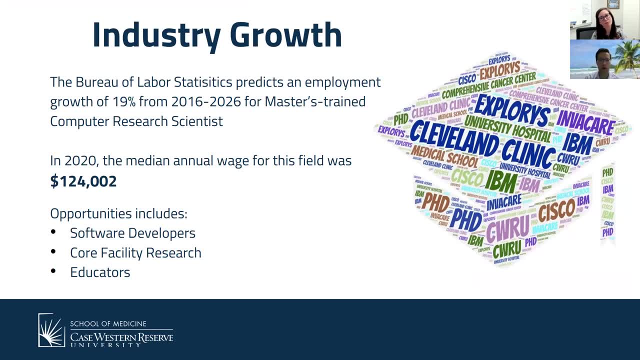 things are run and you can give your, your opinions to the your, your opinions to the your, your opinions to the administration on how things are going. administration on how things are going. administration on how things are going. okay, next slide. so another thing, you know we like to. 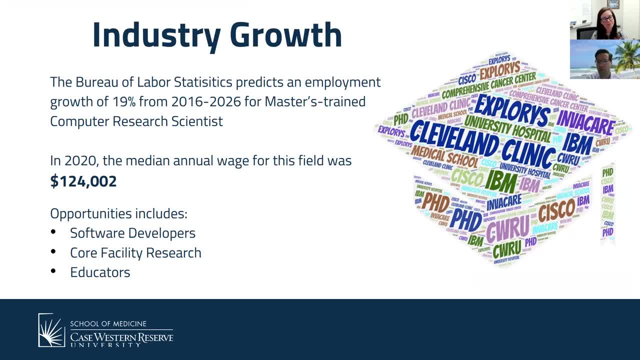 so another thing you know we like to. so another thing you know we like to tell you: is you know this is really a tell you? is you know this is really a tell you? is you know this is really a? the sort of informatics field is an? 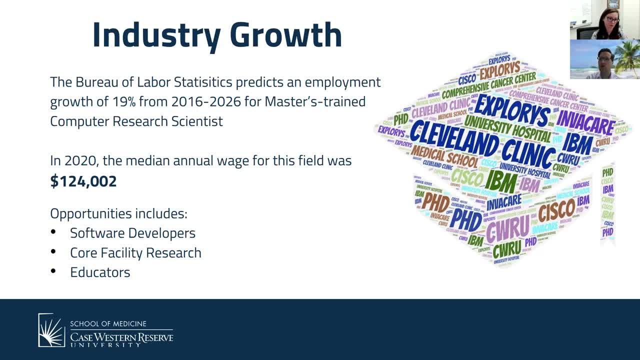 the sort of informatics field is an. the sort of informatics field is an amazingly, amazingly, amazingly great um training, great um training, great um training that you can really take immediately, that you can really take immediately, that you can really take immediately and go go work at a um. 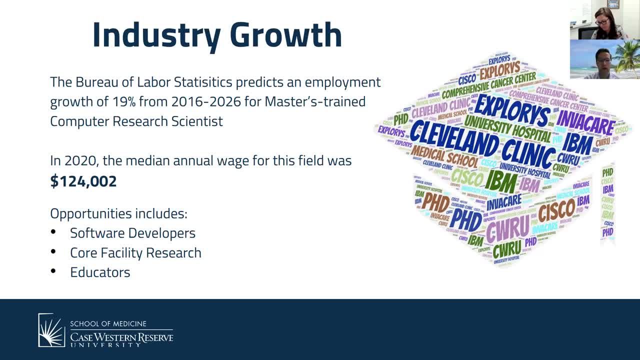 and go go work at a um and go go work at a um. you know in what we call industry um. you know in what we call industry um. you know in what we call industry um. so so, so. median wage for for a bioinformatician. median wage for for a bioinformatician. 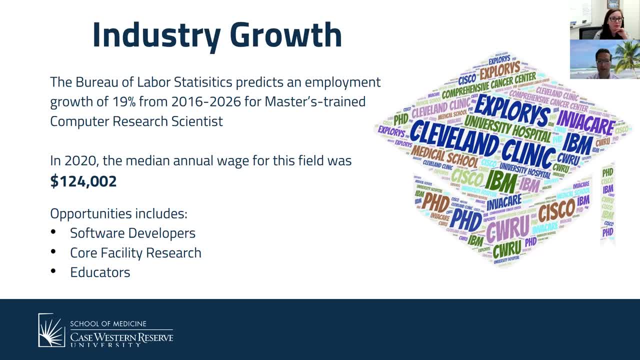 median wage for for a bioinformatician is 124 thousand dollars. is 124 thousand dollars? is 124 thousand dollars um opportunities that you can you can do. um opportunities that you can you can do. um opportunities that you can you can do as a software developer core facility. 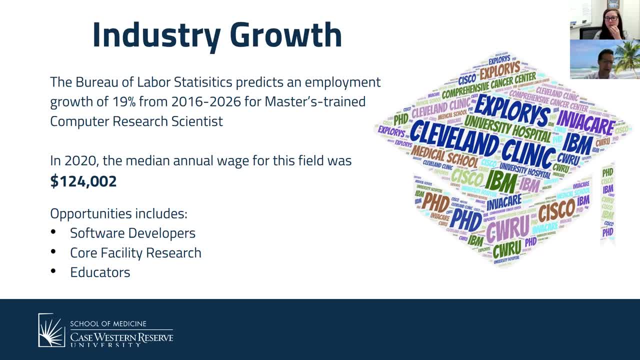 as a software developer core facility, as a software developer core facility. research an educator- really staff i. research an educator- really staff. i research an educator- really staff i. there should be another bullet point. there should be another bullet point. there should be another bullet point here that says staff bioinformatician. 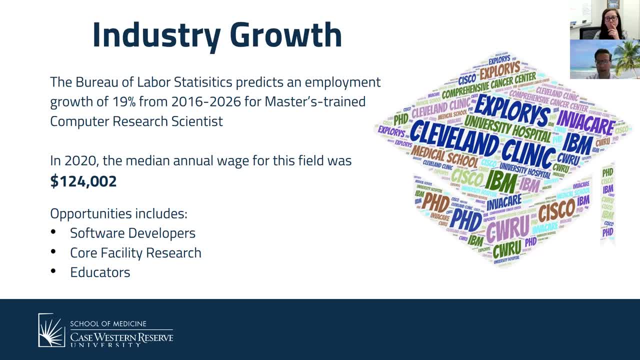 here that says staff bioinformatician. here that says staff bioinformatician. so master's levels level people often so master's levels level people often so master's levels level people often end up in the end up in the end up in the in the uh. 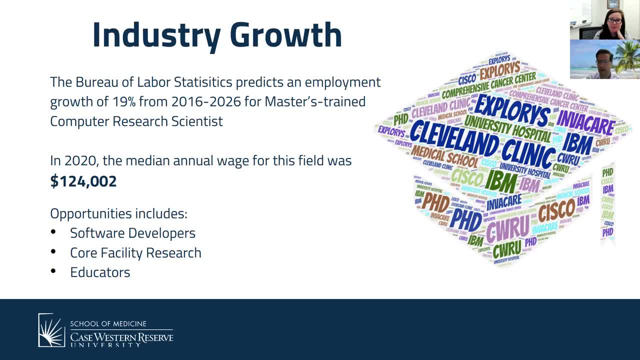 in the uh, in the uh, working as a, working as a, working as a um informatician in a laboratory, that um informatician in a laboratory, that um informatician in a laboratory, that really seems to be a very, really seems to be a very. 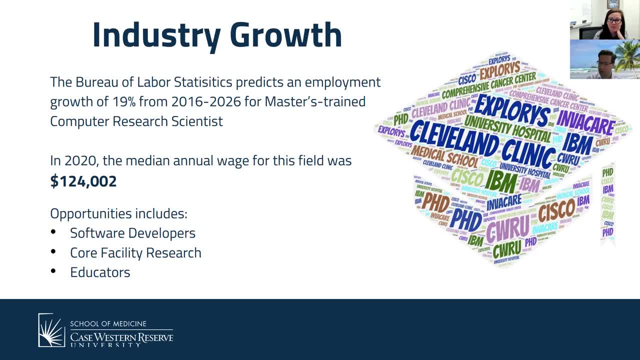 really seems to be a very common place to end up with, common place to end up with, common place to end up with. there are opportunities in cleveland. there are opportunities in cleveland. there are opportunities in cleveland itself, itself itself, for doing some of this: informatics, and so. 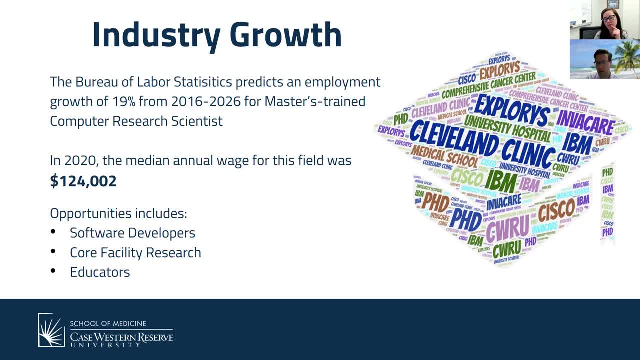 for doing some of this informatics, and so for doing some of this informatics, and so you know, it isn't just that, once you get, you know, it isn't just that once you get you know, it isn't just that once you get your master's degree, you 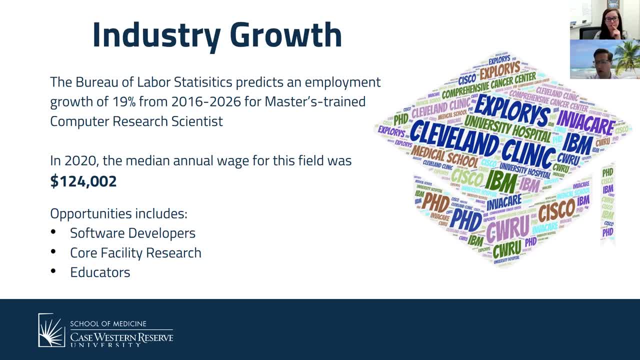 your master's degree, you your master's degree, you have to go to another city or whatever, have to go to another city or whatever, have to go to another city, or whatever. there are certainly are opportunities. there are certainly are opportunities. there are certainly are opportunities, um, in several different. 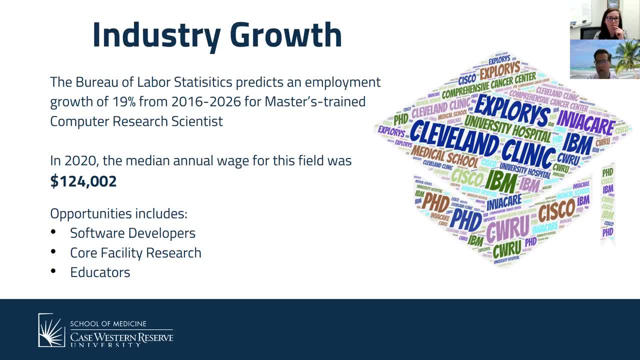 um in several different um in several different um sort of big entities here, exploracus. um sort of big entities here, exploracus, um sort of big entities here. exploracus and ibm both have really large um and ibm both have really large um and ibm both have really large um. cleveland offices here, the cleveland. 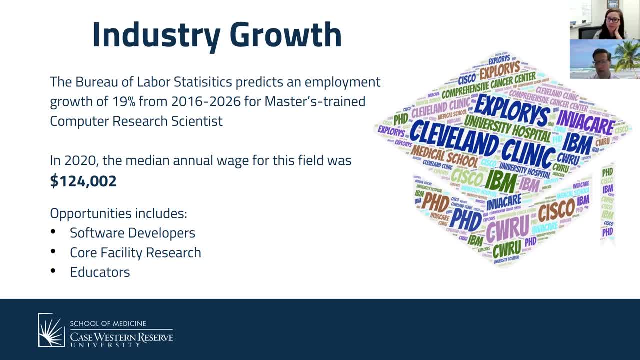 cleveland offices. here the cleveland cleveland offices, here the cleveland clinic clinic, clinic in case western. both have um really in case western. both have um really in case western, both have um really big bioinformatics needs in the big bioinformatics needs in the big bioinformatics needs in the laboratory. so beyond: 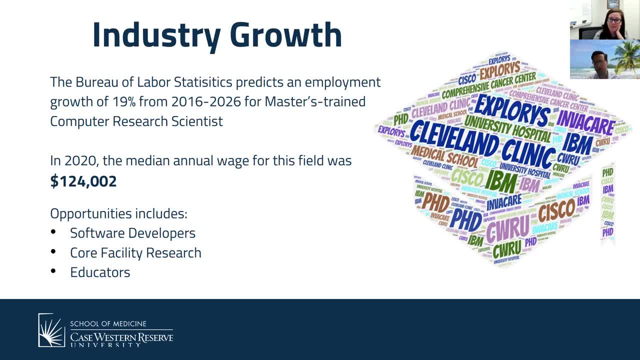 laboratory. so beyond laboratory, so beyond learning as students there, there are learning as students there. there are learning as students there. there are tons of laboratories that really need an, tons of laboratories that really need an, tons of laboratories that really need an informatician- informatician. 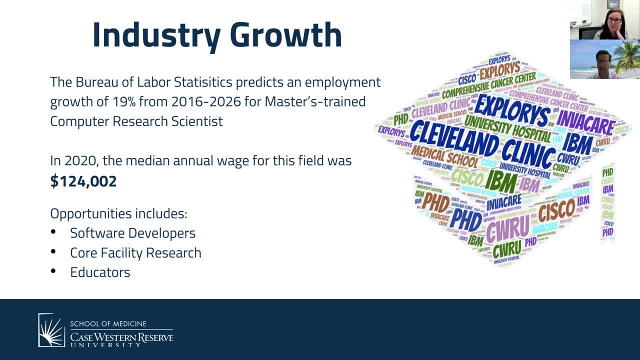 informatician to really tell them what their data, to really tell them what their data, to really tell them what their data means. and so that's really you know. once means, and so that's really you know, once means, and so that's really you know, once you have the masters, that's. 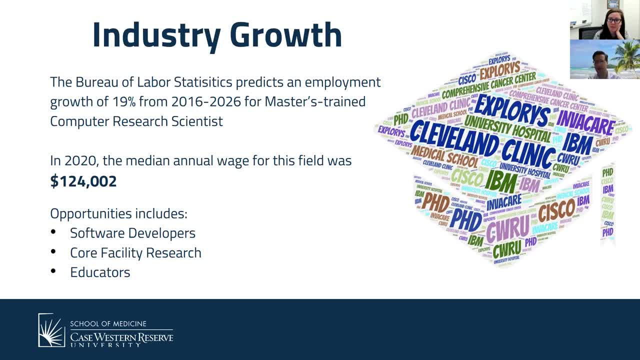 you have the masters. that's: you have the masters. that's that's why that's what people hire you to. that's why that's what people hire you to. that's why that's what people hire you. to do is to make sense out of the giant. 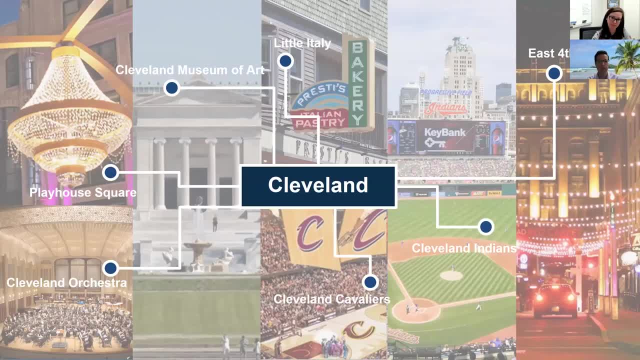 do is to make sense out of the giant do is to make sense out of the giant. data that they can't make sense- okay. data that they can't make sense- okay. data that they can't make sense- okay. next slide: um, so there's lots of things to do in. 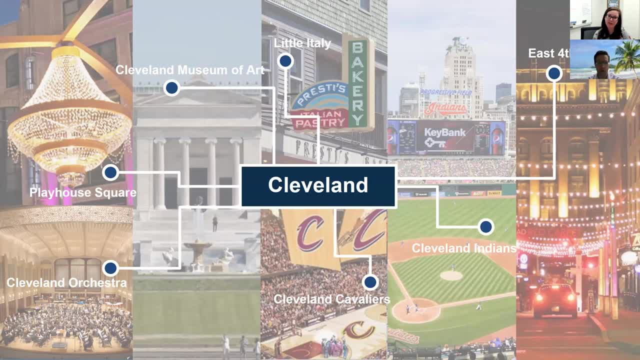 um. so there's lots of things to do in um. so there's lots of things to do in cleveland um beyond um. so there's lots of things to do in cleveland, um beyond um. so there's lots of things to do in cleveland um beyond staying in the lab and working um. 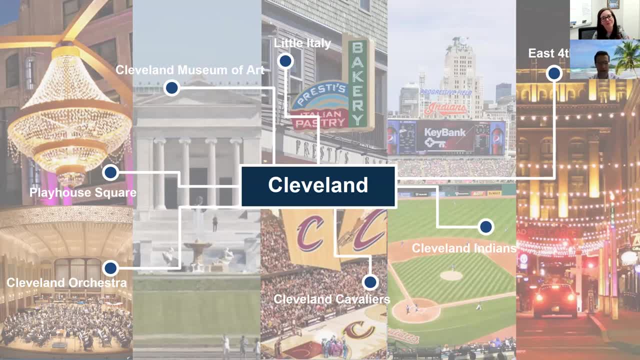 staying in the lab and working um. staying in the lab and working um. playhouse square is is if you like. if playhouse square is is if you like. if playhouse square is is if you like. if you like the theater, it's the second. you like the theater? it's the second. 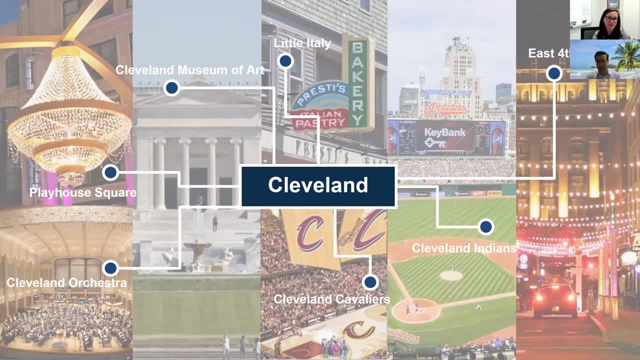 you like the theater. it's the second largest, um, largest, um largest um sort of city theater in the united sort of city theater in the united sort of city theater in the united states. the cleveland museum of art i states. the cleveland museum of art i. 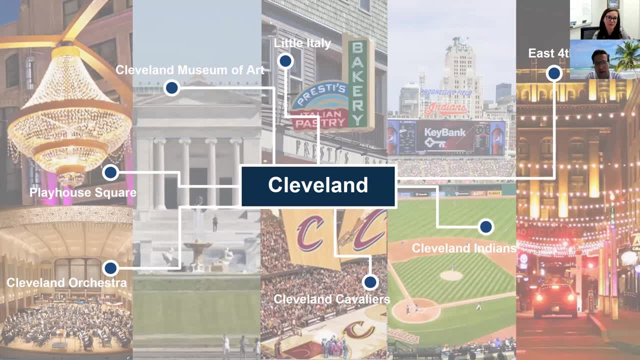 states. the cleveland museum of art, i think, has the largest free collection of think, has the largest free collection of think, has the largest free collection of art in the united states. it really is art in the united states. it really is art in the united states. it really is, and um, if you look, if you squint, really 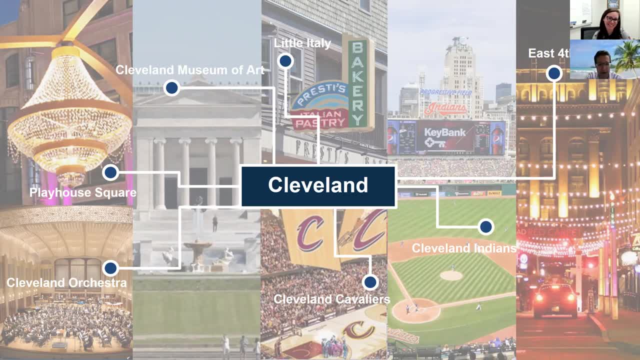 and um, if you look, if you squint really, and um, if you look, if you squint really hard, there's a hard, there's a hard, there's a rodan's thinker which is right there, rodan's thinker which is right there, rodan's thinker which is right there, sitting right in front. um, so that very. 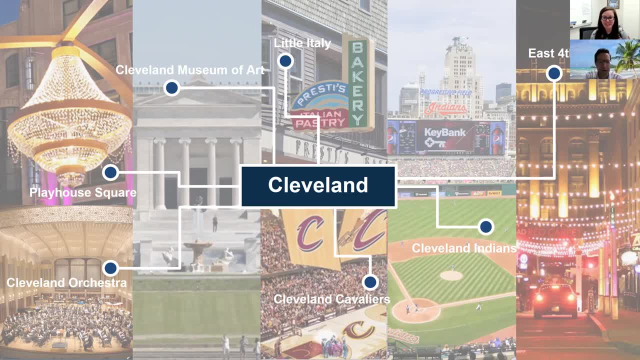 sitting right in front, um, so that very sitting right in front, um, so that very famous guy who's kind of sitting there, famous guy who's kind of sitting there, famous guy who's kind of sitting there and thinking and thinking and thinking um is one of those. is right in front. 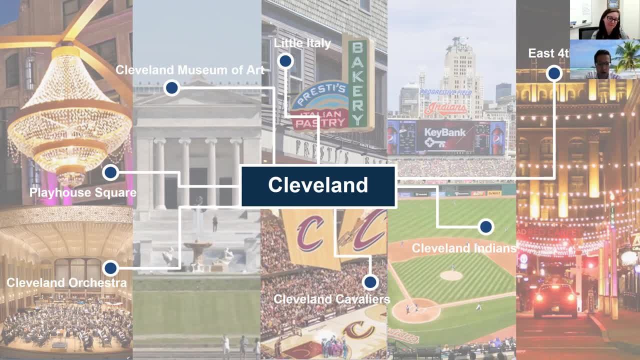 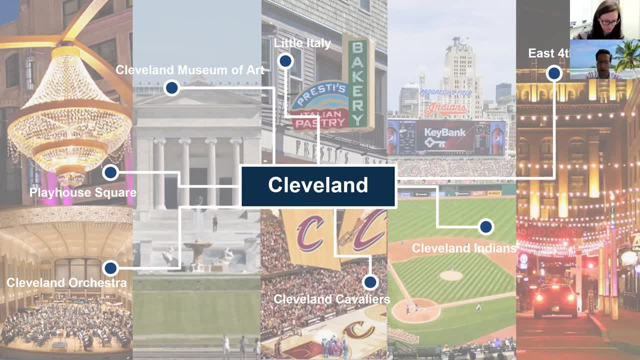 the cleveland symphony are really. the cleveland symphony are really amazing, amazing, amazing. the orchestra meets inside in the. the orchestra meets inside in the. the orchestra meets inside. in the wintertime the symphony meets outside. wintertime, the symphony meets outside. 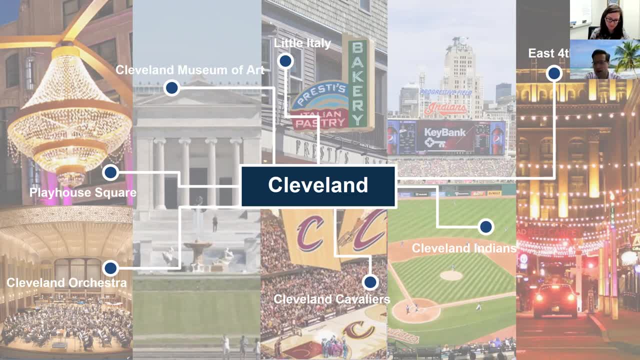 wintertime the symphony meets outside, a little bit away from cleveland, in the, a little bit away from cleveland. in the, a little bit away from cleveland. in the summer you can go sit on the grass, and summer you can go sit on the grass and. 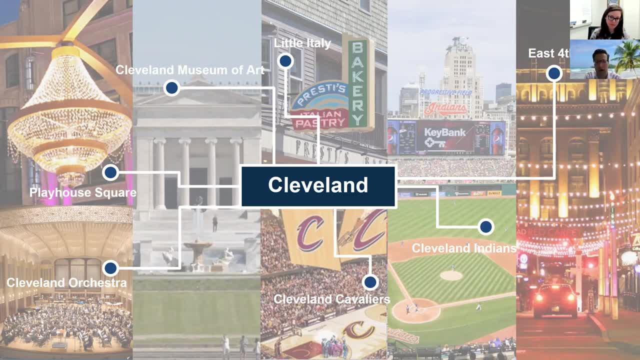 summer you can go sit on the grass and listen, to listen, to listen to all kinds of great music. um, there's a all kinds of great music. um, there's a all kinds of great music. um, there's a lot of lot of lot of ethnic sort of there's like little. 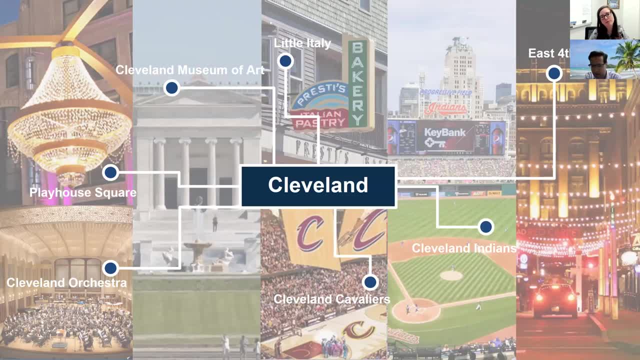 ethnic sort of there's like little. ethnic sort of there's like little. italy is right by campus. they're really italy is right by campus. they're really italy is right by campus. they're really great italian food, if that's something. great italian food, if that's something. 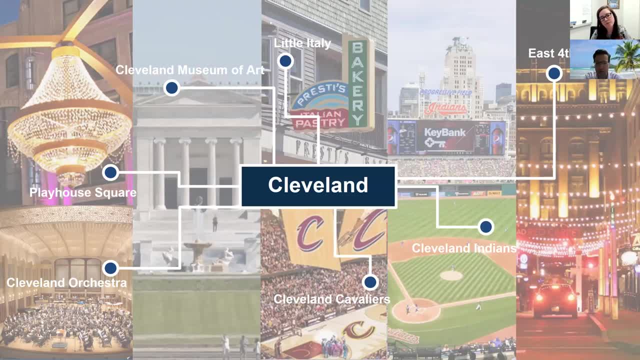 great italian food, if that's something that you like. there's a lot of sports. i'm that you like there's a lot of sports. i'm that you like there's a lot of sports. i'm not sure why football is not on this. not sure why football is not on this. 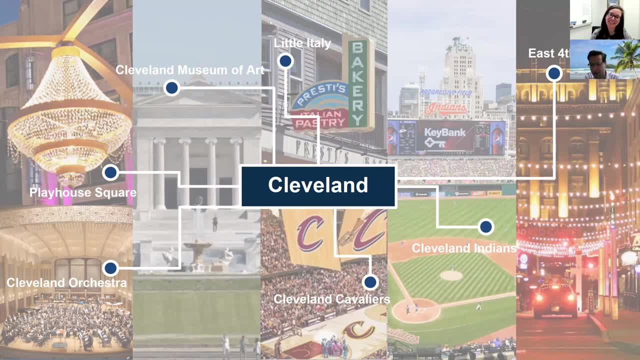 not sure why football is not on this, on this slide, but we have the cavaliers on this slide, but we have the cavaliers on this slide, but we have the cavaliers, the indians and the browns, the indians and the browns, the indians and the browns, um, and then there's a lot of nightlife. 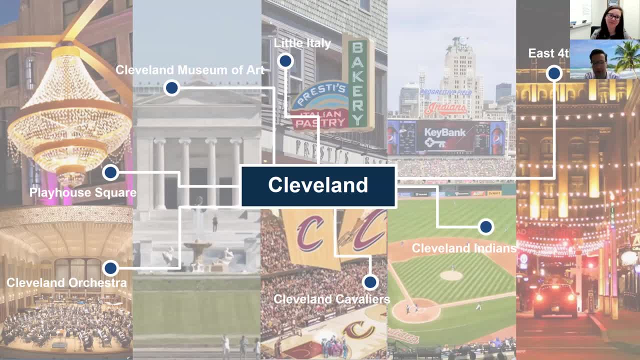 um, and then there's a lot of nightlife, um, and then there's a lot of nightlife, too, downtown. you really can you, if you, too, downtown, you really can you, if you too, downtown, you really can you, if you, if you like that kind of thing there, if you like that kind of thing there. 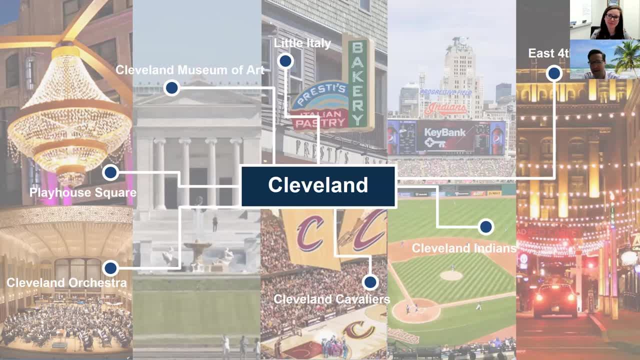 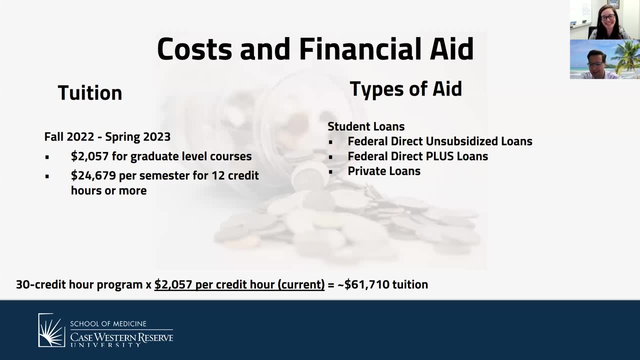 if you like that kind of thing. there really is a very young and hip kind of, really is a very young and hip kind of, really is a very young and hip kind of thing to do in downtown. okay, next slide, okay, next slide, okay, next slide, okay. so this is where i let jackie take. 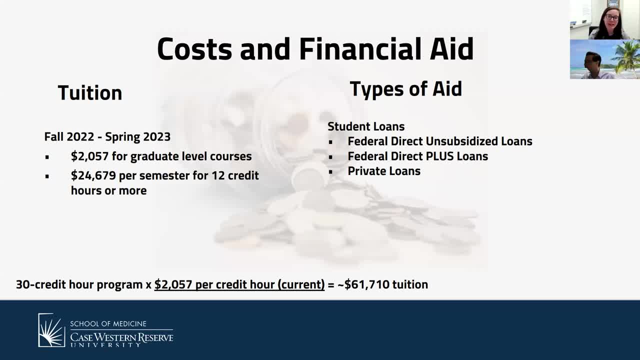 okay, so this is where i let jackie take. okay, so this is where i let jackie take. okay, so i work more on the enrollment. okay, so, i work more on the enrollment. okay, so i work more on the enrollment and admission side. so, and admission side so. 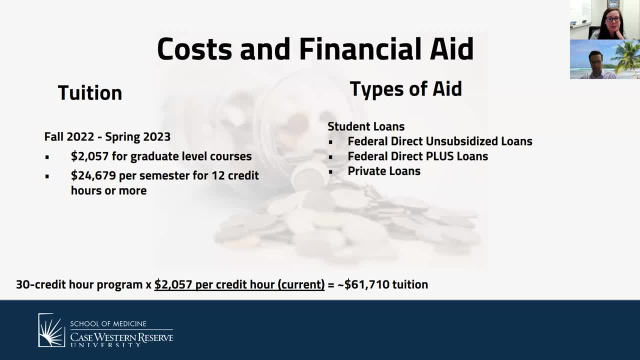 and admission side. so let's just go over the current tuition. let's just go over the current tuition. let's just go over the current tuition and cost of cwru so currently. and cost of cwru so currently. and cost of cwru so currently for our fall spring rate: it is 2057. 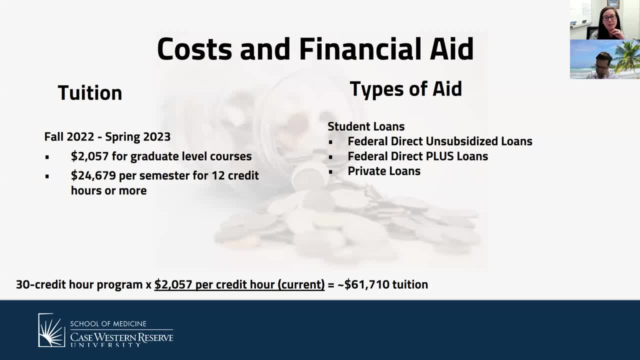 for our fall spring rate: it is 2057. for our fall spring rate: it is 2057. a credit hour for graduate level, a credit hour for graduate level, a credit hour for graduate level coursework, and that does top out at 12 coursework and that does top out at 12. 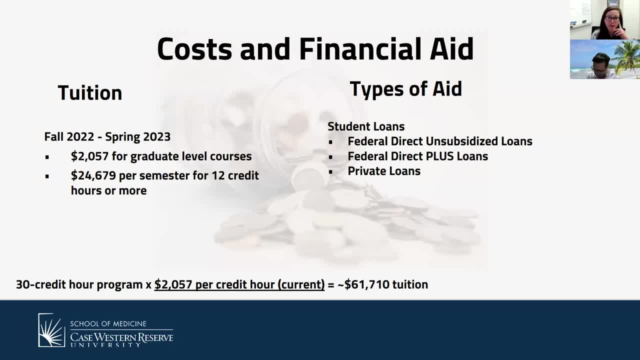 coursework and that does top out at 12 credit hours. so if you wanted to get credit hours, so if you wanted to get credit hours, so if you wanted to get very ambitious and take more than 12, very ambitious and take more than 12, very ambitious and take more than 12 credit hours, let's say 15 credit hours. 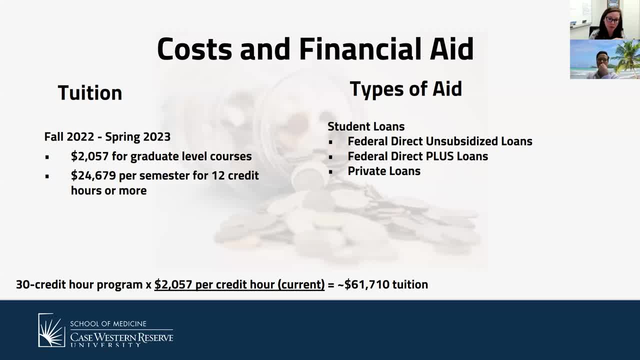 credit hours, let's say 15 credit hours. credit hours- let's say 15 credit hours- in one semester. you would only be in one semester. you would only be in one semester. you would only be getting charged for 12. so that, getting charged for 12, so that. 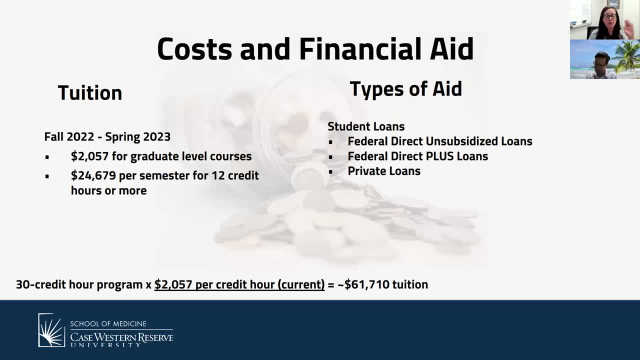 getting charged for 12, so that additional three, additional three, additional three would not count. so for the program in would not count. so for the program in would not count. so for the program in total, if you were to total, if you were to total, if you were to do the 30 credit hours and not do more, 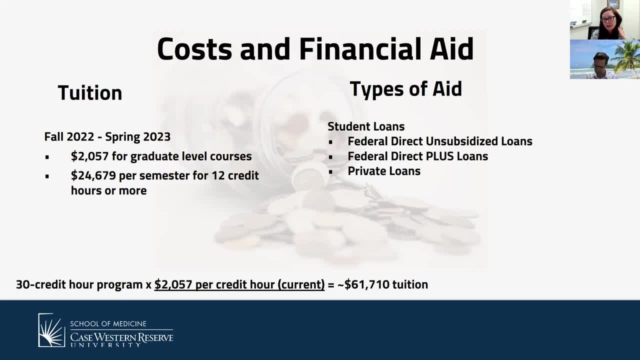 do the 30 credit hours and not do more. do the 30 credit hours and not do more than 12 each semester. that's going to than 12 each semester. that's going to than 12 each semester. that's going to equate to sixty one thousand seven. 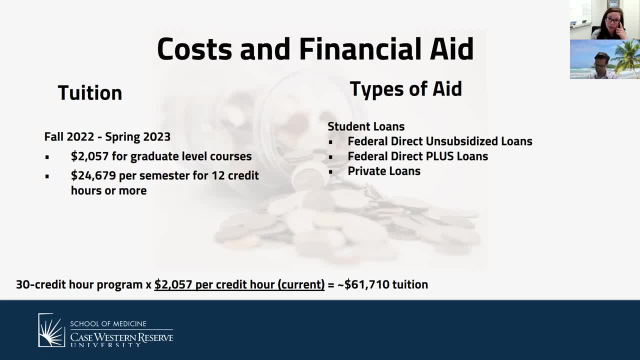 equate to sixty one thousand seven, equate to sixty one thousand seven hundred and ten dollars for a grand hundred and ten dollars, for a grand hundred and ten dollars for a grand total, total total. um, we do offer a few types of aid. um, we do offer a few types of aid. 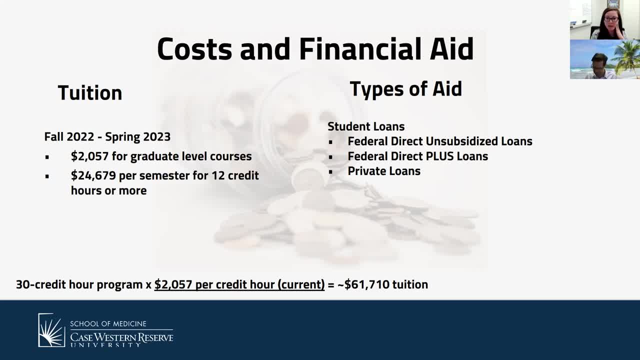 um, we do offer a few types of aid. there are most of our students fund. there are most of our students fund. there are most of our students fund themselves through scholarships and themselves through scholarships, and themselves through scholarships and loans. loans, loans, um, but our financial aid office will. 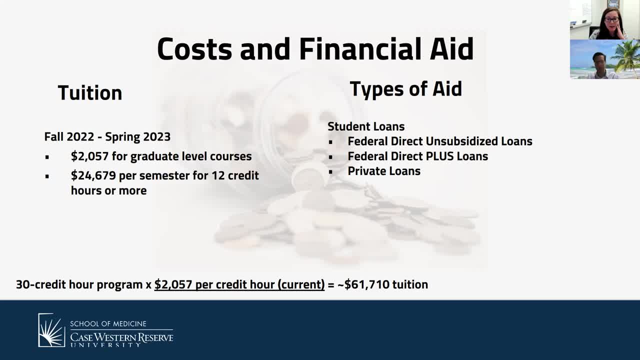 um, but our financial aid office will um, but our financial aid office will work with you for any federal direct work with you, for any federal direct work with you, for any federal direct loans that they can, loans that they can, loans that they can. so, application process, our application: 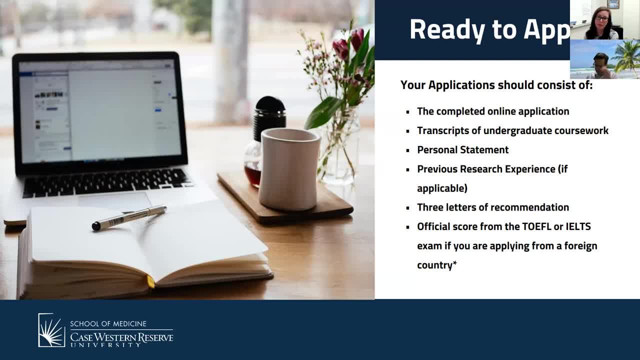 so application process, our application. so application process, our application process is pretty simple. process is pretty simple. process is pretty simple. you will complete an online application. you will complete an online application. you will complete an online application. that is basically just demographic. that is basically just demographic. that is basically just demographic information on you. 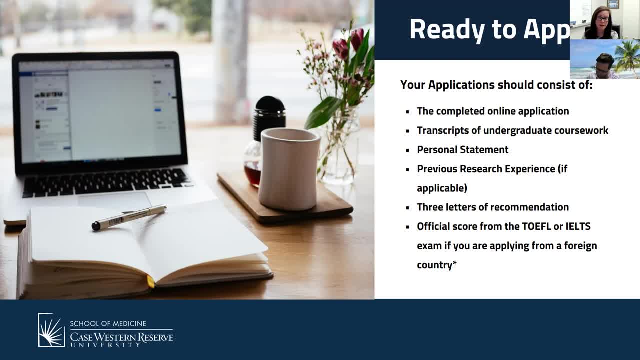 information on you. information on you. we ask for your undergraduate. we ask for your undergraduate. we ask for your undergraduate transcripts. these can be unofficial transcripts. these can be unofficial transcripts. these can be unofficial transcripts. transcripts, transcripts, but if, but, if, but if you are enrolled into the program, you. 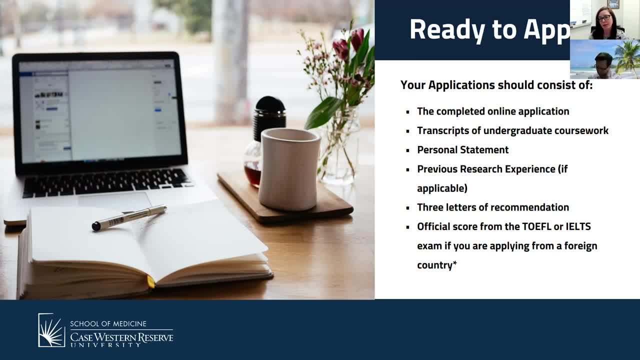 you are enrolled into the program. you you are enrolled into the program, you will need to send official transcripts, will need to send official transcripts, will need to send official transcripts to our graduate student studies office, to our graduate student studies office, to our graduate student studies office. we ask for a personal statement which. 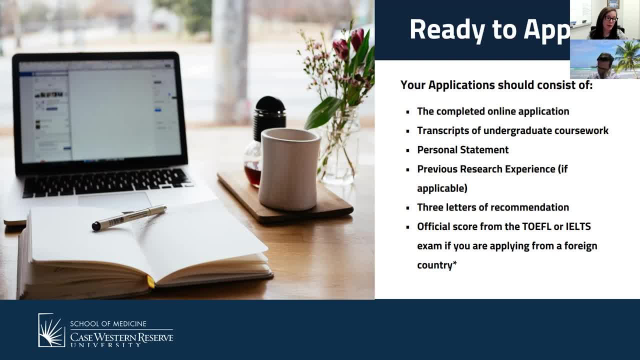 we ask for a personal statement. which we ask for a personal statement which is just a one to two page about you, is just a one to two page about you, is just a one to two page about you, what you've done in the past, what you've done in the past. 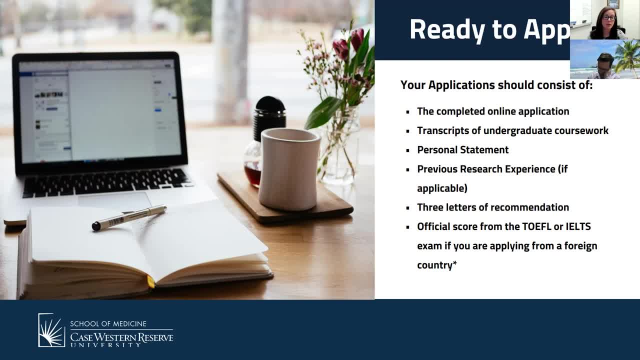 what you've done in the past academically, what your future goals are academically, what your future goals are academically, what your future goals are, if you've done any research, or what your, if you've done any research, or what your, if you've done any research, or what your interest is. 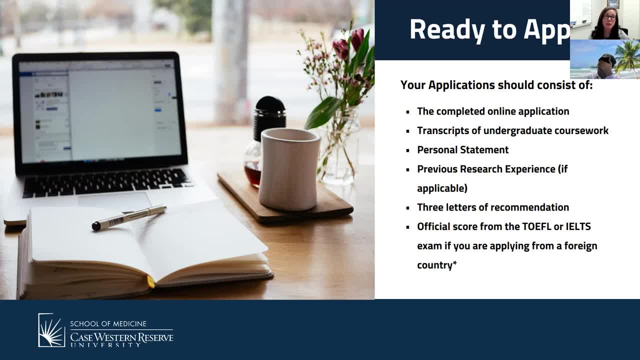 interest is. interest is just so we can get to know you and kind just so we can get to know you and kind just so we can get to know you and kind of understand your trajectory and your of understand your trajectory and your of understand your trajectory and your level of interest. 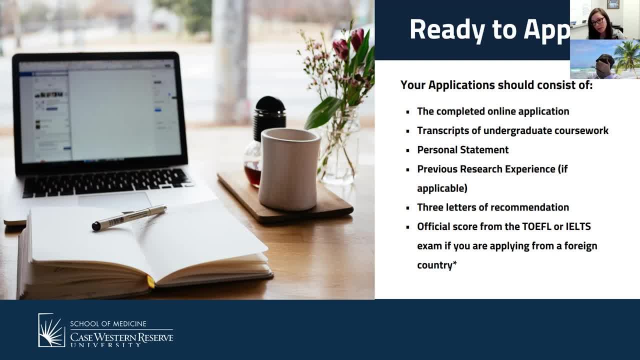 level of interest. level of interest if you have done any research. it is not if you have done any research. it is not if you have done any research. it is not a requirement that you have done, a requirement that you have done, a requirement that you have done research in the past as an undergraduate. 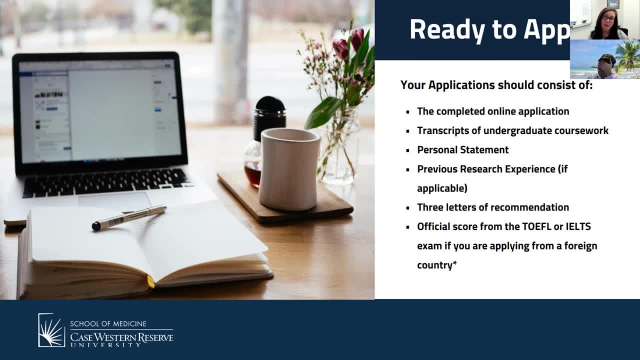 research in the past as an undergraduate. research in the past as an undergraduate. but if you have, we love to see you. but if you have, we love to see you. but if you have, we love to see you. submit that, submit that, submit that. we ask for three letters of. 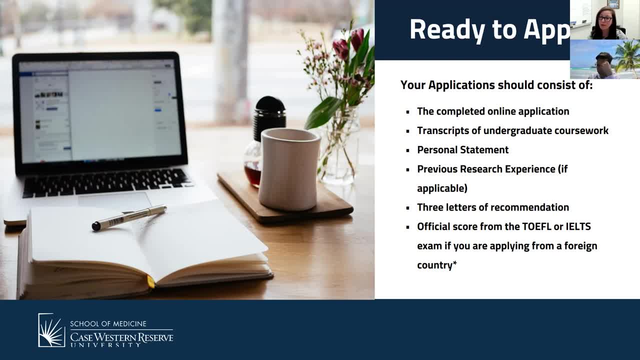 we ask for three letters of. we ask for three letters of recommendation from professional recommendation, from professional recommendation from professional sources. so no friends or family sources. so no friends or family sources, so no friends or family, and if possible, we'd like to see these. and if possible, we'd like to see these. 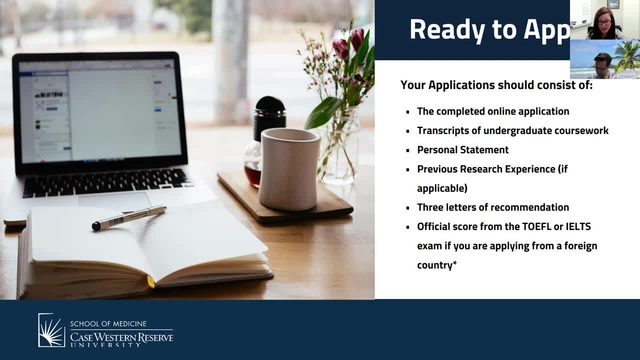 and, if possible, we'd like to see these come from a university, or have somebody come from a university, or have somebody come from a university, or have somebody put them on letterhead, put them on letterhead. put them on letterhead, just so if we can see where they're. 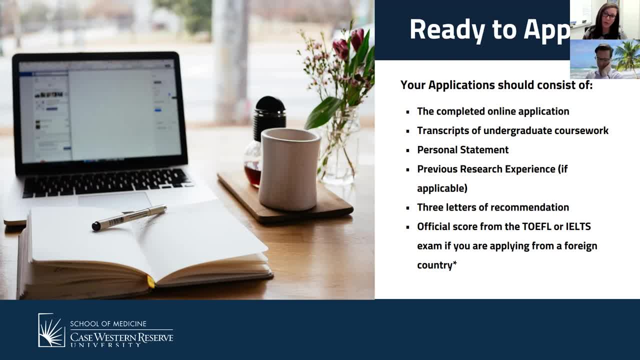 just so if we can see where they're, just so, if we can see where they're coming from, coming from, coming from, and then if you are an international, and then if you are an international, and then if you are an international student or have not previously studied, 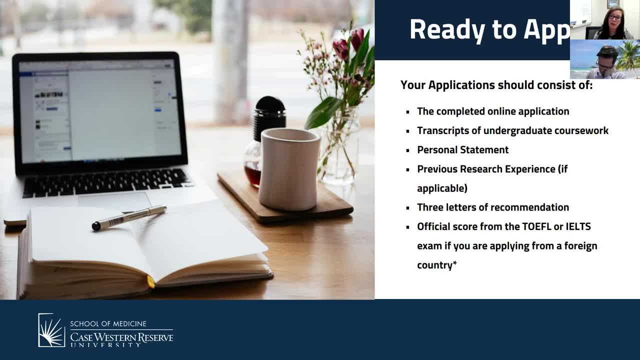 student or have not previously studied student or have not previously studied your undergraduate in english. we ask your undergraduate in english. we ask your undergraduate in english. we ask that you submit a toefl or ielts there. that you submit a toefl or ielts there. 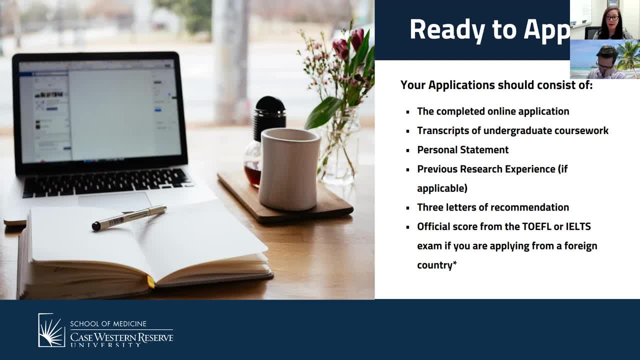 that you submit a toefl or ielts. there are a few other types of. are a few other types of. are a few other types of exams that we will accept. however i exams that we will accept. however, i exams that we will accept. however, i frequently get asked if we accept dual. 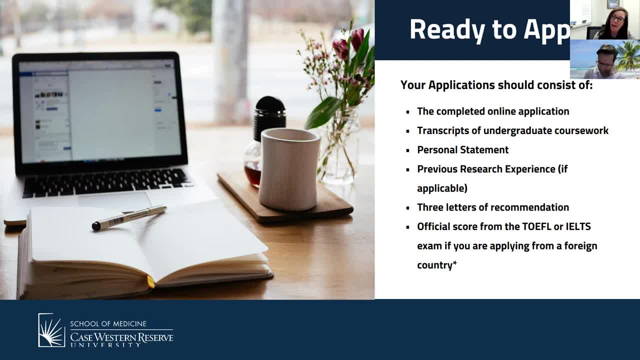 frequently get asked if we accept dual, frequently get asked if we accept dual lingo and that lingo and that lingo, and that is a no um is a no um is a no um. so then let's talk about deadlines. so then let's talk about deadlines. 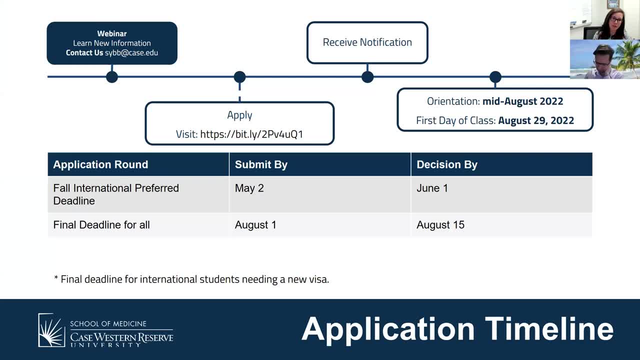 so then let's talk about deadlines. uh for our application. we did kind of uh for our application. we did kind of uh for our application. we did kind of just to incentivize people. we have a just to incentivize people. we have a just to incentivize people. we have a fall international preferred deadline. i. 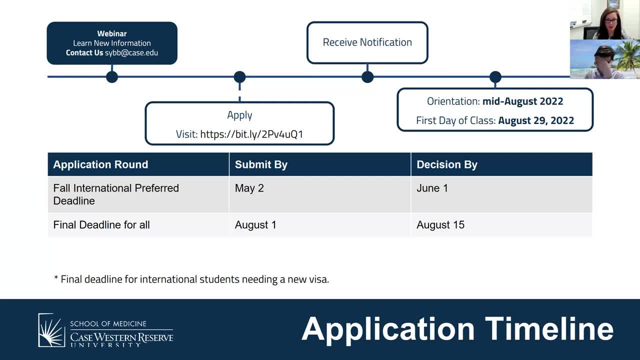 fall international preferred deadline. i fall international preferred deadline. i don't want to say don't, want to say don't want to say it's a final deadline, because of course it's a final deadline, because of course it's a final deadline, because of course we'll accept your application after that. 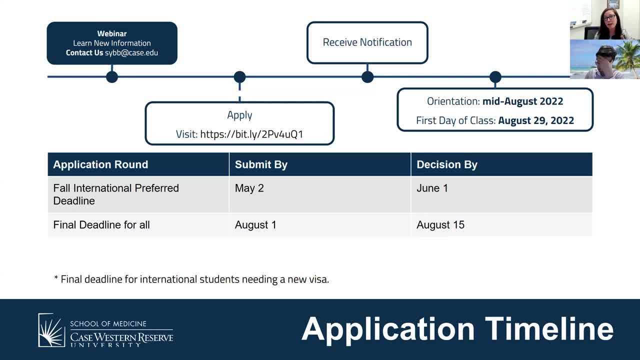 we'll accept your application after that. we'll accept your application after that. but we like to see all of our but we like to see all of our, but we like to see all of our international students apply by may 2nd. international students: apply by may 2nd. 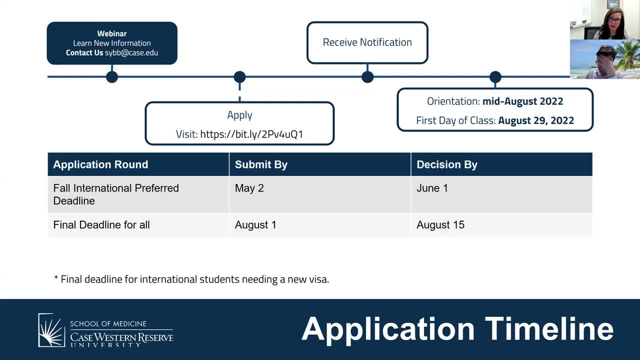 international students. apply by may 2nd for you, so that you have time to for you, so that you have time to for you, so that you have time to go through the visa application process. go through the visa application process. go through the visa application process. find housing and not be rushed. 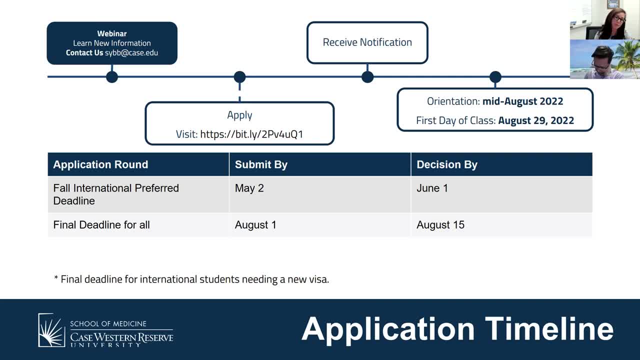 find housing and not be rushed. find housing and not be rushed. so that's just to help set you up for so, that's just to help set you up for. so that's just to help set you up for success in being enrolled, success in being enrolled, success in being enrolled, our final deadline for everybody. 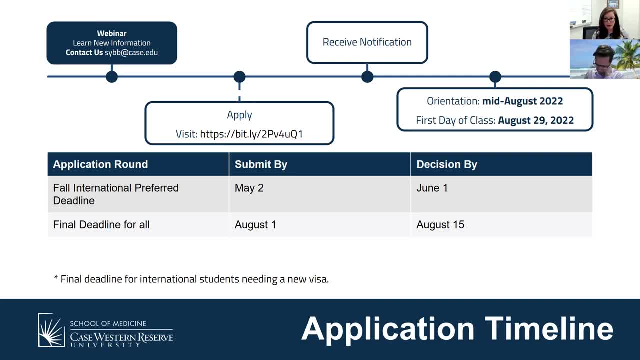 our final deadline for everybody. our final deadline for everybody, whether they are domestic or whether they are domestic or whether they are domestic or international, is august 1st. international is august 1st. international is august 1st. again. this does not leave you a lot of. again, this does not leave you a lot of again, this does not leave you a lot of time. if you're an international student time, if you're an international student time, if you're an international student, if you don't already have a visa and you, if you don't already have a visa, and you. 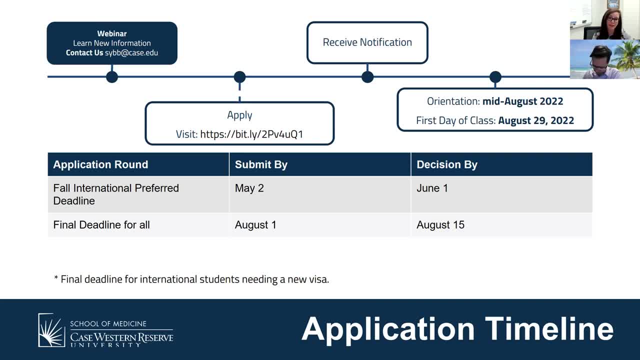 if you don't already have a visa and you need to go through that process, i would need to go through that process. i would need to go through that process. i would not recommend waiting until that long. to not recommend waiting until that long. to not recommend waiting until that long to apply. 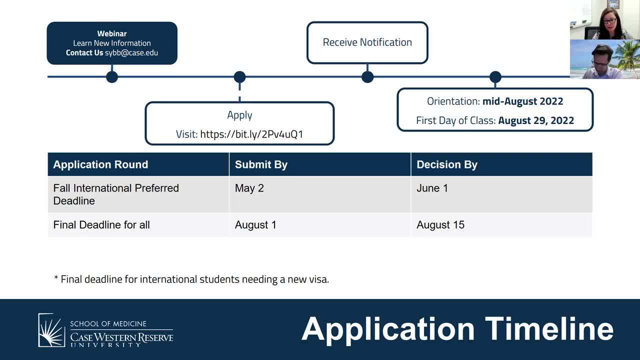 apply, apply, but you have up until that date. and dr, but you have up until that date. and dr, but you have up until that date. and dr. lodowski and the panel who reviews lodowski and the panel who reviews lodowski and the panel who reviews applications are very quick to turn. 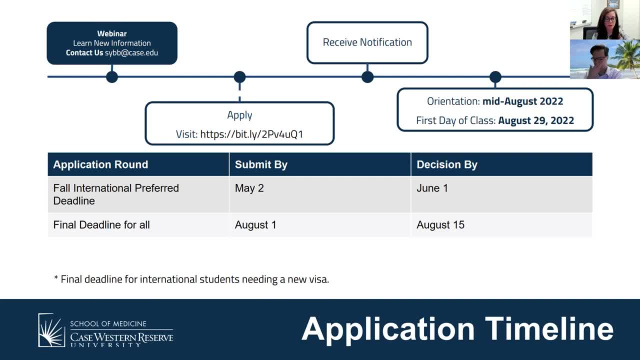 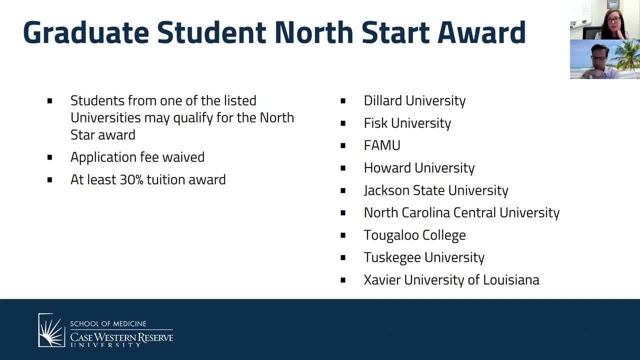 applications are very quick to turn. applications are very quick to turn around your application. they try to around your application. they try to around your application. they try to if you have studied your undergraduate, if you have studied your undergraduate, if you have studied your undergraduate at any of these. 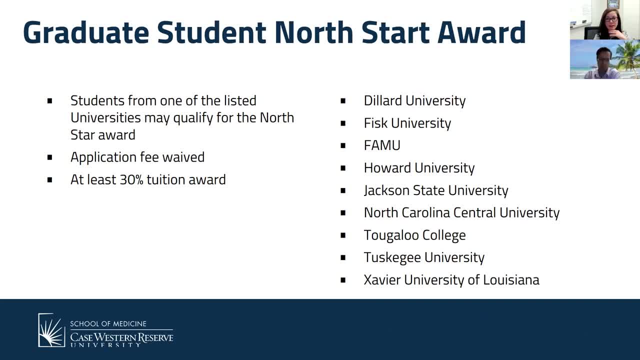 at any of these, at any of these places, the universities that are listed places, the universities that are listed places, the universities that are listed here on the right hand side, here on the right hand side, here on the right hand side- um, you, um, you, um. you do qualify for this. you don't need to do. 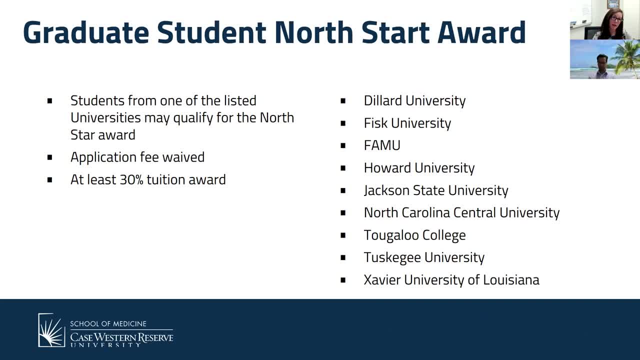 do qualify for this. you don't need to do do qualify for this. you don't need to do anything additional for this. and what anything additional for this? and what anything additional for this? and what that means is you automatically have that means. is you automatically have that means, is you automatically have your application fee waived, and 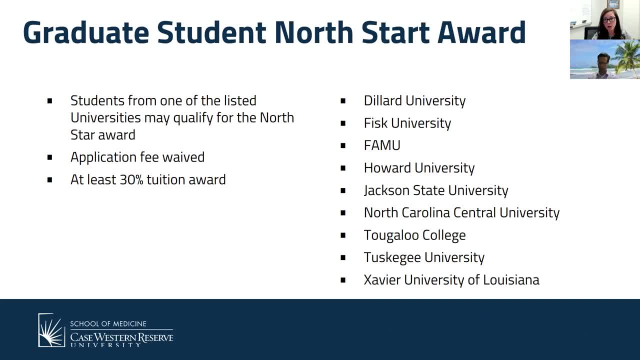 your application fee waived and your application fee waived and additionally, you receive at least 30 additionally. you receive at least 30. additionally, you receive at least 30 tuition awards, so you get 30 off your tuition awards. so you get 30 off your tuition awards. so you get 30 off your tuition. 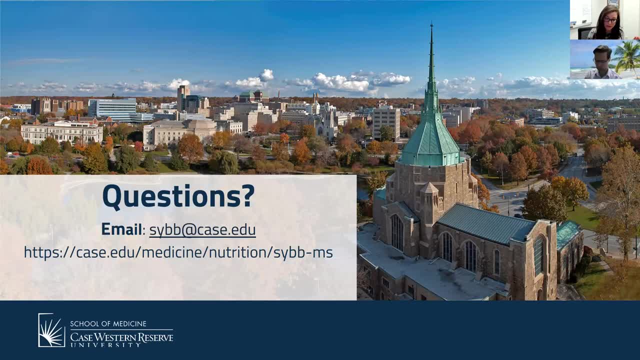 so pretty simple is now. i have a couple. so pretty simple is now i have a couple. so pretty simple is now i have a couple of pre-submitted questions for you, dr, of pre-submitted questions for you, dr, of pre-submitted questions for you, dr lodowski, and then we will open it up if 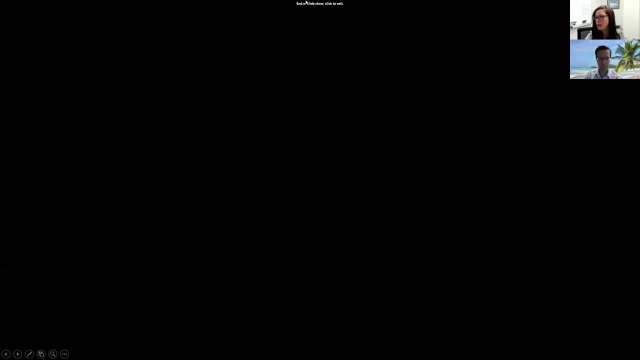 lodowski, and then we will open it up. if lodowski, and then we will open it up. if anybody has a question, please feel free. anybody has a question. please feel free. anybody has a question, please feel free to to to drop it in the chat. drop it in the chat. 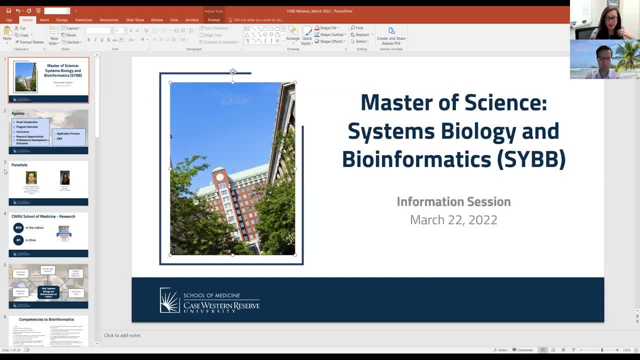 drop it in the chat. um. the first question is um. the first question is um. the first question is if you could go on a little more about. if you could go on a little more about if you could go on a little more about different career opportunities. that 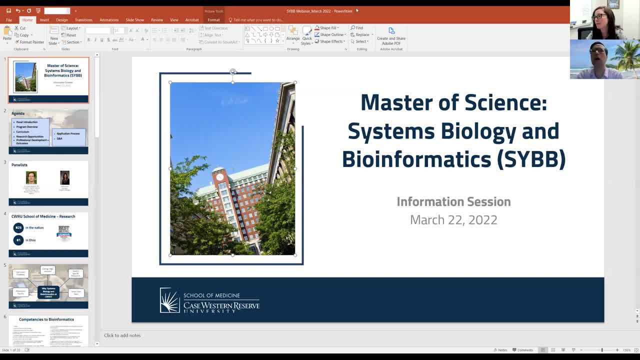 different career opportunities, that different career opportunities that you've seen. sure um, let's see, so we've had. sure um, let's see, so we've had. sure um, let's see, so we've had. i, we've graduated, so we're a relatively. i we've graduated, so we're a relatively. 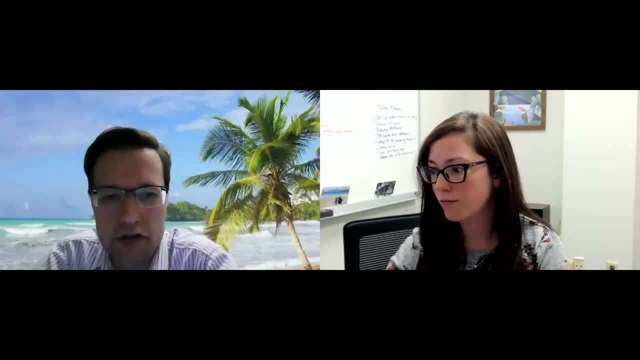 i, we've graduated, so we're a relatively new program. we've been around for about new program. we've been around for about new program. we've been around for about eight years now. um so we've. i think we've eight years now. um so we've, i think we've. 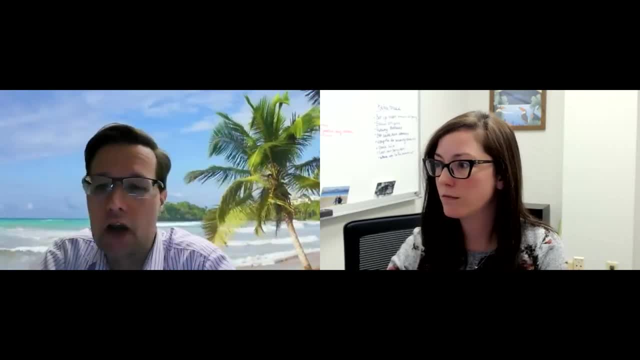 eight years now, um, so we've, i think we've- graduated in the neighborhood of graduated in the neighborhood of graduated in the neighborhood of about 30 master students, about 30 master students, about 30 master students. um, and you know, um, and you know um, and you know. they've done all kinds of different things. 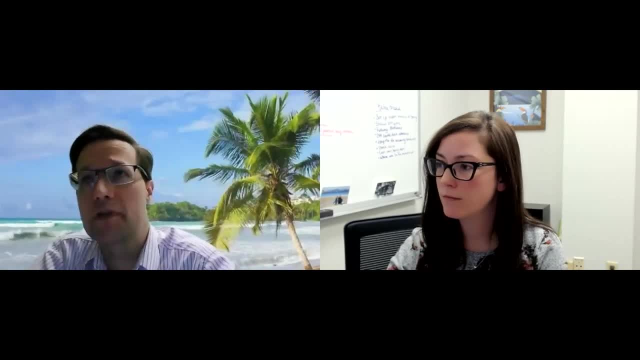 they've done all kinds of different things. they've done all kinds of different things: um clinical research coordinator at um clinical research coordinator at um clinical research coordinator at a hospital, a hospital, a hospital. um i've had five or six of the sybb. um i've had five or six of the sybb. 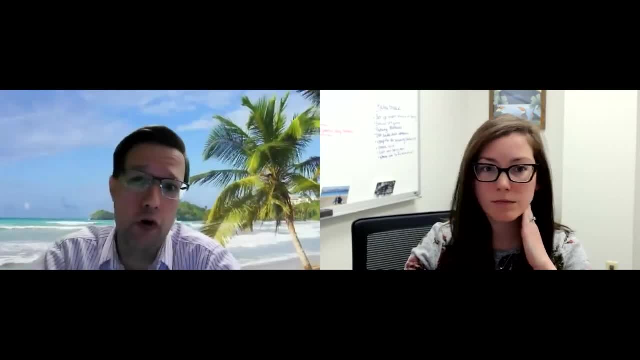 um, i've had five or six of the sybb students go on directly to phd students, go on directly to phd students, go on directly to phd? um, two of them, two um. two of them. two, um two. no, three of them actually stuck around. 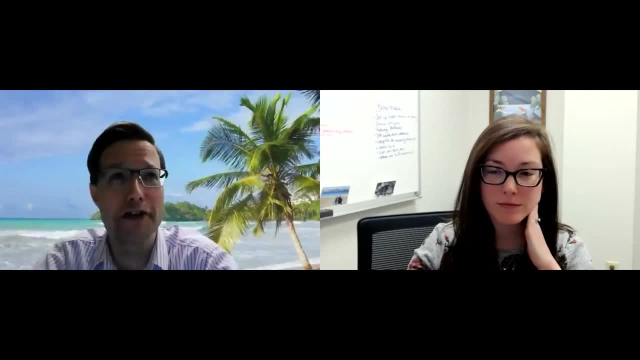 no three of them actually stuck around. no three of them actually stuck around: here and got a phd, or here and got a phd, or here and got a phd, or in the process of getting a phd at case. in the process of getting a phd at case. 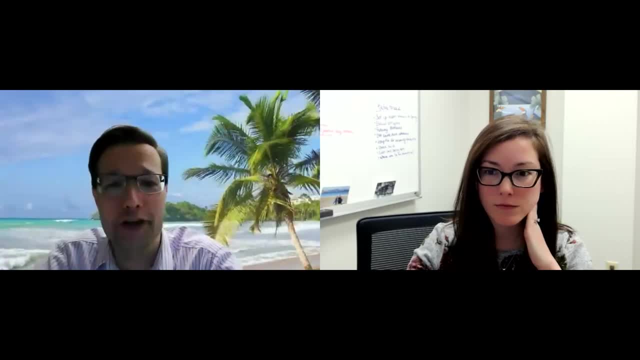 in the process of getting a phd at case um, one of which actually left and went um, one of which actually left and went um. one of which actually left and went into industry for a year. decided he into industry for a year. decided he into industry for a year. decided he hated it, wanted to go back to. 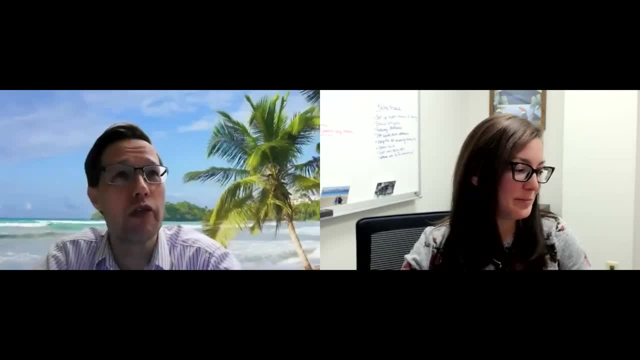 hated it wanted to go back to. hated it wanted to go back to go go back to academia. um, we have a guy: go go back to academia. um, we have a guy go go back to academia. um, we have a guy that. that's that that. um went to go work. 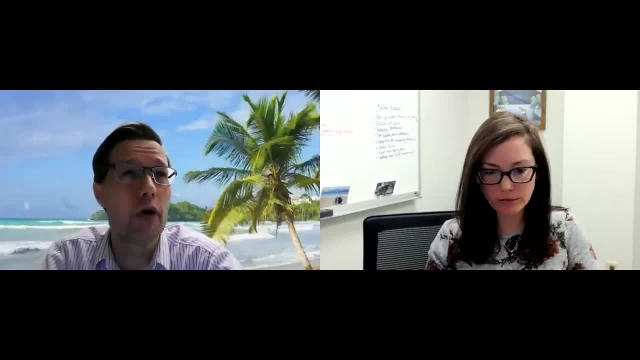 that that that um went to go work, that that that um went to go work for cisco, for cisco, for cisco. um another one works for ibm. both of um. another one works for ibm. both of um. another one works for ibm. both of those guys, actually, while they were. 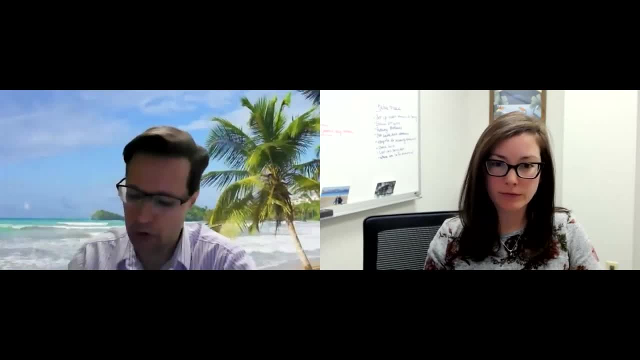 those guys actually, while they were, those guys actually, while they were trained in biological data analysis, trained in biological data analysis, trained in biological data analysis, actually do, actually do, actually do non-biological data analysis at this, non-biological data analysis, at this non-biological data analysis at this point. 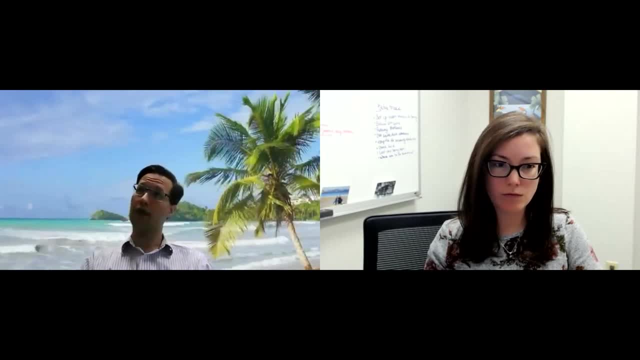 point, point um, there's quite a few of the master's. um, there's quite a few of the master's um, there's quite a few of the master's students, students, students that end up in medical school. um, that end up in medical school. um, that end up in medical school. um, let's see, i'm trying to go through all. 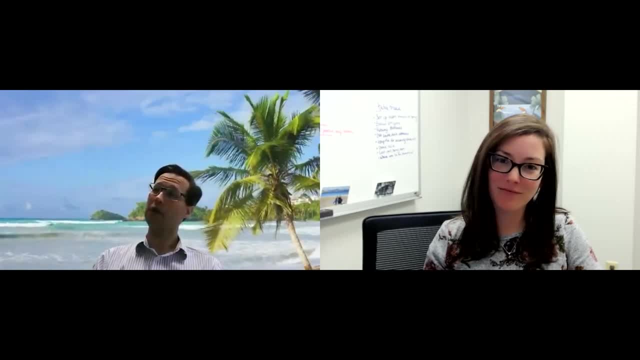 let's see, i'm trying to go through all. let's see, i'm trying to go through all these people in my head, these people in my head, these people in my head, um, anybody else that i that pretty much. um, anybody else that i that pretty much. 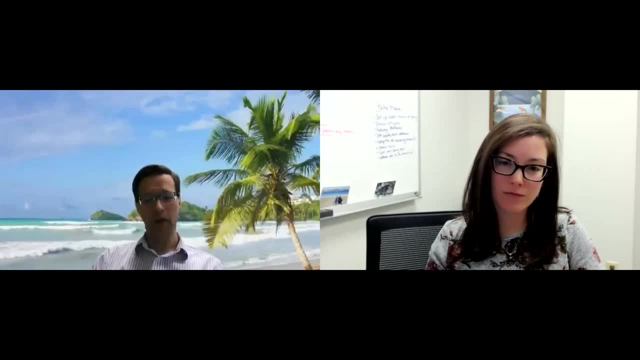 um anybody else that i, that pretty much covers everybody. everybody. that um covers everybody, everybody. everybody that um covers everybody. everybody, everybody that um, um, that i can think of off the top of um, that i can think of off the top of um, that i can think of off the top of my head, okay, so 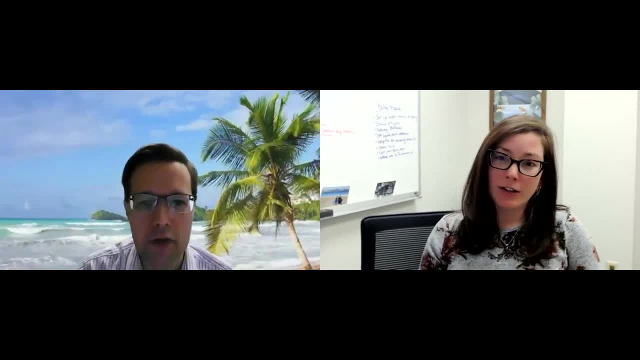 my head okay. so my head okay. so someone sent it sent a question, okay. so someone sent it sent a question, okay. so someone sent it sent a question, okay. so i'm short on one letter of. i'm short on one letter of. i'm short on one letter of recommendation, now okay. 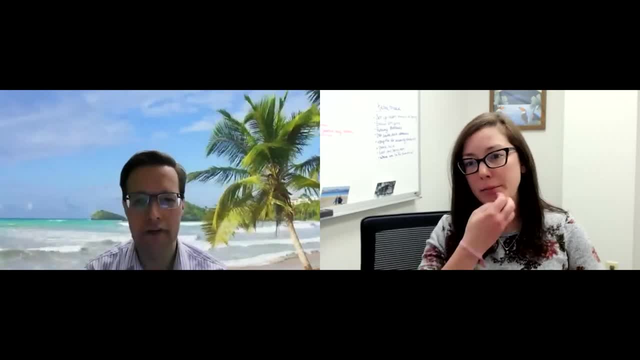 recommendation now okay. recommendation now okay. so, so, so, so i can actually answer that. um so, if so, i can actually answer that. um so, if so, i can actually answer that. um so, if you're short on one letter of you're short on one letter of you're short on one letter of recommendation, you really can't get a. 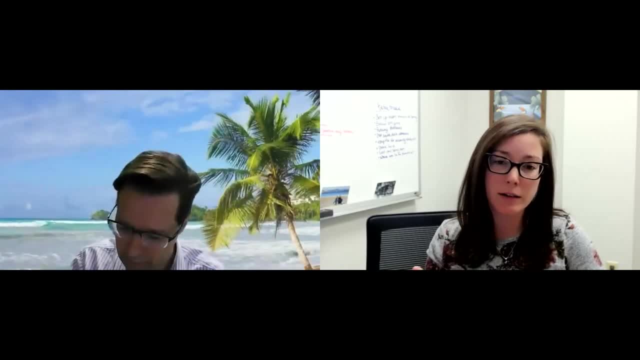 recommendation. you really can't get a recommendation. you really can't get a hold of it. that that's up to dr hold of it. that that's up to dr. hold of it. that that's up to dr lodowski. if lodowski, if lodowski, if a lot of times he will review those for. 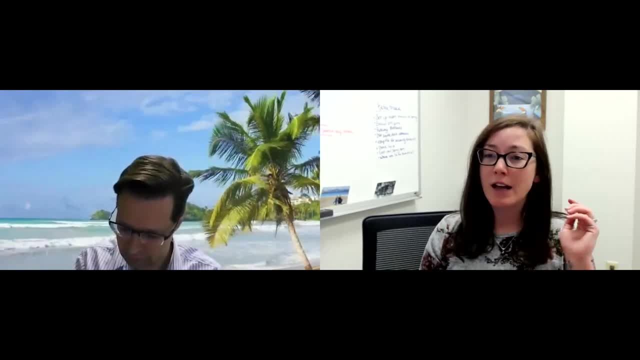 a lot of times. he will review those for a lot of times. he will review those for you, um. but if you're having trouble, you, um. but if you're having trouble, you, um. but if you're having trouble getting them with the system, getting them with the system. 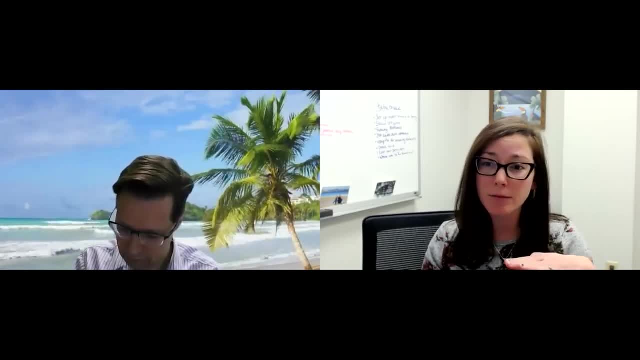 getting them with the system. and it's not. it's. it's showing me that and it's not. it's it's showing me that and it's not. it's: it's showing me that you have no letters of recommendation. you have no letters of recommendation. you have no letters of recommendation. that's probably why your application is. 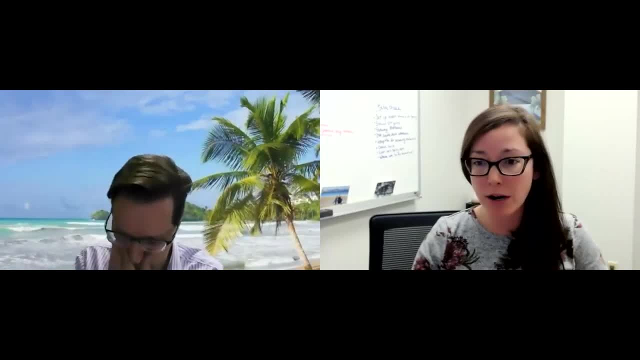 that's probably why your application is. that's probably why your application is not being pulled for any reason. just not being pulled for any reason, just not being pulled for any reason. just email those to email those, to email those to sybb at caseedu. sybb at caseedu. 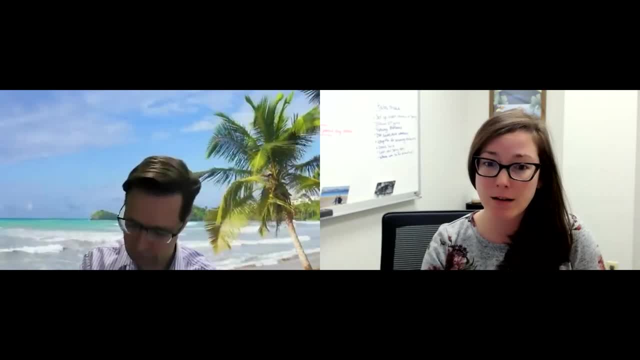 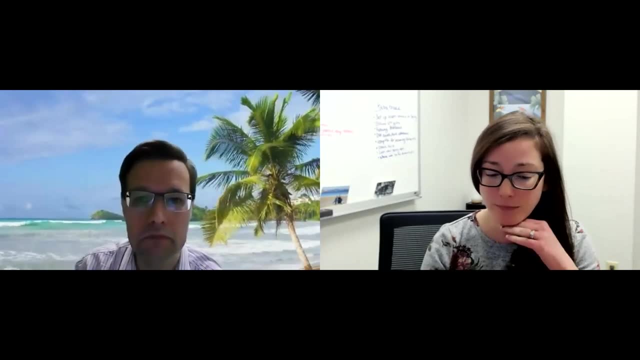 sybb at caseedu and i'll get those uploaded to your and i'll get those uploaded to your and i'll get those uploaded to your system. so another question we had is. so another question we had is. so another question we had is: a student has a bachelor's in chemistry. 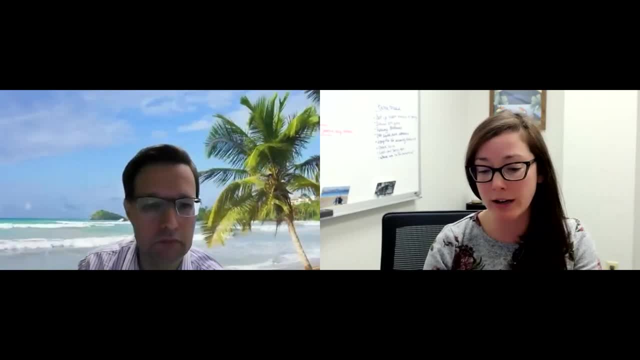 a student has a bachelor's in chemistry. a student has a bachelor's in chemistry and they want to know if you will still and they want to know if you will still and they want to know if you will still accept them, even though they've only had. 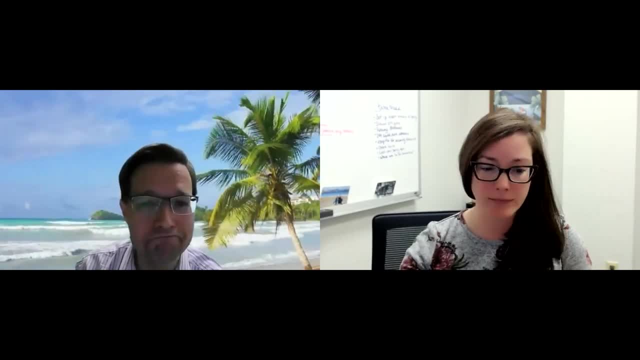 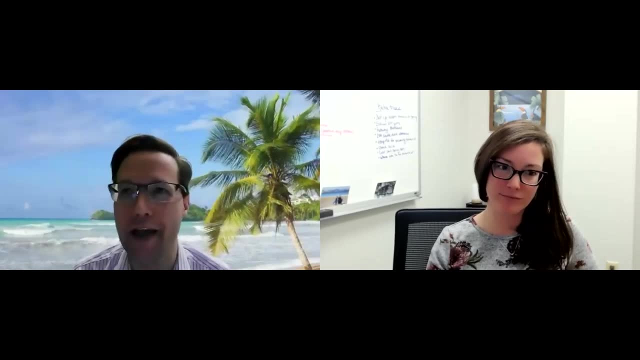 accept them, even though they've only had, accept them, even though they've only had biology one biology, one, biology one. yes, yes, no, i i mean you there, yes, no, i i mean you there, yes, no, i i mean you there, i really, we, we were, look, i i mean yeah. 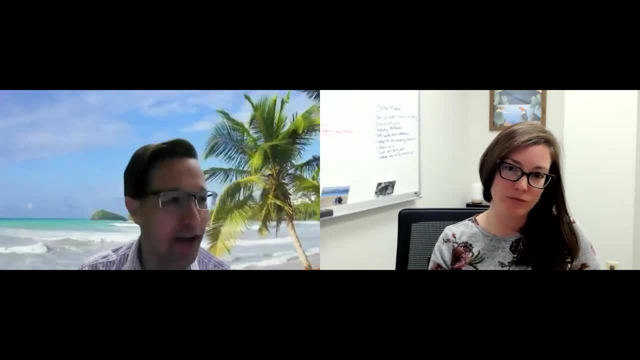 i really we, we were look. i i mean, yeah, i really we, we were look. i i mean, yeah, you're you're going to need to apply and you're you're going to need to apply and you're you're going to need to apply and and we'll look at your application. but 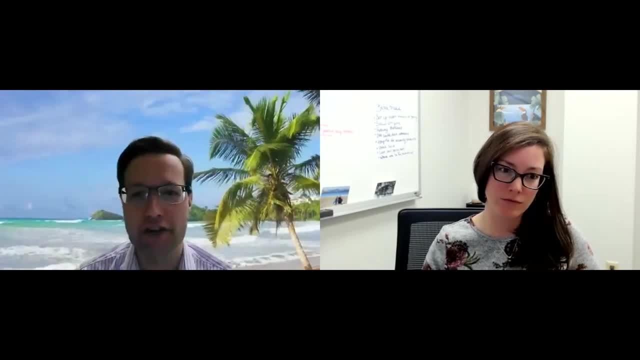 and we'll look at your application, but and we'll look at your application, but we don't, we don't um, we don't, we don't, we don't um, we don't, we don't, we don't um. we don't necessarily assume that because you 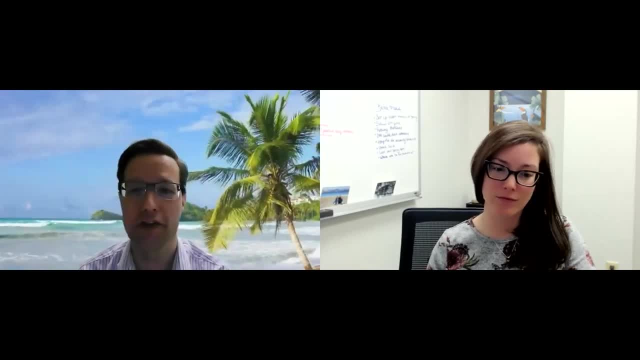 necessarily assume that, because you necessarily assume that because you only had a, only had a, only had a, you know one class in biology that you, you know one class in biology that you, you know one class in biology that you have, and the truth is is that there are. have, and the truth is is that there are have, and the truth is is that there are quite. we have people that come in with quite. we have people that come in with quite. we have people that come in with computer science degrees too, and they computer science degrees too, and they. 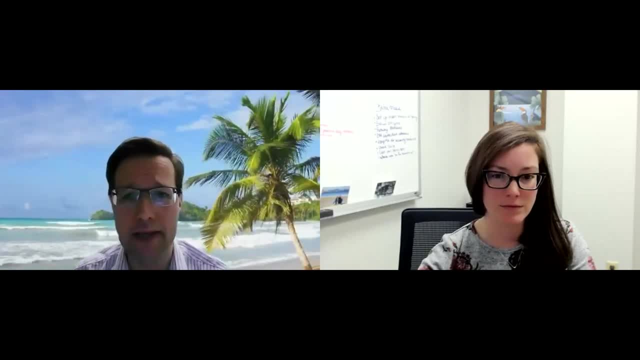 computer science degrees too, and they don't have any bio biology. so you don't have any bio biology, so you don't have any bio biology. so you wouldn't be in any real, wouldn't be in any real, wouldn't be in any real. and i think you know, having the 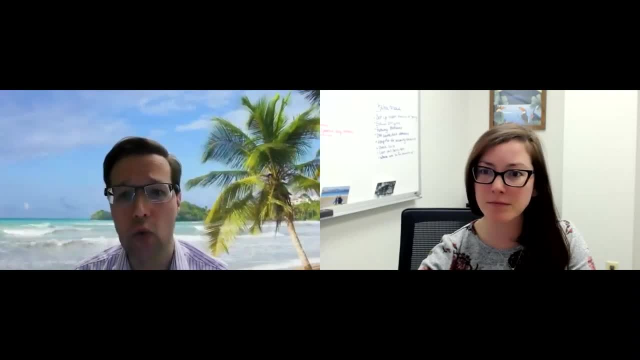 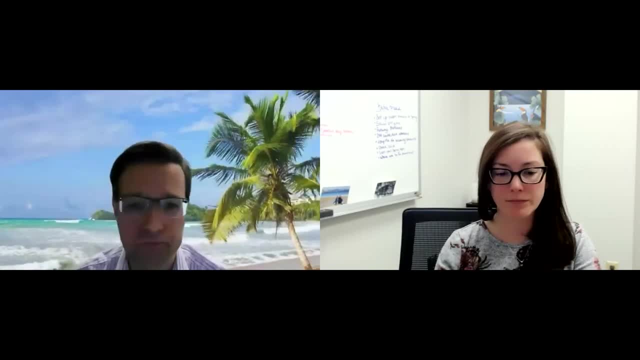 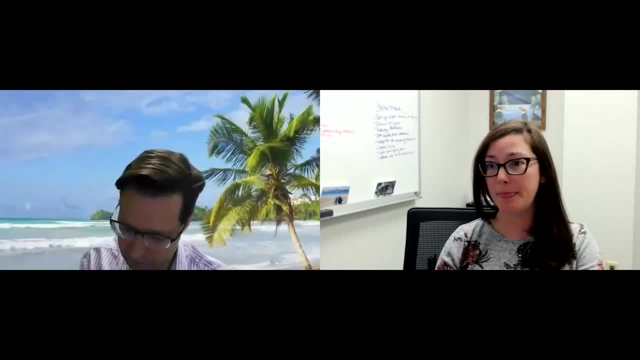 scholarship opportunities we do have in. scholarship opportunities we do have in the department. it's a very small pocket, the department. it's a very small pocket, the department. it's a very small pocket of funding, of funding, of funding, um, it's only five thousand dollars and um, it's only five thousand dollars. and 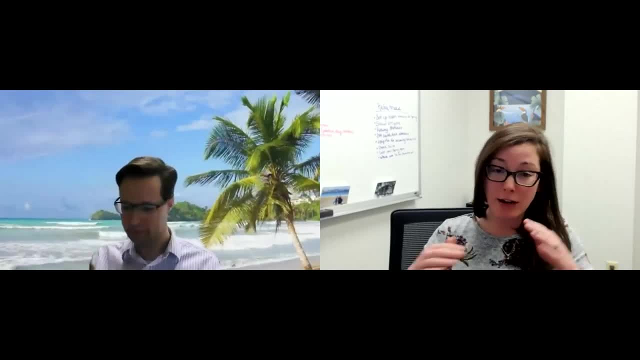 um, it's only five thousand dollars and it only goes to a couple of students, so it only goes to a couple of students, so it only goes to a couple of students. so, if, if, if, and it will know what, like obviously, and it will know what, like obviously. 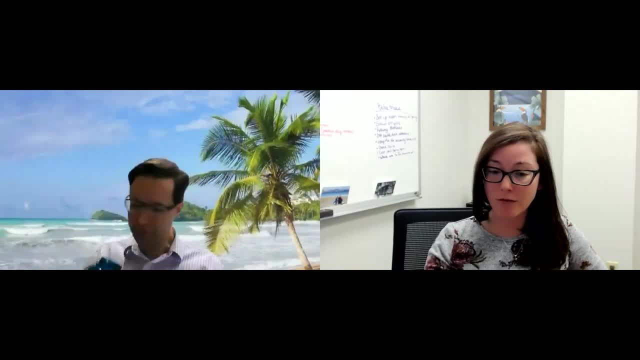 and it will know what. like: obviously, that is not going to cover the cost of that, is not going to cover the cost of that, is not going to cover the cost of tuition. we talked about the cost of tuition. we talked about the cost of tuition. we talked about the cost of tuition and, unfortunately, one of my most. 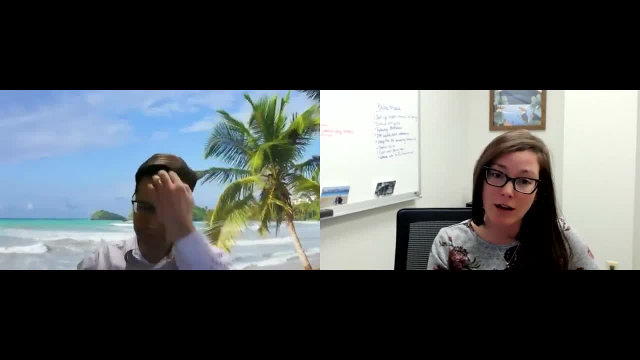 tuition and unfortunately one of my most tuition and unfortunately one of my most frequently asked questions is about. frequently asked questions is about. frequently asked questions is about graduate assistantships, graduate assistantships, graduate assistantships, and in our department we do not have and in our department we do not have. 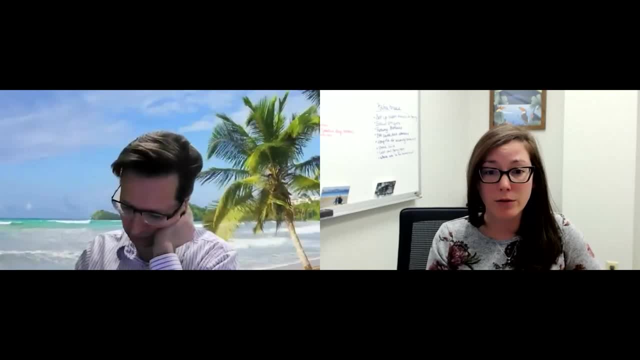 and in our department we do not have those. a lot of our students have to find those. a lot of our students have to find those. a lot of our students have to find private funding or loans for their private funding or loans for their private funding or loans for their studies. 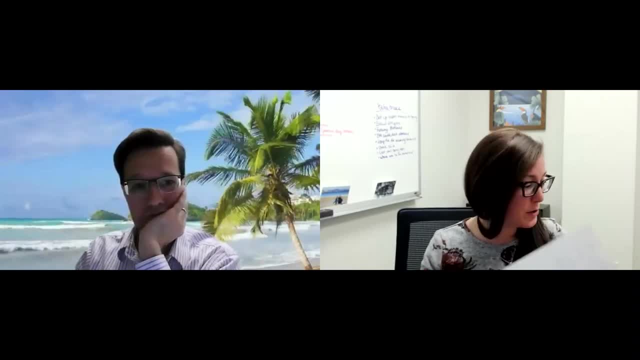 that's always the sad part. i get a lot. that's always the sad part. i get a lot of questions about funding and i wish i of questions about funding and i wish i of questions about funding and i wish i could do more for students but could do more for students. but 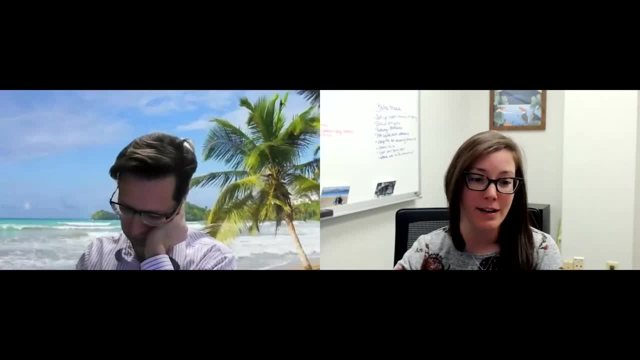 could do more for students. but that's where we are. that's where we are. that's where we are. does anyone else have any additional? does anyone else have any additional? does anyone else have any additional questions? i also just to kind of elaborate a little. i also just to kind of elaborate a little. 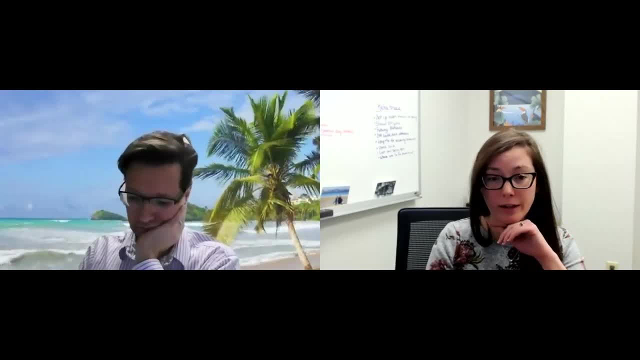 i also just to kind of elaborate a little bit. i get asked a lot of questions on bit. i get asked a lot of questions on bit. i get asked a lot of questions on cleveland in general, um cleveland is, cleveland in general, um cleveland is. 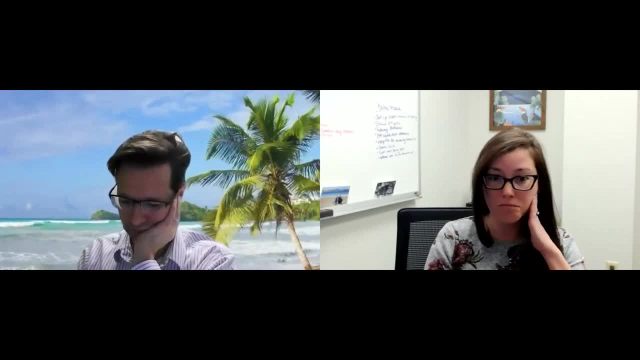 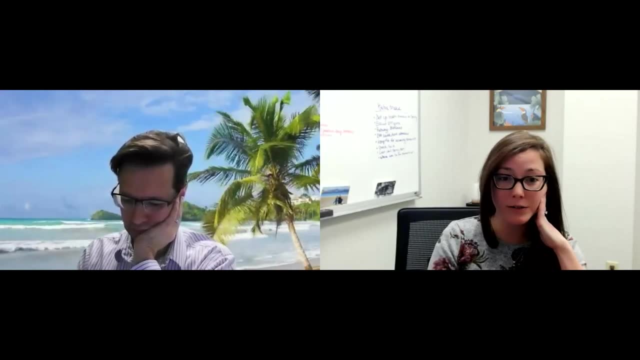 cleveland in general, um, cleveland is very affordable. the cost of living here very affordable. the cost of living here very affordable. the cost of living here is is is housing around campus, several of which housing around campus, several of which housing around campus, several of which are walkable to campus. 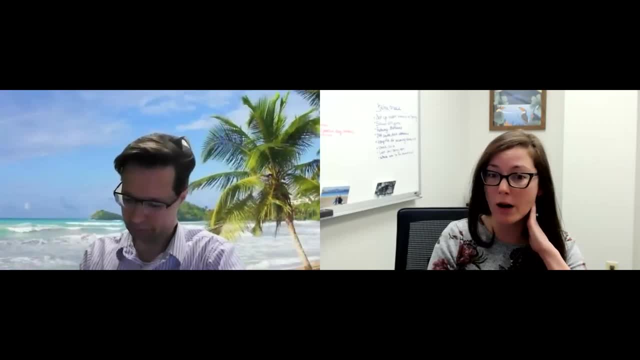 are walkable to campus are walkable to campus. um, we do have a bus system that runs. um. we do have a bus system that runs. um. we do have a bus system that runs right down the main street, that we're right down the main street, that we're. 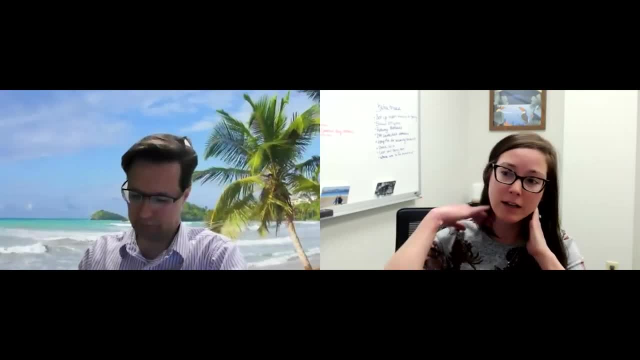 right down the main street that we're located off of, as well as a rapid located off of, as well as a rapid located off of, as well as a rapid station, rapid train that can kind of station rapid train, that can kind of station rapid train that can kind of allow you to go from one side of 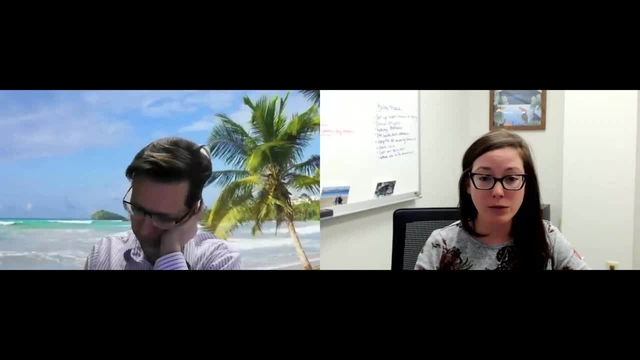 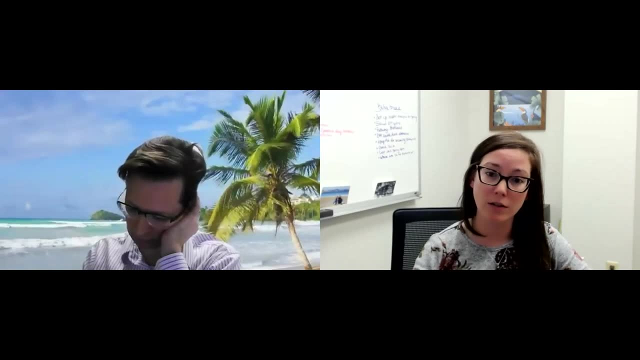 allow you to go from one side of, allow you to go from one side of cleveland to the other, and you do have cleveland to the other and you do have cleveland to the other, and you do have discounts for several different, discounts for several different. 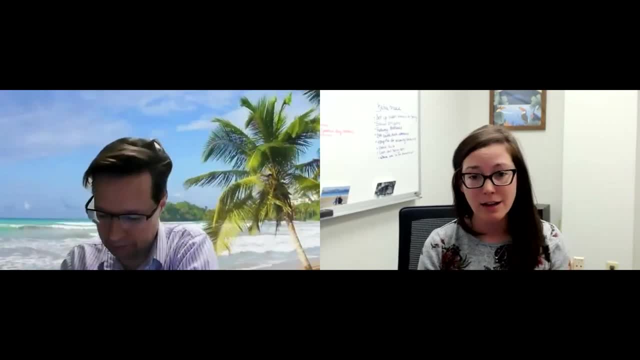 discounts for several different that are free to you as well. so there's that are free to you as well. so there's that are free to you as well. so there's plenty. it's a very diverse city, plenty. it's a very diverse city, plenty. it's a very diverse city and there is always plenty to do here. 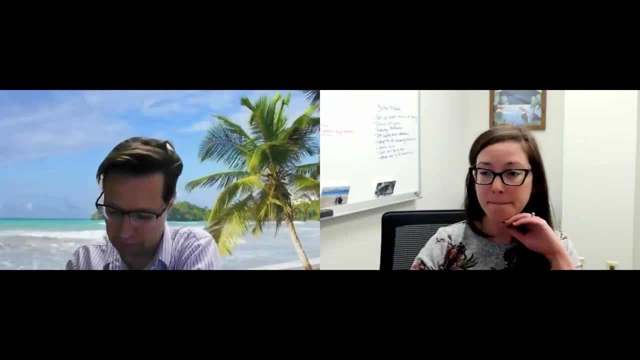 and there is always plenty to do here, and there is always plenty to do here at an affordable cost. so i think that's about it if people so. i think that's about it if people so. i think that's about it if people think of questions after the fact. 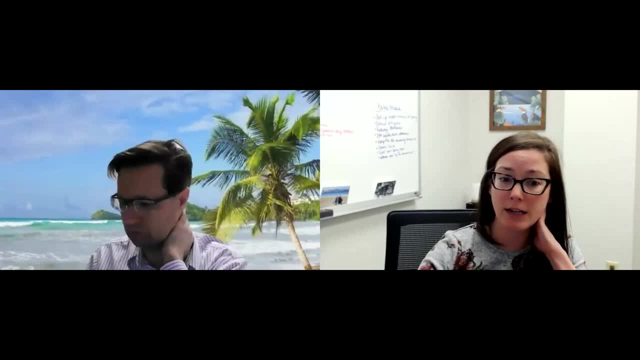 think of questions after the fact. think of questions after the fact. please feel free to email sybb at caseedu. please feel free to email sybb at caseedu. please feel free to email sybb at caseedu and either myself or dr lodowski can, and either myself or dr lodowski can. 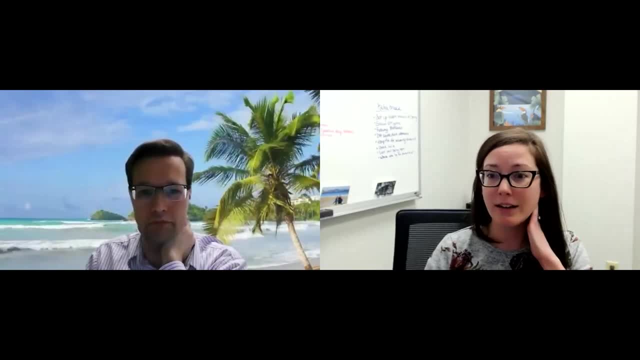 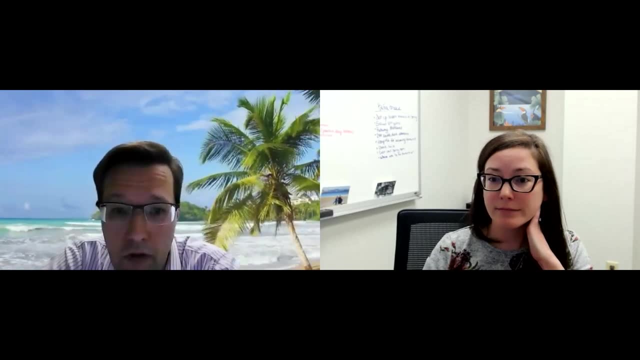 and either myself or dr lodowski can answer any questions that you might answer, any questions that you might answer, any questions that you might think of. well, i think we already kind of answered well, i think we already kind of answered. well, i think we already kind of answered that. so 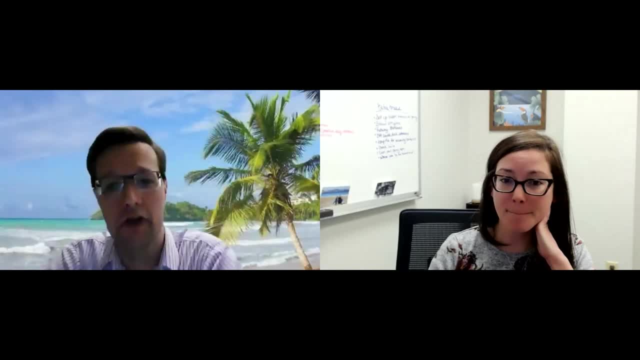 that, so that. so there's, there's only a small amount of there's, there's only a small amount of there's, there's only a small amount of aid at the master's level, aid at the master's level, aid at the master's level. um, now, to me it sounds, if you're, if, 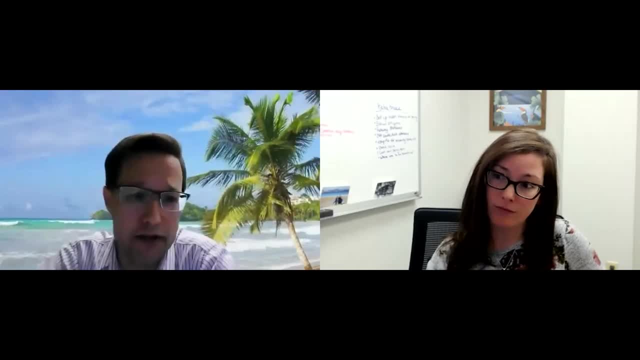 um. now to me it sounds if you're, if um. now to me it sounds if you're, if you really are that you really are, that, you really are that well published, you might consider well published. you might consider well published. you might consider applying to the phd program next year. 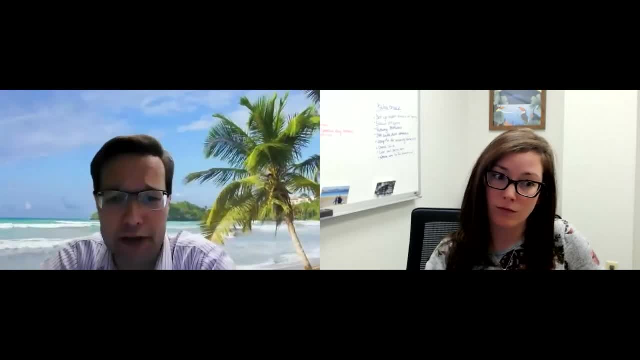 applying to the phd program next year. applying to the phd program next year. i mean that that's the only, that's the. i mean that that's the only, that's the. i mean that that's the only. that's the only way that you can make it free. 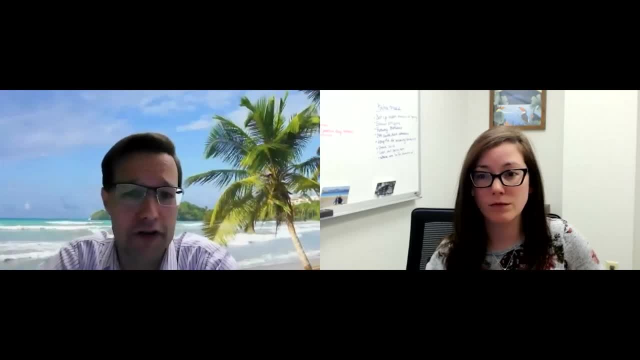 only way that you can make it free, only way that you can make it free, is that, if you, if you sign on for the, is that, if you, if you sign on for the, is that, if you, if you sign on for the phd right, there's a 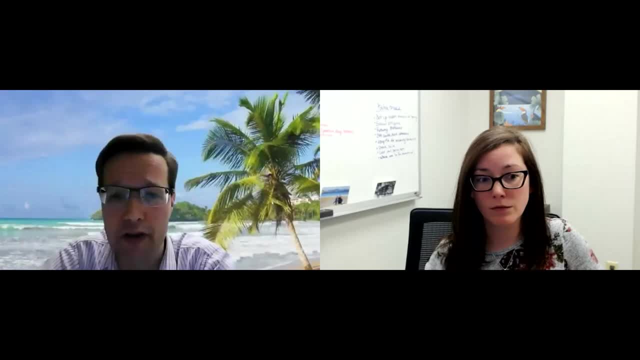 phd right. there's a phd right, there's a that that does not have tuition, that that does not have tuition, that that does not have tuition associated with it. uh, however, it is associated with it. uh, however, it is associated with it. uh, however, it is quite. 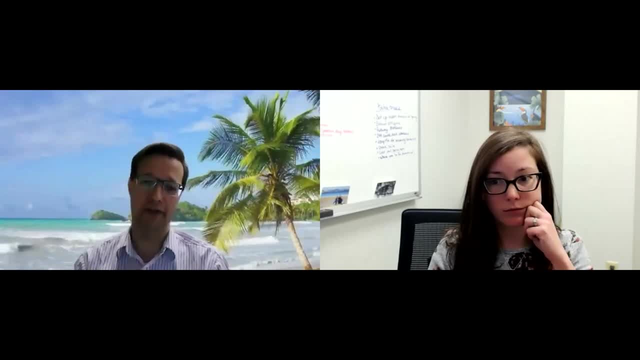 quite, quite um competitive, so anyway. so that's the? um competitive, so anyway. so that's the? um competitive, so anyway. so that's the. that's all i can say really. that's all i can say, really. that's all i can say really, and that and that. 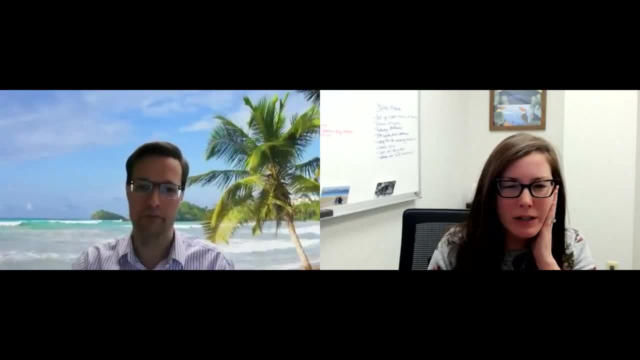 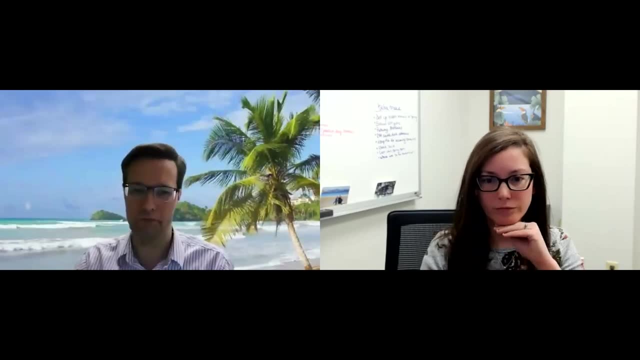 and that that application cycle has closed out, for that application cycle has closed out, for that application cycle has closed out for this year and it will reopen in this year. and it will reopen in this year and it will reopen in november, november, november, yeah, yeah, yeah, beginning of november, yes, 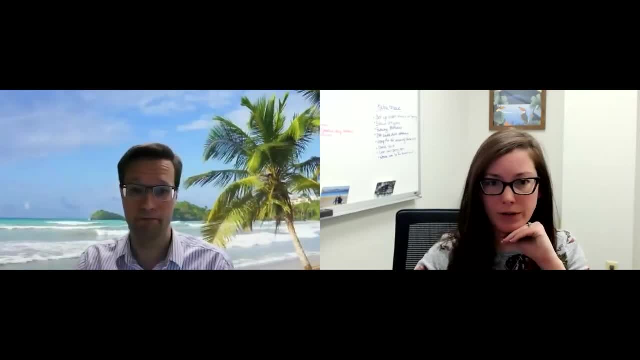 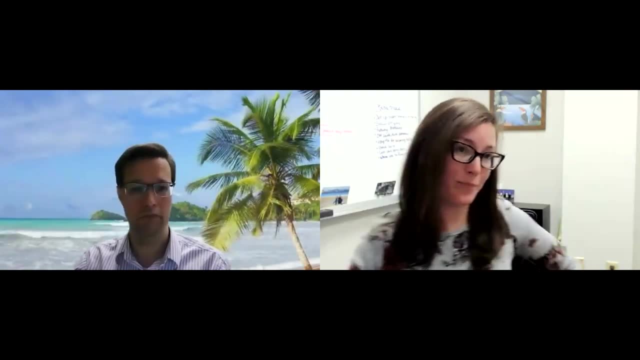 okay, well, thank you for your time and again. any additional questions can, and again, any additional questions can, and again, any additional questions can go to sybb caseedu. go to sybb caseedu. go to sybb caseedu. thank you, thank you, thank you.